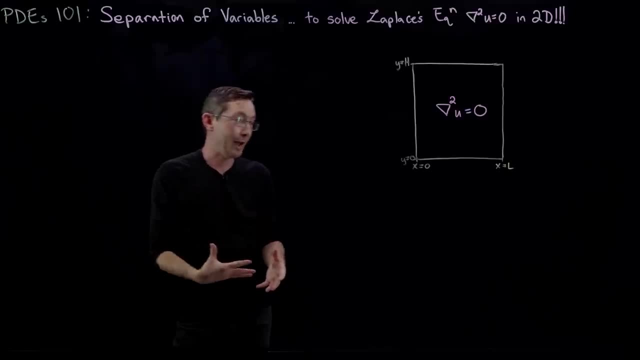 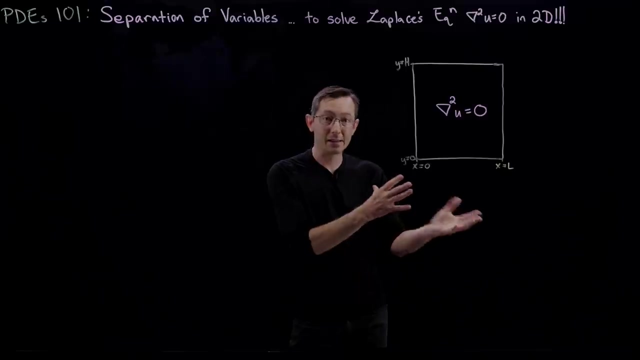 talk about some of the most important concepts in in engineering math, For example, we're going to show that when we take our separation of variables and we get our system of ordinary differential equations, we will essentially derive that the Fourier transform sines and cosines, a basis of 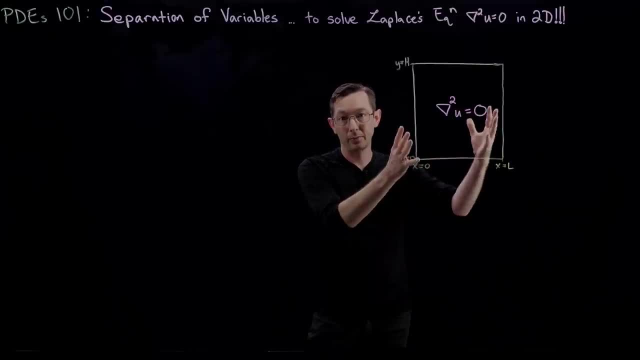 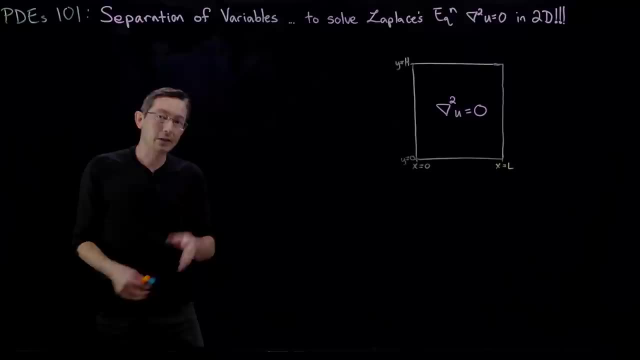 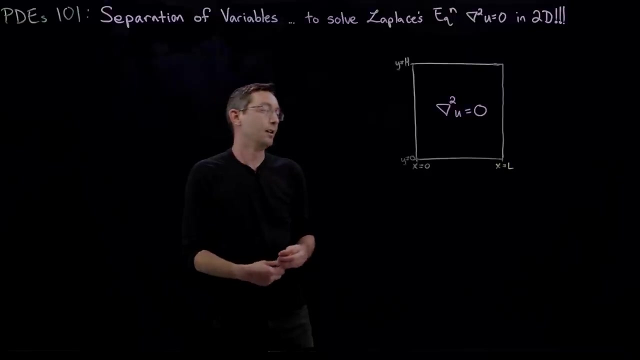 sines and cosines are the eigenfunctions of Laplace's equation on this domain. So really important connections and I'm super excited to walk you through this. Believe it or not, this is a weekend. I'm back in Seattle since our year-long sabbatical at Caltech and I couldn't wait. I've 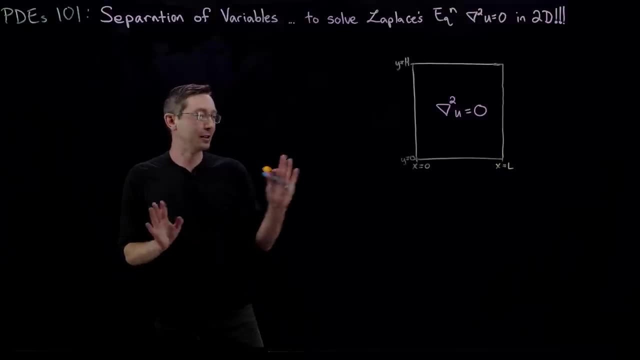 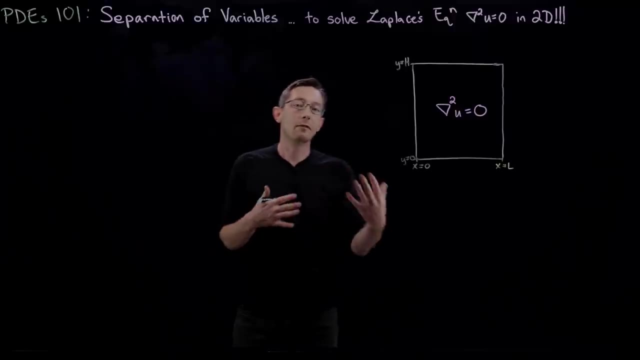 been planning a whole set of videos for a while, so I decided to come in and film this up. All right, and whenever you solve a partial differential equation, of course you need some combination of initial conditions and boundary conditions, depending on if it's a PDE in space or in time. 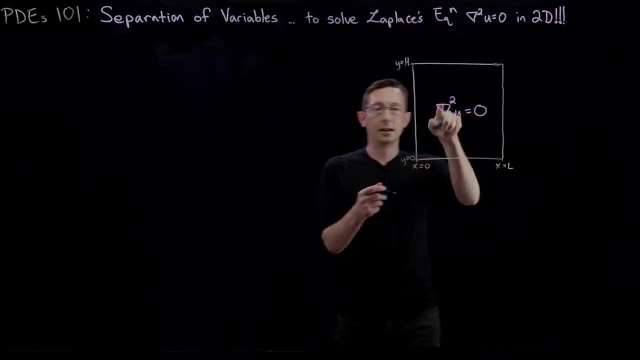 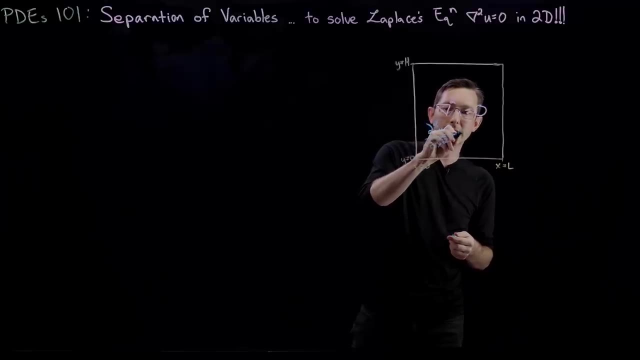 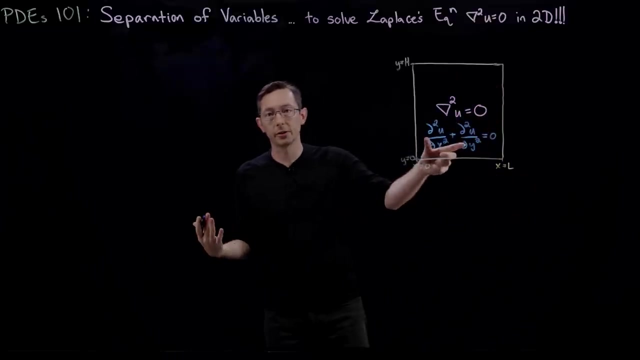 For this Laplace's equation- and remember Laplace's equation- u is just the second partial derivative of u with respect to x squared, plus the second partial derivative of u with respect to y squared equals zero. So this is a partial differential equation, because u is a function of x and y and we are representing conservation of thermal energy or 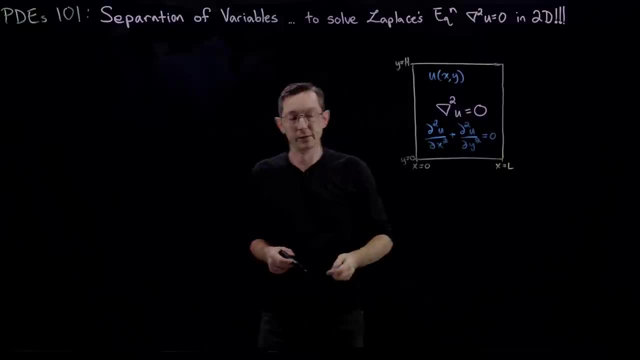 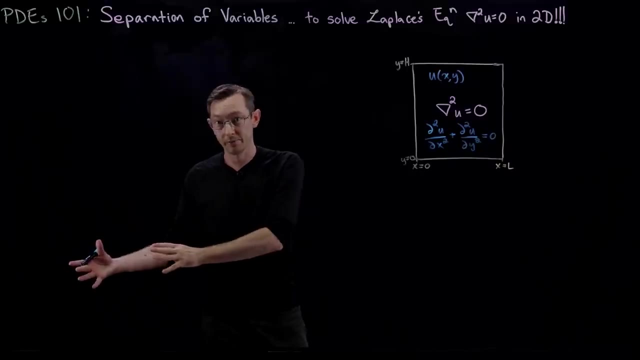 you know, the steady state heat distribution in terms of these partial derivatives with respect to x and with respect to y. So we're going to talk about the partial differential equation of u with respect to x and y And we derived the heat equation in the last lecture in two dimensions as, again, a conservation. 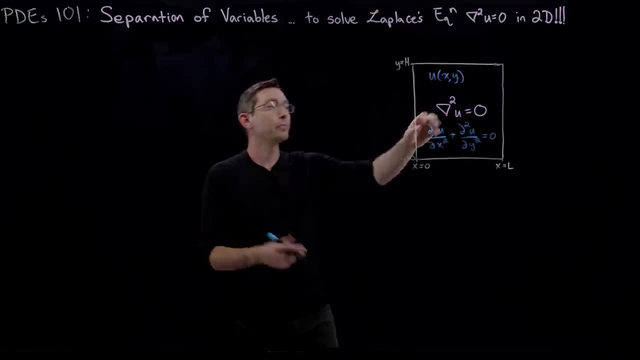 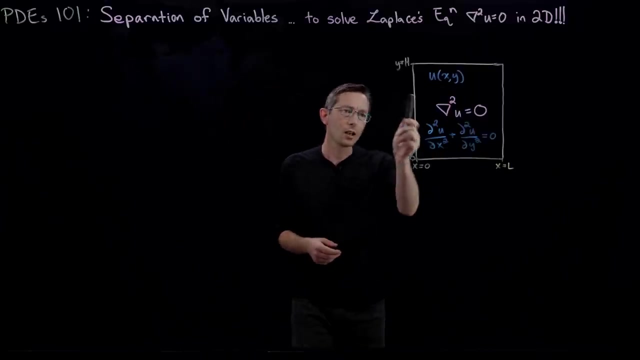 of thermal energy in a volume or on a square or on a rectangle, And if you take the limit as time goes to infinity- so that's what I mean by steady state- all the transients die out, then you arrive at this steady state heat distribution equation, given by Laplace's equation. Now we need some. 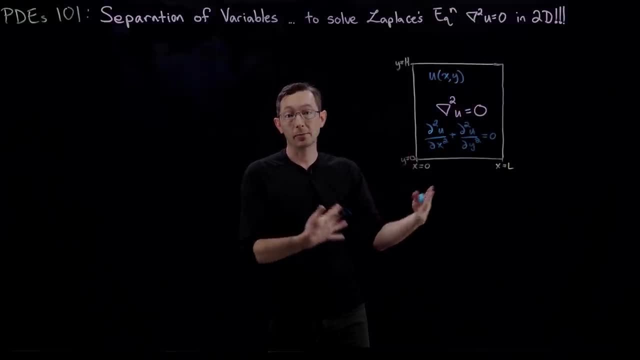 boundary conditions to make sure that we have a steady state heat distribution equation. So let's look at some of these boundary conditions. Here we have a well posed problem. So the first boundary condition on the left wall. so what we're going to assume is that we impose a constant temperature. 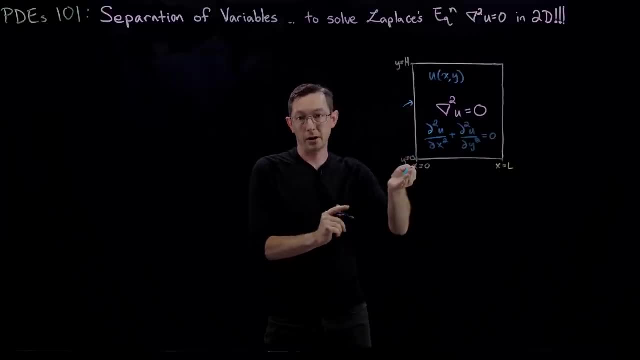 distribution on the left wall, the top wall, the right wall and the bottom wall. And so u at x equals zero. that's the left wall. for all points y, we're going to say that that equals f1 of y Some. 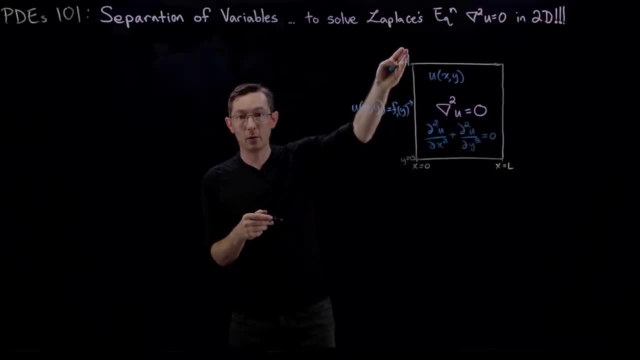 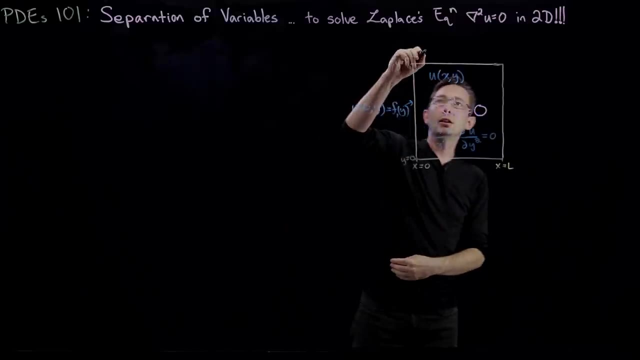 specified function f1 of y. So that's going to be f1 of y. So we're going to say that that equals f1 of y, which is a function of the y variable which goes from zero to some height: h. Similarly, we're going to specify at the top boundary condition: u. 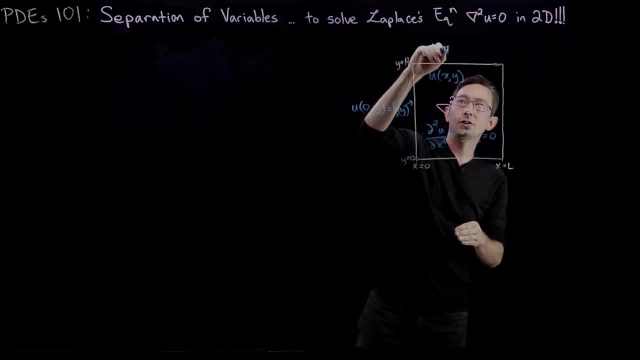 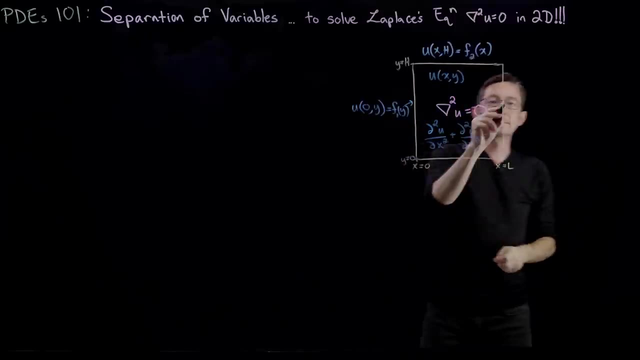 now this varies in x, u of x comma. h equals f2, and this is a function of x because it varies in the x direction. We're going to specify a right boundary condition again: u at x equals l. for all of these points, y equals f3.. 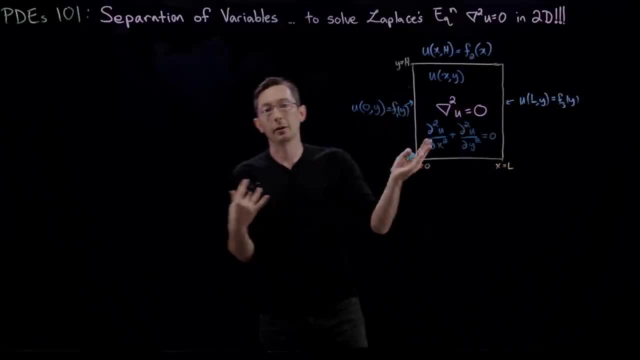 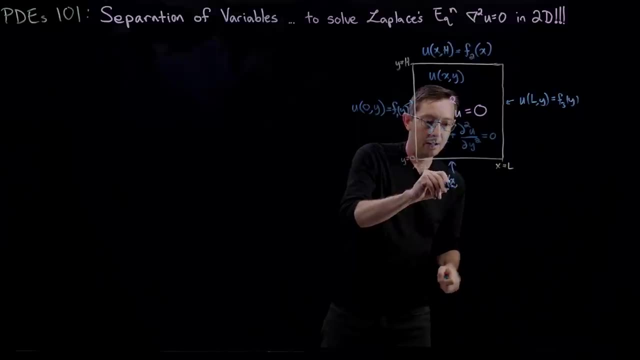 Again, this is a function that varies in y. And finally, we specify our fourth boundary condition at the bottom, which is: u of x, again, fixed at y equals zero. That's what the bottom line equals, f4, and this is a function of x. 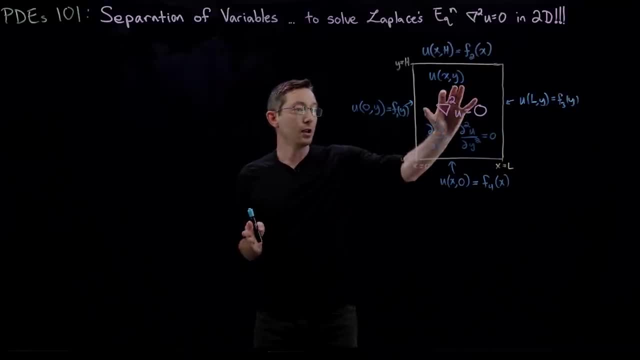 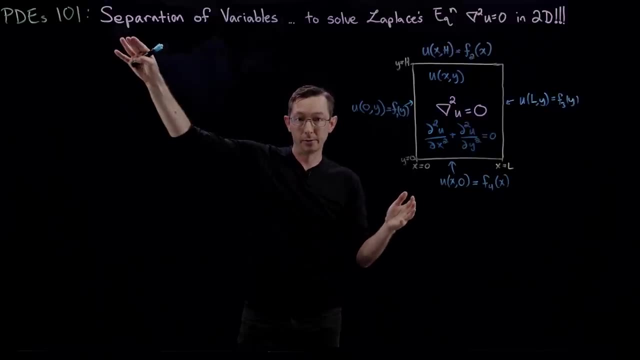 So okay, Now let's go ahead and do some math. Now we have a partial differential equation and enough boundary conditions that this is a well-posed problem. I'm going to walk you through solving this using the separation of variables. 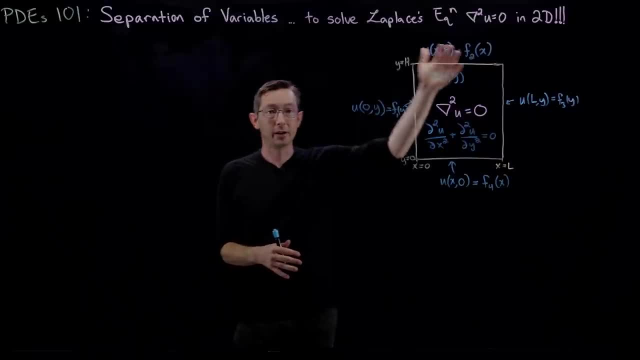 And this is actually kind of a gnarly problem to solve with all of these boundary conditions, And so one of the things I really like to do in my class. I think this is illustrative of how you take a complicated problem like this. 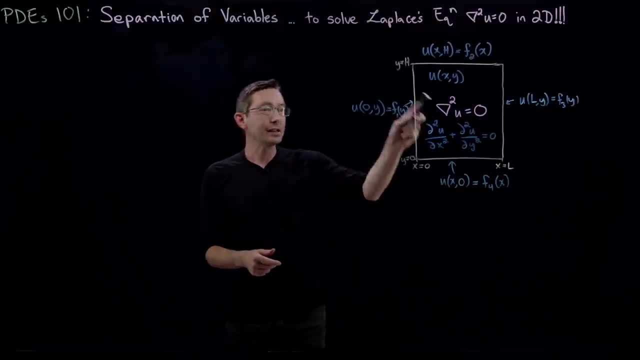 and break it down into a simpler problem, Because Laplace's equation is linear, meaning if I have, I had a solution u1 and a solution u2 and a solution u3.. If I add all of those solutions up, that is still a solution of Laplace's equation. 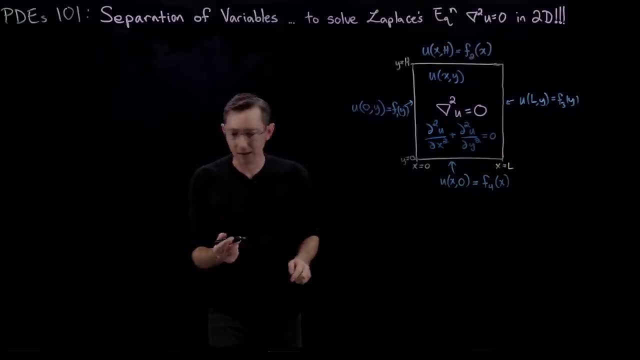 It's a linear, partial differential equation, And so what that means is that if I have this full set of boundary conditions, where I have, you know, f1, f2,, f3,, f4, and I have my solution: u of x, y. 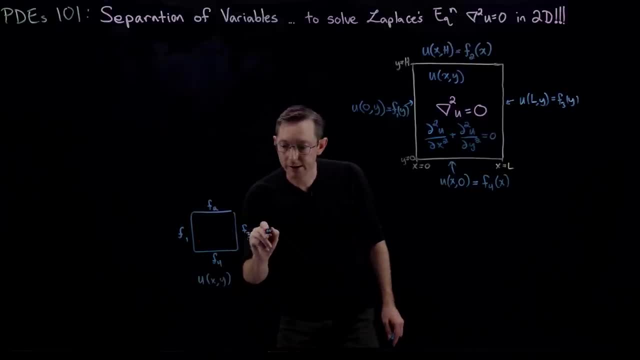 Okay, That's my full solution. This is equal to the sum of four simplified problems, where in the first problem I have f1, 0, 0, 0.. Okay, So I've kept my f1 boundary condition, but I made all of my other ones 0.. 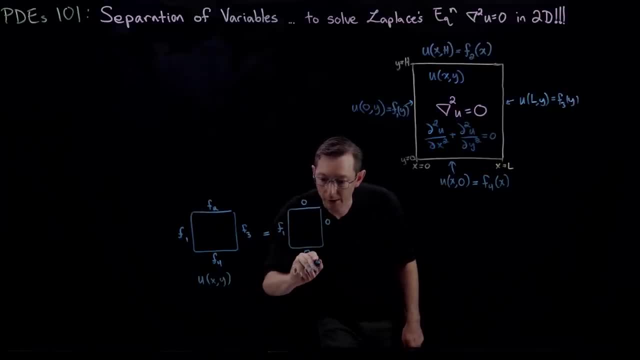 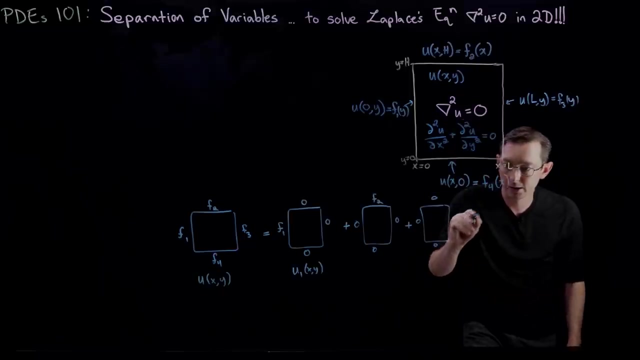 We're going to call this u1 of x and y, plus another set: 0, f2, 0, 0 plus 0, 0, f3, 0, plus 0, 0, 0, f4.. 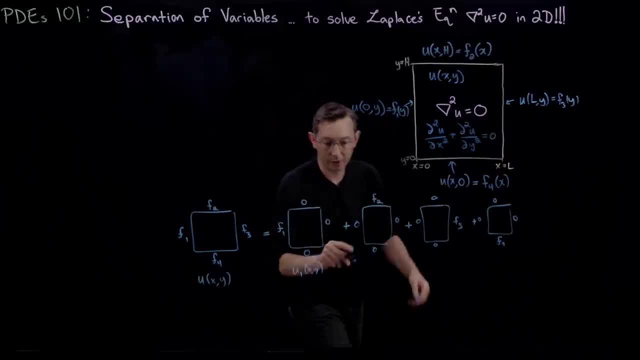 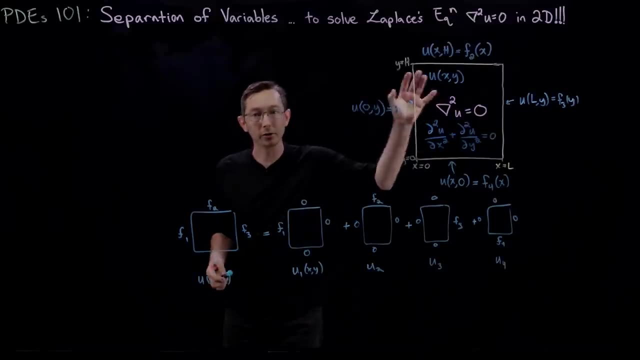 And again, the solution of each of these sets of boundary conditions is u1,, u2,, u3, and u4.. And because this is a partial differential equation that is linear if I add up these four solutions- u1, u2,, u3, and u4,- 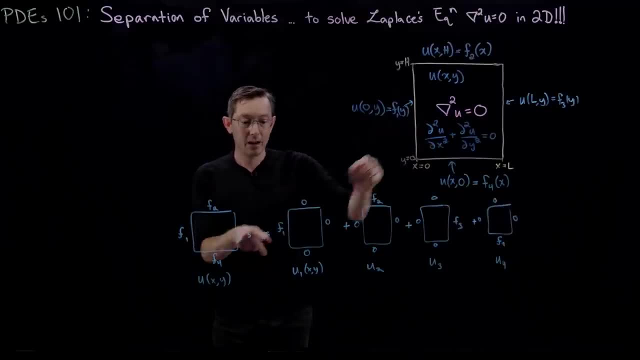 it is a solution again of Laplace's equation. It is a solution of u1,, u2,, u3, and u4. That satisfies the boundary conditions f1,, f2,, f3, and f4 at those four sides. 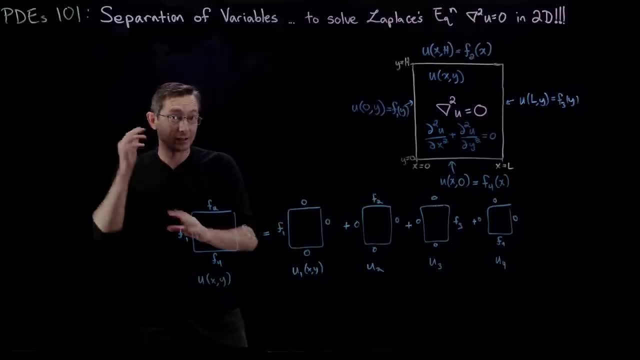 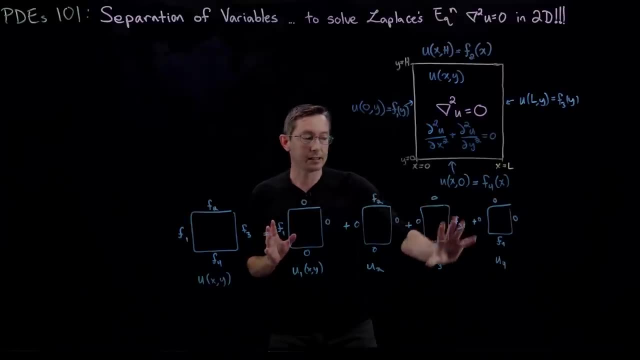 So I'll show you in this video. So this is going to. My guess is this is going to be like 30 or 40 minutes. So buckle up. I'm going to pick this one here because this is the easiest one for me to solve with the boundary conditions. 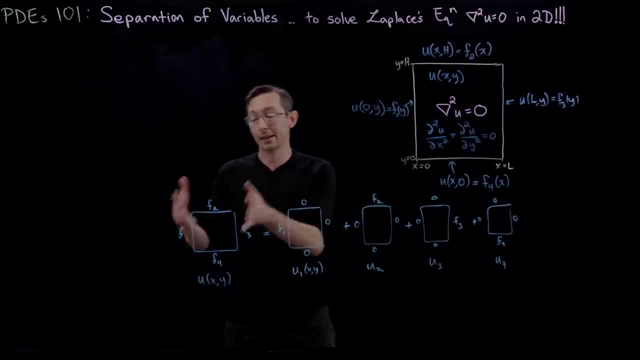 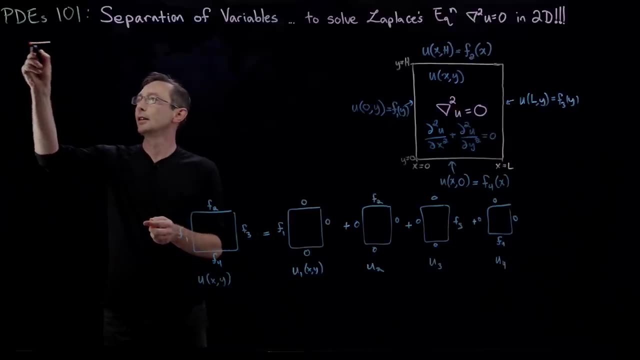 And then, as kind of a homework problem, you can solve these other ones and add them up to get the full solution. So I'm going to pick this problem here And I think I should just probably I'm going to write this out, as this is where we're going to remember. 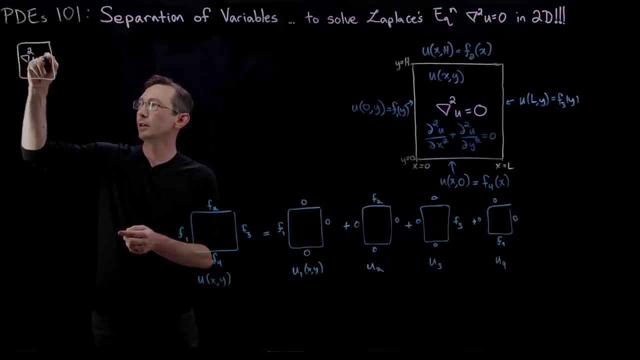 what problem we're solving. So we're solving: del squared, u equals 0 with the boundary conditions 0, 0, f3, 0.. Let's call this f3 of y, And I'm just going to write down my boundary conditions. 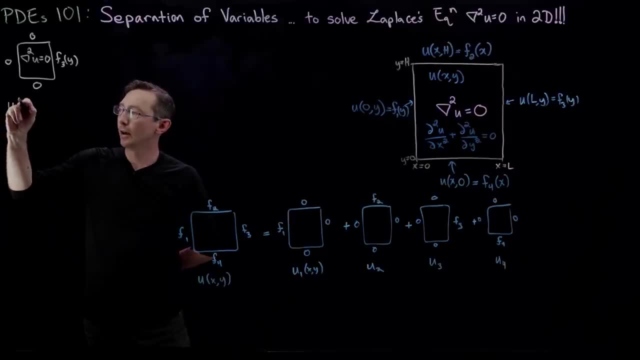 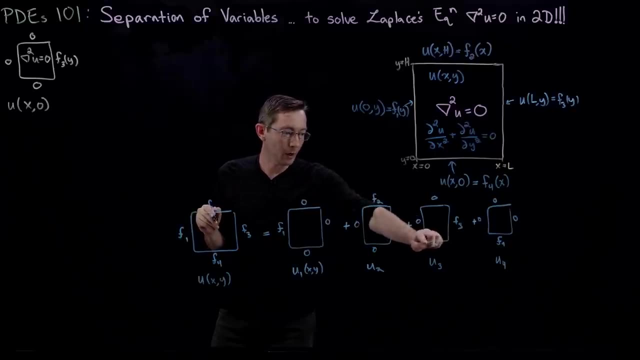 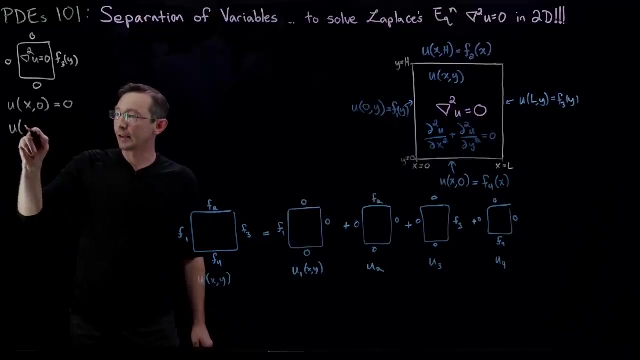 to be very, very explicit. So I have u of x- 0.. So u of x at the y equals 0, is 0.. I have u of x at the top of my square at h, also equals 0.. 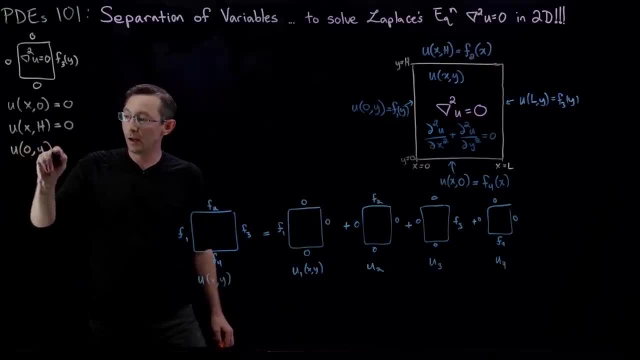 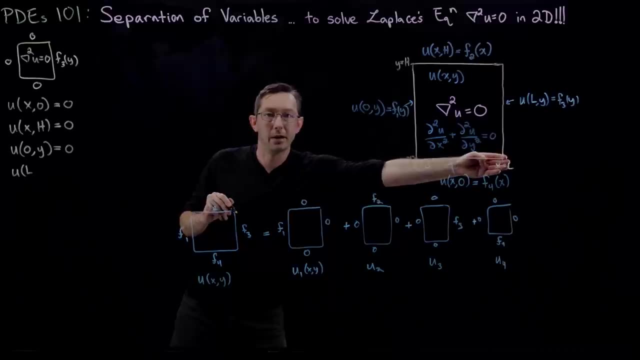 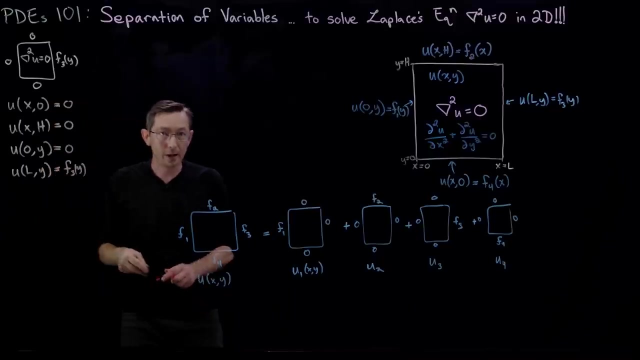 I have u of x equals 0, all along, y equals 0.. And I have u of x equals l. at the far length of my domain, for all points, y equals this f3.. So these are my boundary conditions. This is the problem we're going to solve. 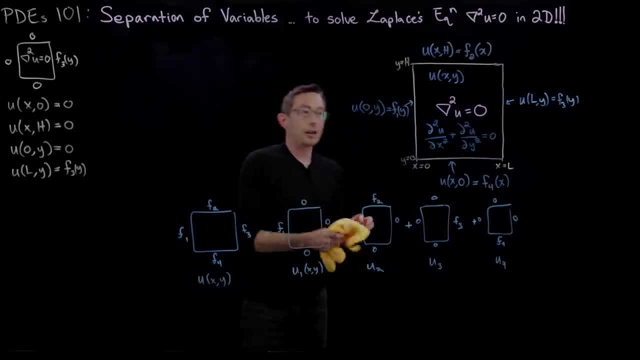 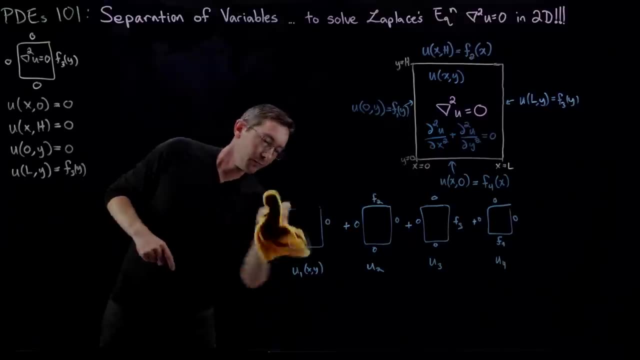 And we're going to solve it using separation of variables. Okay, good, I'm going to erase this because I need all the board space I have. If this takes too long to erase, I might speed it up. All right, Time travel. 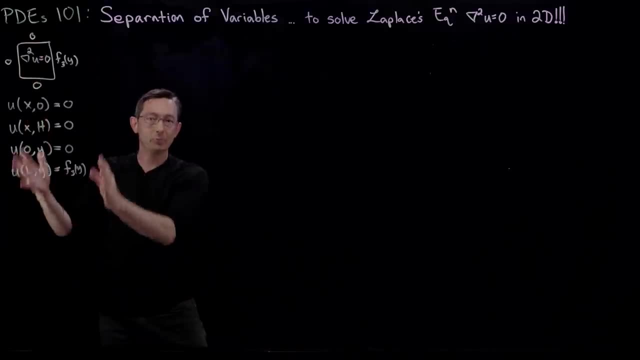 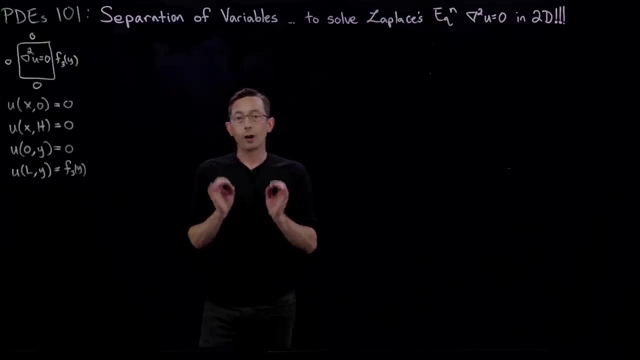 Good. So now we're going to solve this simplified problem of Laplace's equation using separation of variables, And this is So. this is an incredibly powerful technique which essentially, was introduced by Jacob Bernoulli in 1690.. And 1690 was a very, very interesting time in Europe mathematically. 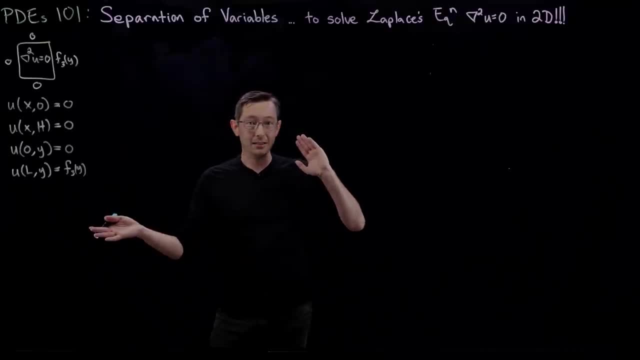 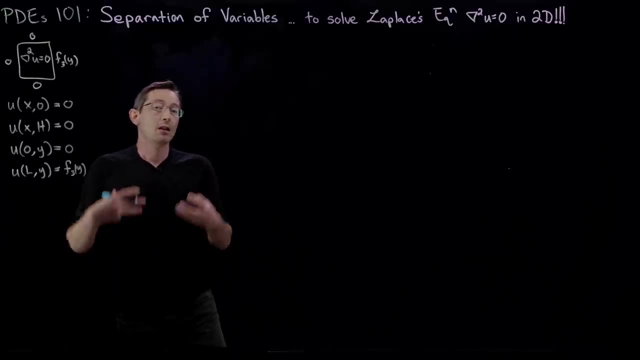 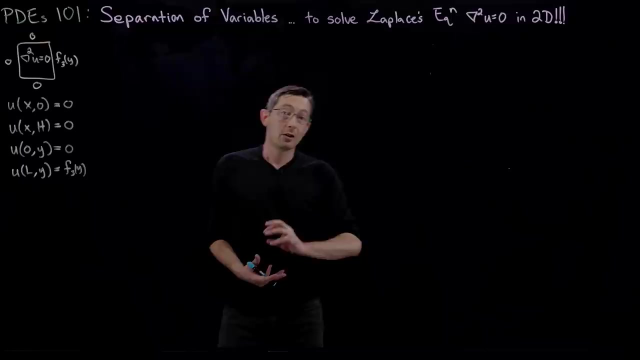 So, if you think about it, in that century, from 1600 to 1700,, Kepler had used Tycho Brahe's data to solidify the Copernican model, with the sun at the center of the solar system. Galileo had been imprisoned or under house arrest and died in his home. 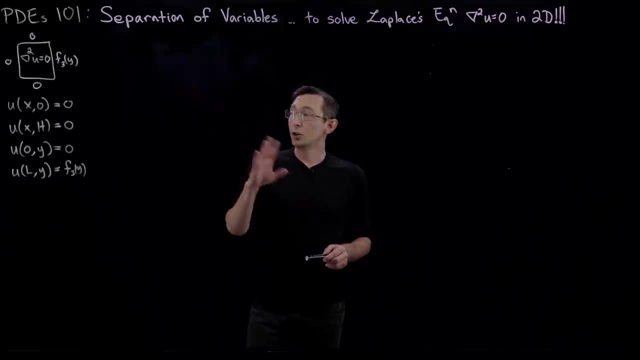 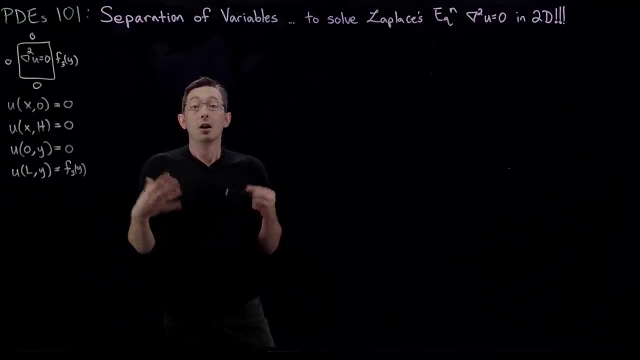 in the middle of that century, And two or three years before Jacob Bernoulli introduced the separation of variables to solve this isochrone problem, Newton released his Principia. So just an incredibly rich time in the history of math and physics. 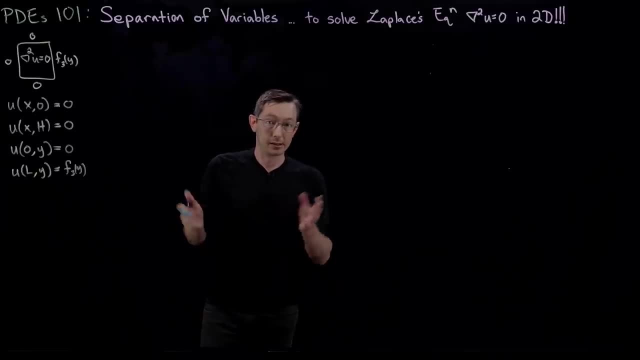 And I actually think that the separation of variables is a very, very important thing. And I actually think that the separation of variables is a very, very important thing, And I actually think that the separation of variables is one of the culminations of this kind of rich thought environment. 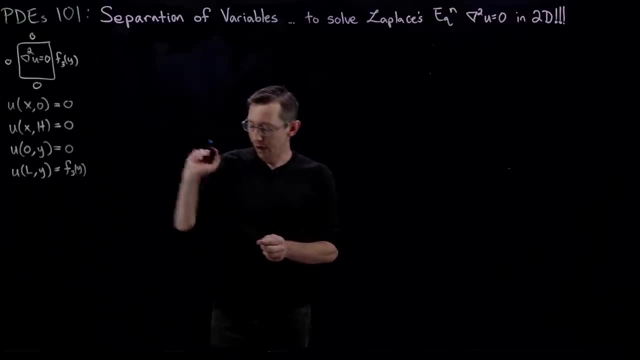 So the idea is that we are going to take our solution. So we're gonna say u of x, y. This is a huge assumption. We're gonna say that this equals some function of x, some function in the x direction. 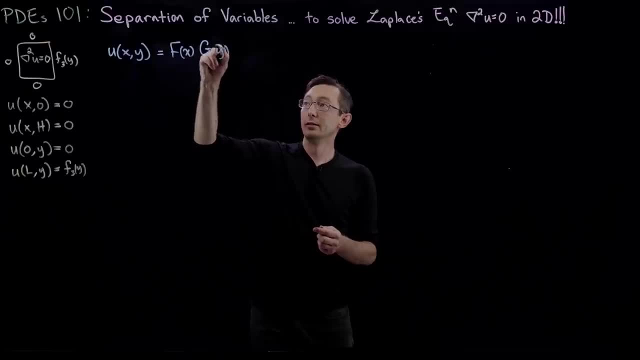 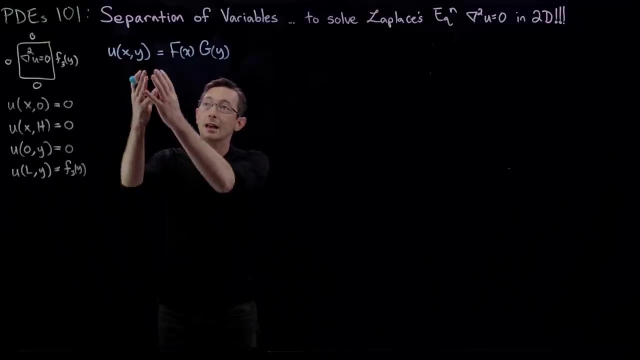 times, some function in the y direction. Now, this is a really big assumption. We're assuming that this is a really big assumption. We're assuming that this is a really big assumption. We're assuming that this is a really big assumption- that these dynamics in X and Y can be split into the product of functions of X. 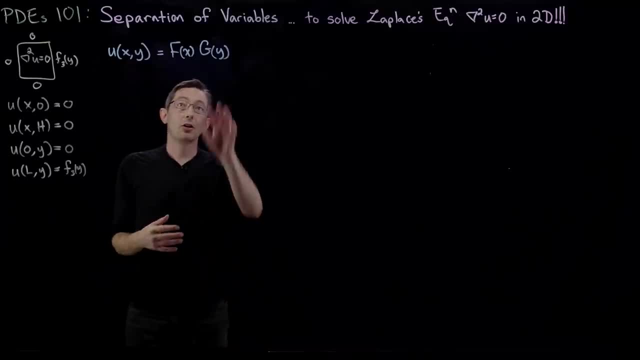 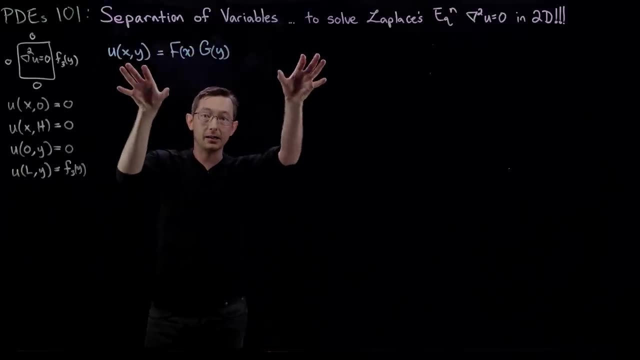 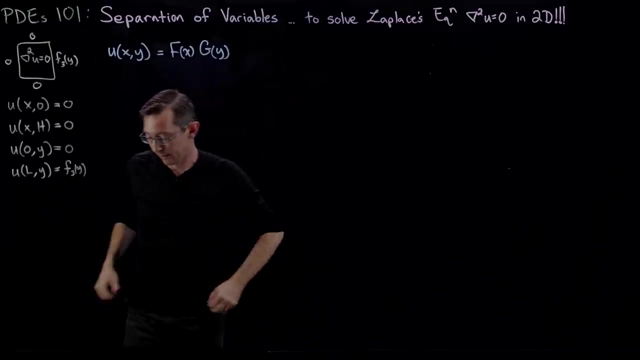 times functions of Y. Now, that means that there are no weird cross terms here. like well, this means that I can factor my solution into a term, a set of terms in X and a set of terms in Y, but that it is separable into into those two functions. 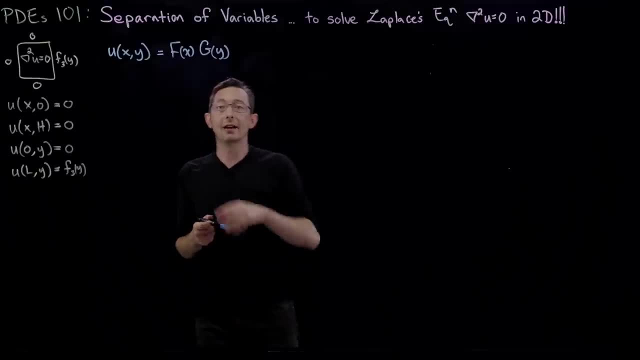 So I'd actually like you to think of some examples of functions of X and Y that are in unseparable, that cannot be split into this. I'm thinking of things like X plus Y squared. X plus Y, quantity squared is, is not separable in this way. 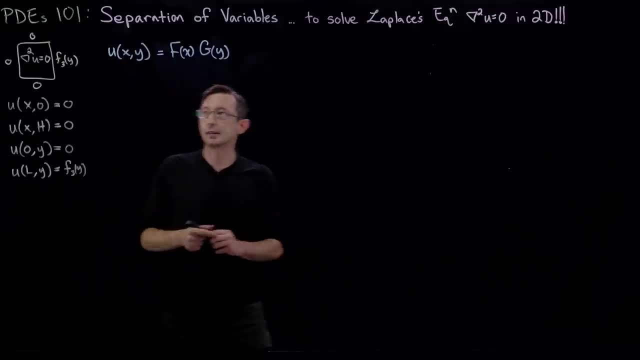 I don't think You should double check that. I just made that up on the spot. Okay, so the first assumption- this is a huge assumption- is that we are going to assume this separation of variables and then what we're going to do is we're 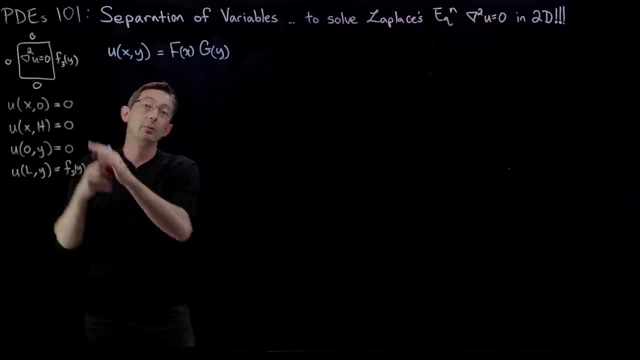 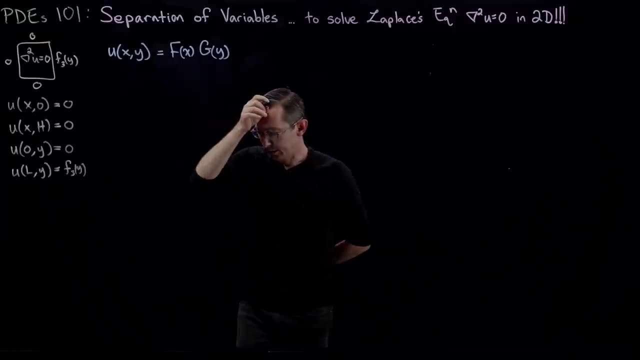 going to plug this into our partial differential equation and then we're going to plug this into our partial differential equation and we're going to get ordinary differential equations for F and for G that have to be satisfied. So let's do this. So if I do del squared of U and remember this is: 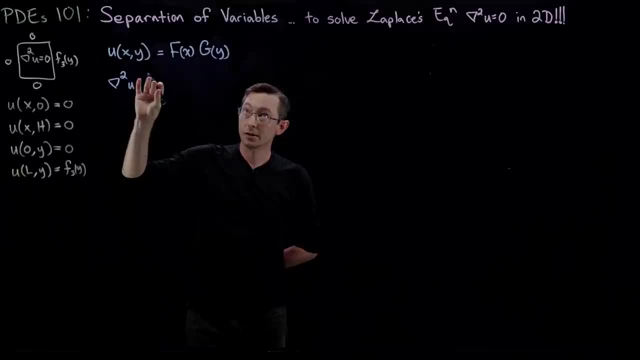 partial squared U, partial X squared plus partial squared U, partial Y squared. Okay, so partial this, and again we're going to do the chain rule. so the second partial derivative of this with respect to X is just F X, X. subscript here means partial derivative. I took two partials with. 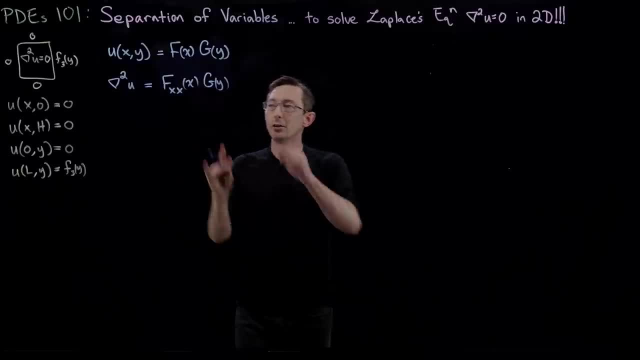 respect to X times G of Y. now you could say plus F of X, g, X, x of Y, but since G is a function of Y, it's partials with respect to X are zero. Okay, Okay, so this is the first term of Laplace's equation. 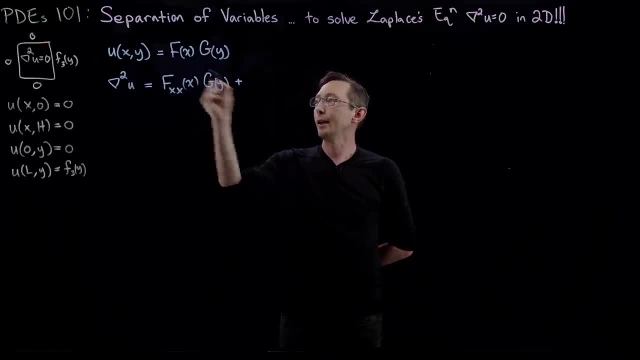 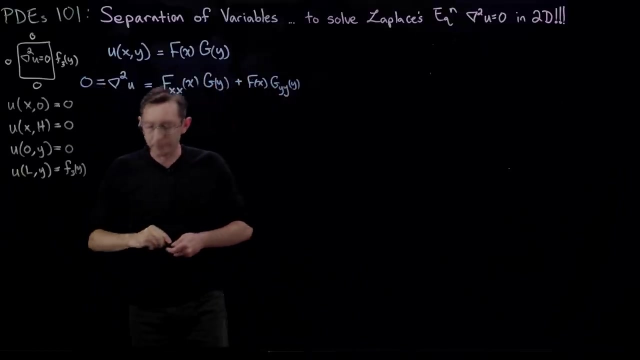 the second derivative, and X plus the second derivative and Y is again F of X, g, Y, Y. Okay, So you have, you're Van der Waals kin againstл of y, and of course this equals zero. okay, we know that this equals zero. good, so so. 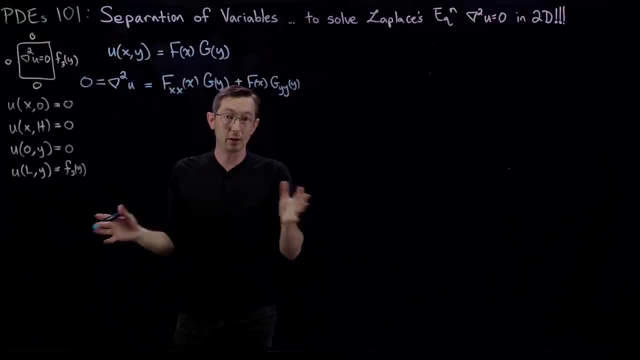 this is Laplace's equation, if we assume that we can split our function u into a product of f of X and G of Y, and so now what we're going to do is kind of play around with these a little bit. so I'm gonna move one of these over to the 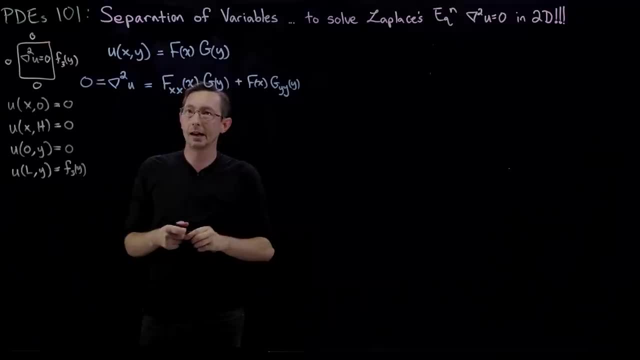 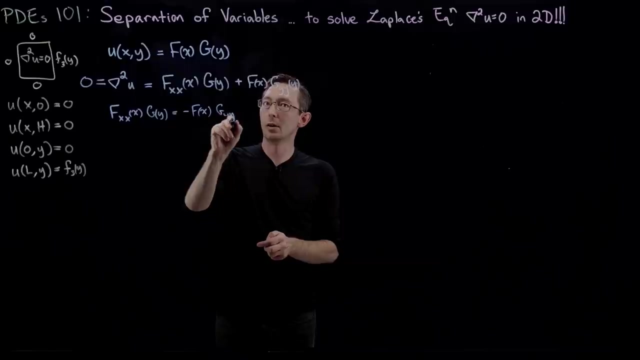 right hand side, because both of these add up to zero, so I can move one over to the right hand side and I can say so. I'm gonna rearrange this and say: f x, x of x times G of Y equals minus f of x, G, y, y, y. and now I'm gonna collect all of my f. 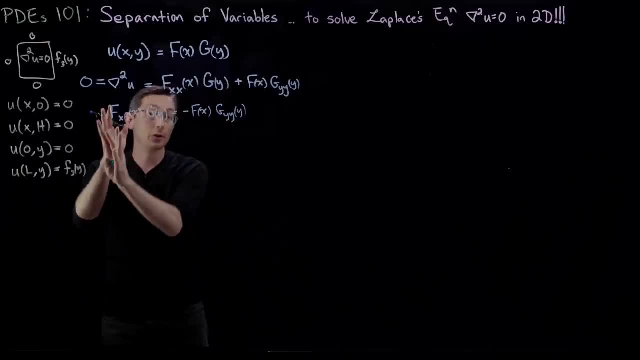 terms in one side and all of my G terms on the other, everything that's a function of x and everything that's a function of y on different sides of the equation. and I'm going to get f and X, X divided by F, these are both functions of X. equals minus G, Y, Y over. 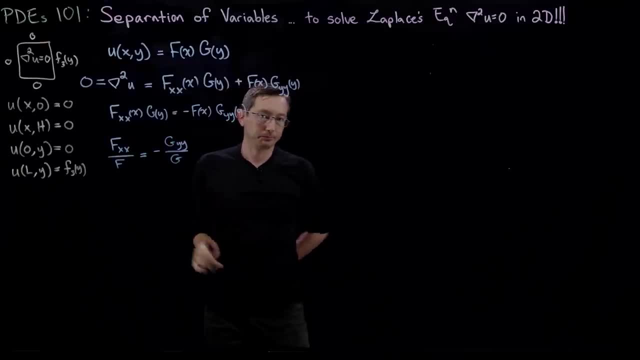 G. okay, because these are, I collected all of my G, my Y terms over here and all of my X terms over here. good, so this, if you think about it, only is a function of X. so, even though these are partial derivatives with respect to X, F is only. 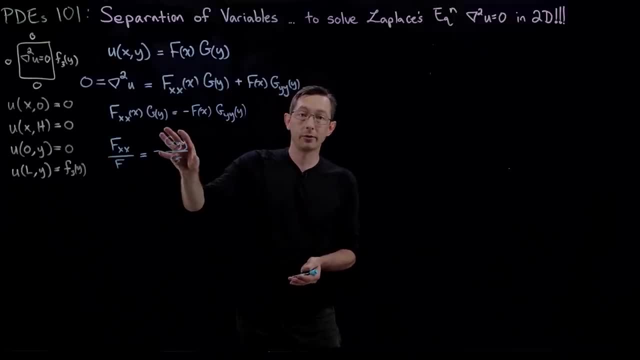 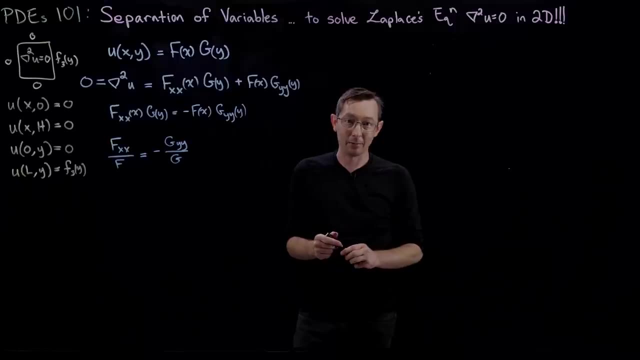 a function of X. so these are just normal derivatives. and these are normal derivatives with respect to Y. and one of the really cool things about separation of variables is this: next step is that these two equations, because they equal each other, these, these two terms equal each other. they both have to equal a. 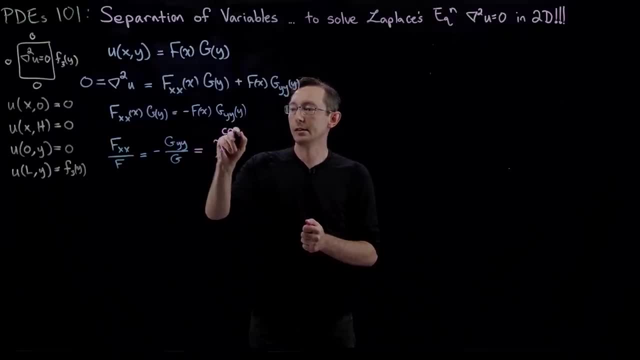 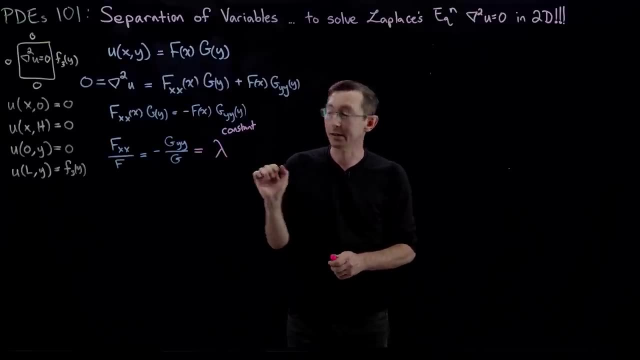 constant, lambda. so I'm going to say this is a constant and if you have watched my videos before, you know that I love eigenvalues- lambda. so I am calling this lambda because this is going to be an eigenvalue. you'll see that in a few minutes. but these two terms have to be constant and 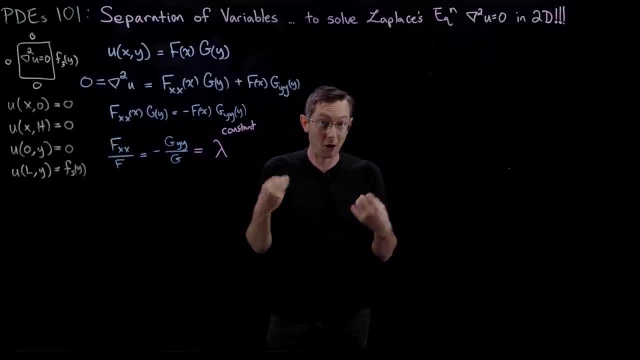 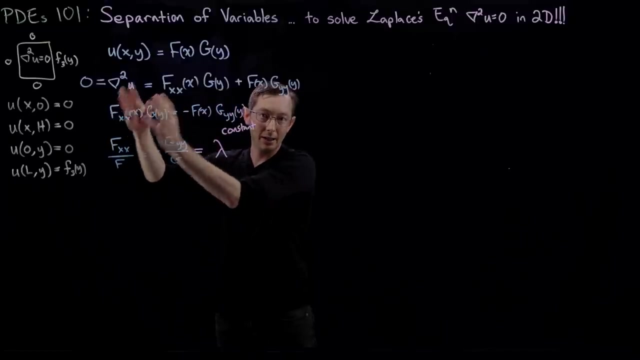 and I always pause and I ask my students to think hard about why this is. so I'm gonna pause for a minute and you're gonna think I got these equations by taking this. you know partial differential equation equals zero. so I move terms over. I divided and collected like terms. you know my X terms and my Y terms. why do 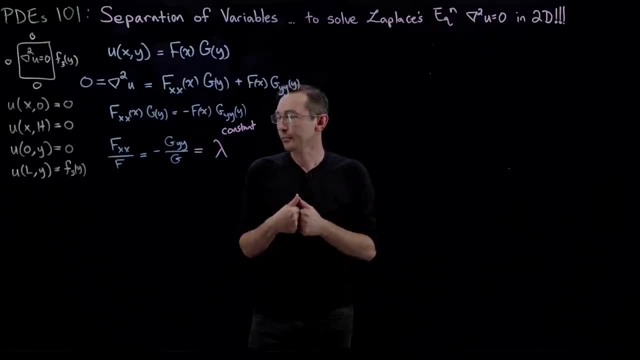 those have to equal a constant. and the answer is because if this is only a function of X and if this is only a function of Y, then for any Y value- I, I very you know this equation- it still has to be equal to this one at every single. 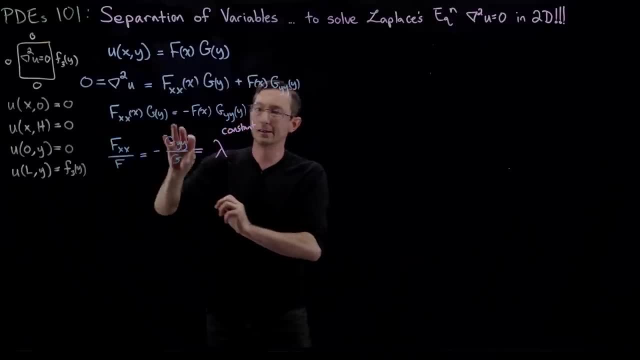 X value. so, because this is only a function of X and this is only a function of Y, the only way that those can equal each other is if it's the constant function. if it's like you know, 1 equals 1 or 2 equals 2, you can't have x equals minus y. 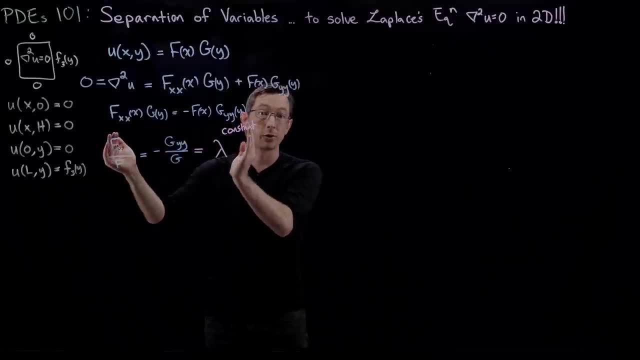 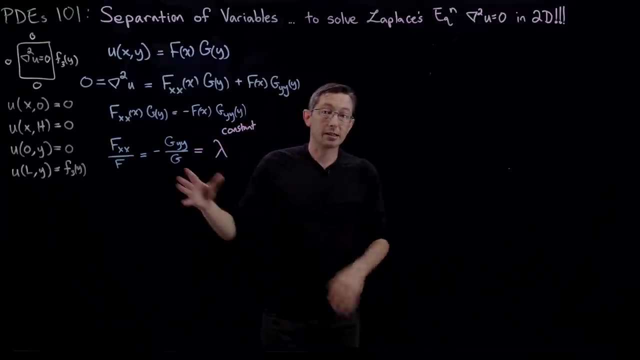 for all why? and for all X. so the only way this is true for all y and all x is is that they both equal of constant good, and so we're actually getting really close to starting to solve this problem. so we still set this up, and I'm gonna 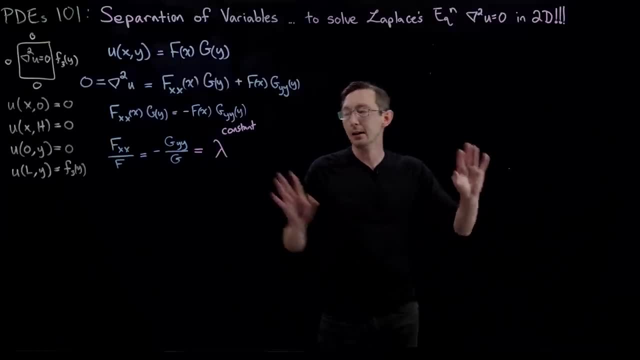 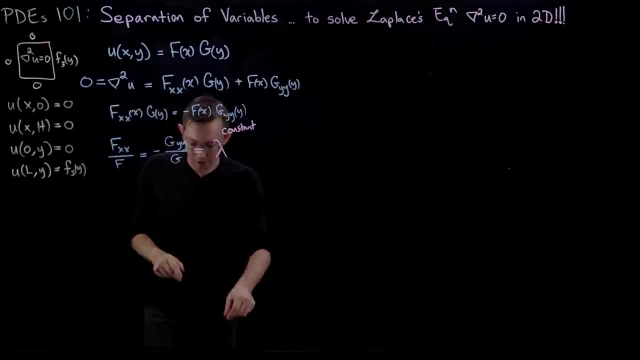 take a big step back and or you can jump ahead to the summary, or, you know, I'm going to have these summary moments where I summarize all the steps, but I'm going to keep going just a little bit. So what we've done so far is we have 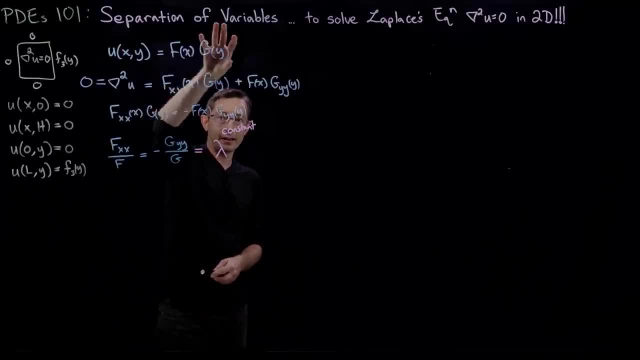 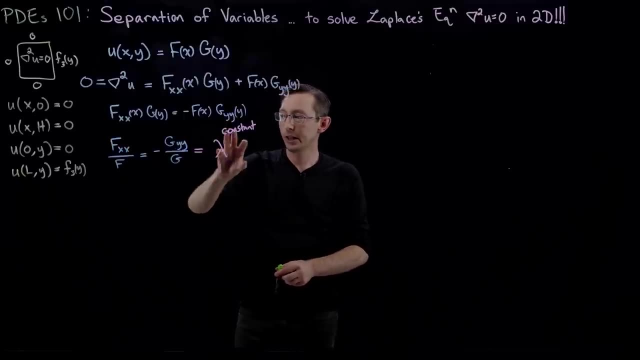 assumed that we can split our function into a product of f of x times g of y. We've plugged it into our partial differential equation and now we have recovered this relationship which I claim is two systems of ordinary differential equations. So this, in my mind, is two systems of ordinary. 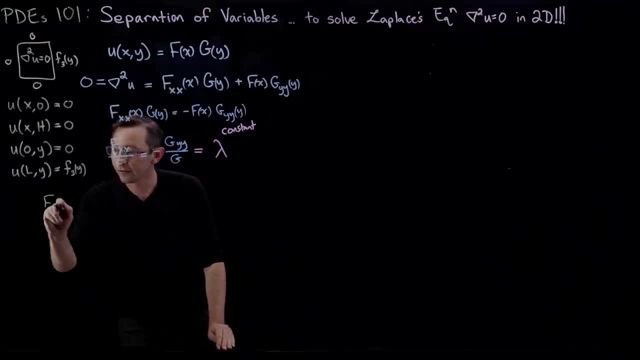 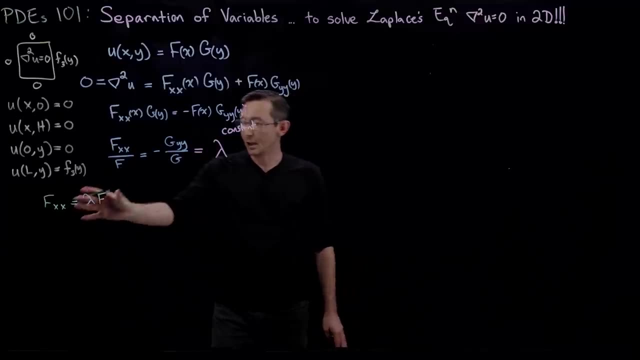 differential equations. We have f, x, x equals lambda f. Okay, this is a ordinary differential equation in f of x. Okay, f is a function of x. so you, really you could think of this as like: f prime, prime equals lambda f. We know how to. 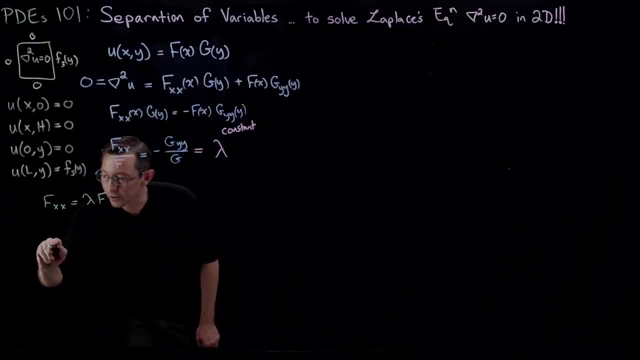 solve this And we have another differential equation: g y- y equals, minus lambda, g- y. And if you're a little quicker than I am, I've been thinking about this so I know the answer. but if you're a little quicker than I was, you'll recognize that. 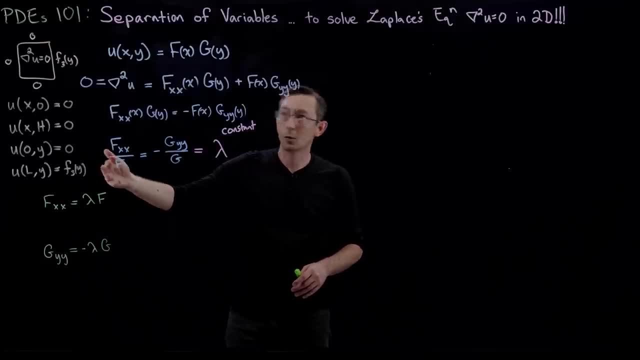 the solutions of this are going to be things like plus or minus, you know, either the plus or minus root lambda t or root lambda x, and solutions of this are going to be things like sines and cosines of root lambda y's. Okay. so these solutions. 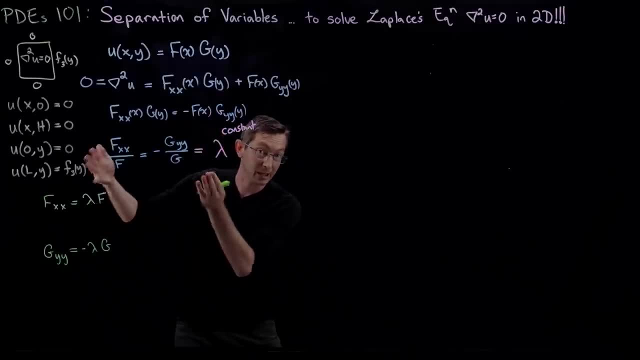 of these are going to be sines and cosines. Solutions of these are going to be exponentials, Good And importantly, these have our boundary conditions here translate into like initial conditions for our ordinary differential equation. So at f we're going to use our, our x equals 0 and x equals l conditions here. So f of 0 equals. 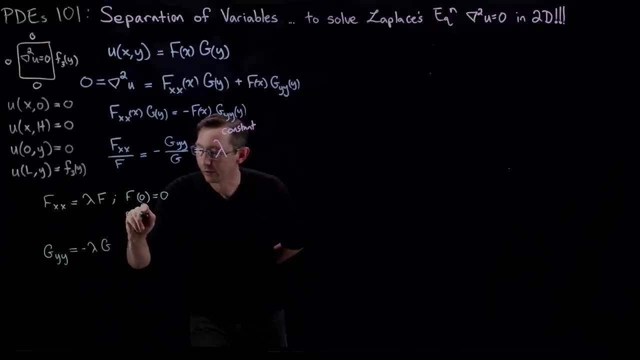 0 and f of l. f of l has to equal f. 3 of y. Okay, this is a little messy, I'm gonna. I probably shouldn't have written that down, but the x equals l condition is going to come from this one And 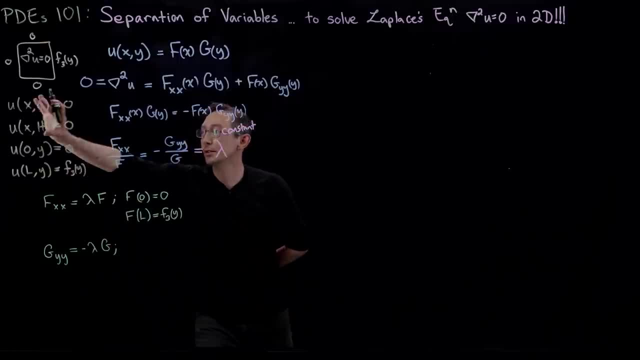 similarly, we have these conditions on g- g ones are easier- which is: g at 0 has to equal g at h has to equal 0.. Those are these, these conditions here. Okay, so now what we have is we've turned our nasty partial differential equation into a. 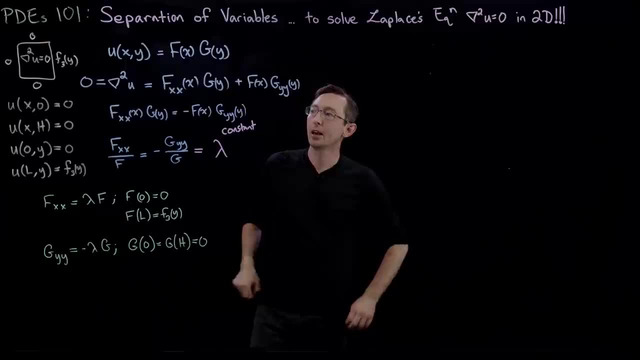 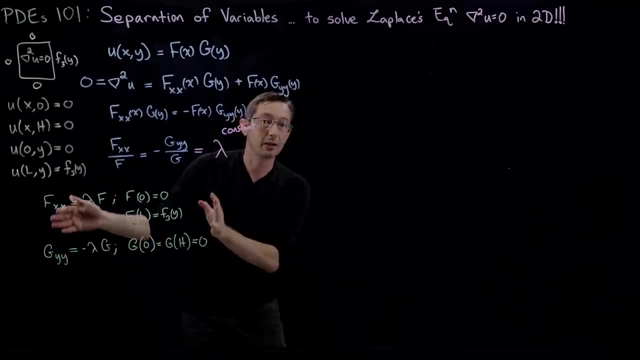 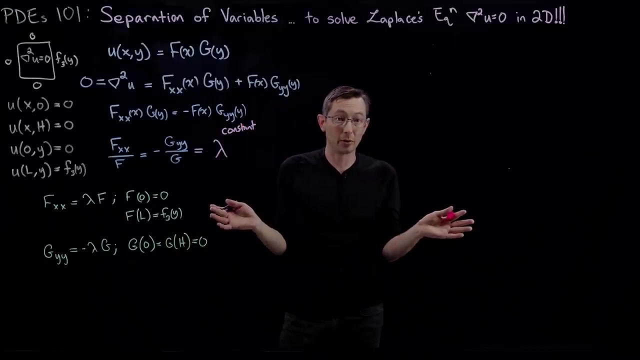 function, which is a function of x and y, you know two spatial variables, And we have, by separation of variables, shown that now we can reduce this to two systems of ordinary differential equations. And these ordinary differential equations it's actually a whole family, It's infinitely many ordinary differential equations, for 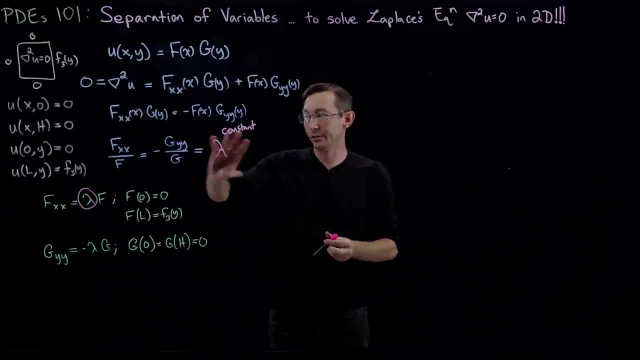 any value lambda that I choose Any value lambda here. this is absolutely true. If this is pi, if this is negative 2, if this is 15, this is still true. And so I get this whole family of ordinary differential equations I solve, But I'll 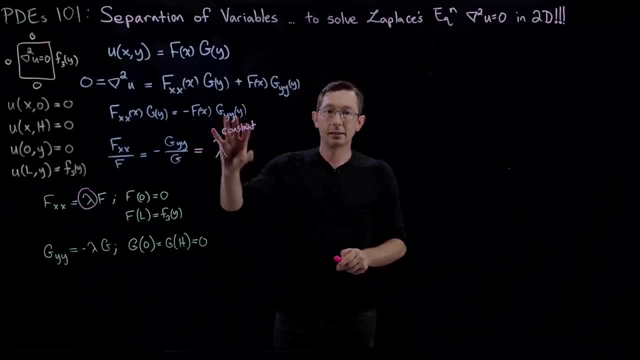 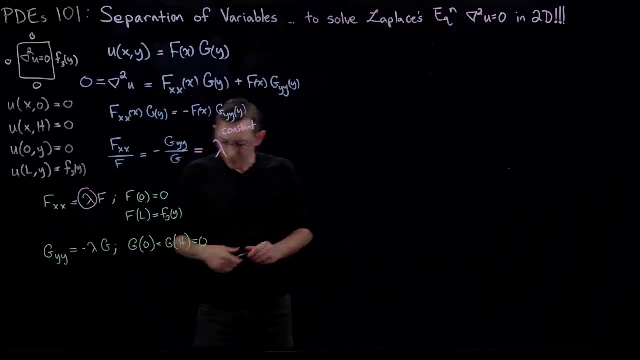 point out that, even though any constant lambda makes this true, only special lambda- remember, eigenvalues are special values. only special eigenvalues lambda will allow me to satisfy these two sets of boundary conditions, These kind of ODE initial conditions. So that's really important. Okay, good, And I'm 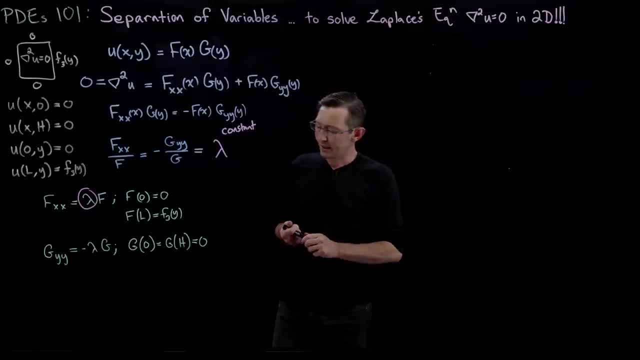 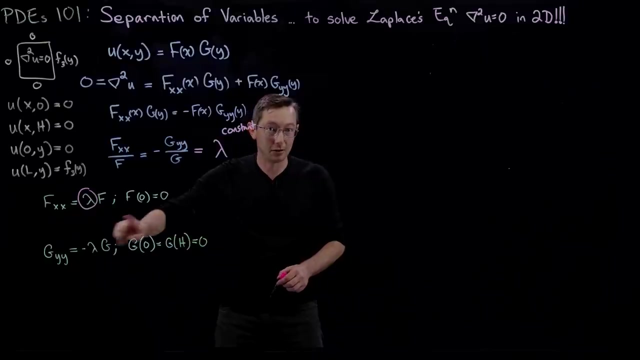 just going to think for a minute: Yeah, realistically, this, I'm going to erase this one, We're going to come back to this boundary condition. So I think at this point you should be seeing: this looks like a much easier system to solve because I have really easy. my boundary conditions give me really easy. 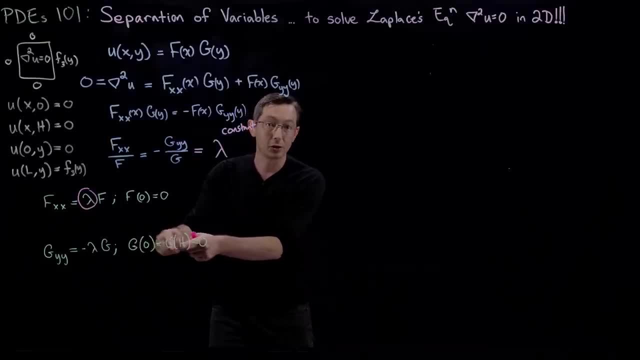 kind of constraints on my solutions here, whereas the F variables are going to be nastier because this right-hand side imposed temperature distribution. So that's going to be a little hairy. So I'm going to solve this GYY equation. first I'm going to find which special lambdas 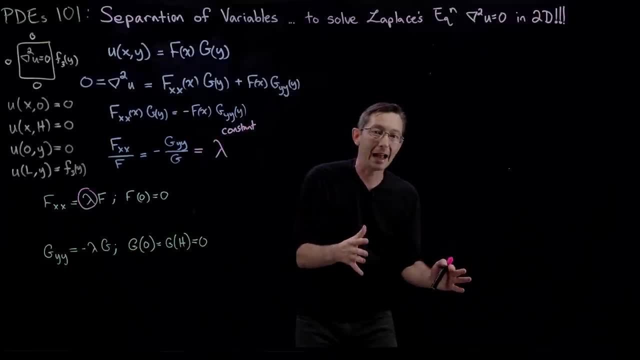 allow me to satisfy these boundary conditions And then, once we have those special lambdas, we'll solve F and we'll take all of our solutions and we'll plug them back in to reconstruct U of XY. Okay, So that's what we're doing. Good, I think we should just get into it. We're already. 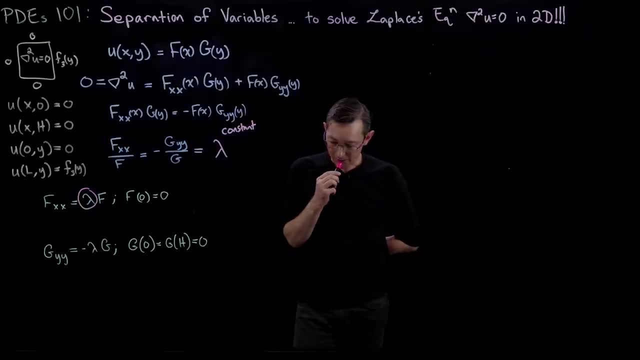 pretty far into it, So okay. So now, what I want to do is I want to solve my GYY equation. I might just do it down here, because I think I have enough space. Okay, So, GYY. Now we have a. 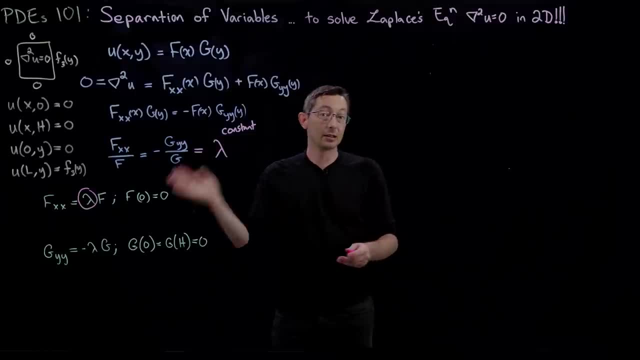 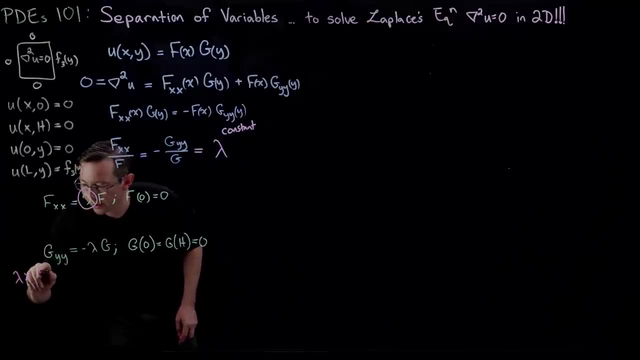 few different cases. We could do it if lambda is positive or if lambda is negative, Okay. So if lambda- let's say lambda- is greater than zero, Okay, I'll let you think about what happens when an interesting case, but let's just think about this for now. So if lambda is greater than zero, 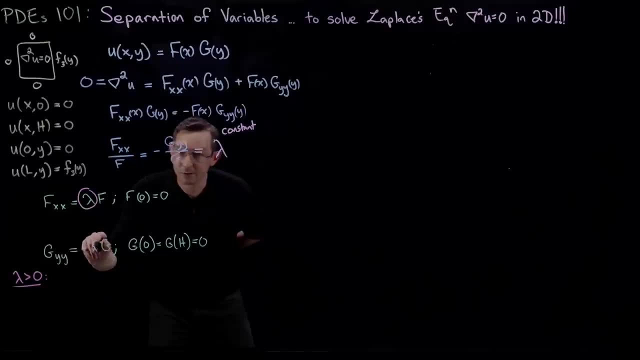 then essentially this GYY equals minus lambda G. The solutions of this are sines and cosines. This is literally G. prime prime equals minus lambda G, And we know so you could assume. if GY equals E to the alpha Y and you double differentiate it, you'll find that the eigenvalues of this have to be: 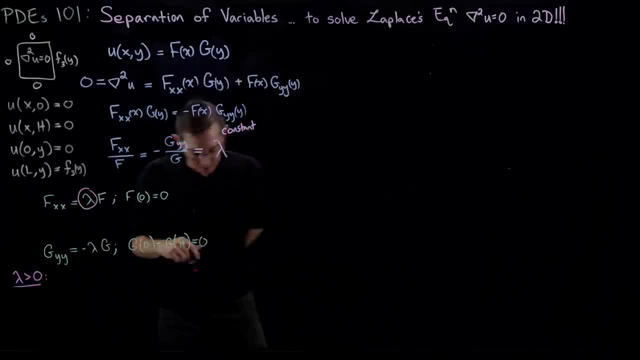 complex conjugate pairs, plus or minus I, omegas, And so we know that we're going to have solutions- are sines and cosines, And so we're going to say that our GYs are equal to zero, Because G0 equals zero. I can't have any cosine components, So I could write down you. 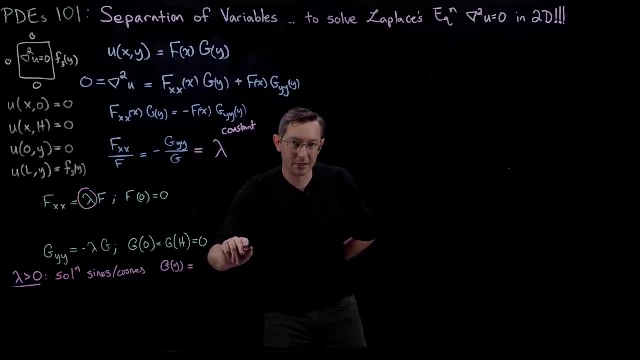 know sine of root lambda Y plus cosine of, you know, root lambda Y, But I can't have any cosine term because of this boundary condition, Because a cosine of zero is one, it's not zero. So I'm only going to keep my sine term, So sine of root lambda Y. And now I have to find the really. 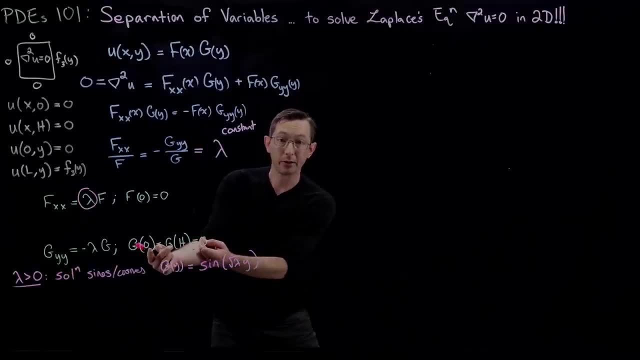 really special root lambdas that satisfy both of these boundary conditions. So we know that sine of, you know, root lambda Y is zero when root lambda is zero, or pi, or 2pi, 3pi, 4pi, 5pi. So I'm 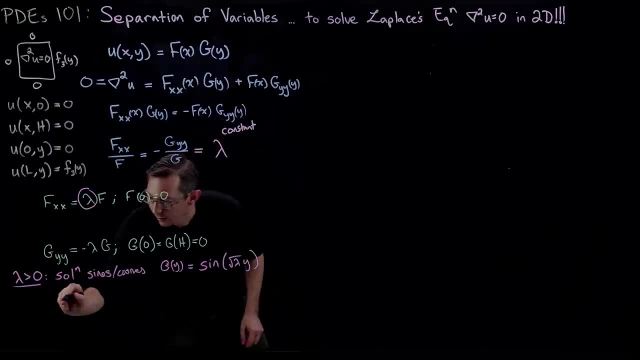 going to basically say that if root lambda equals some integer multiple of pi- and I'm pretty sure I needed this to be Okay- So when G of H, when I plug in so lambda, root, lambda H has to equal an integer multiple of pi. 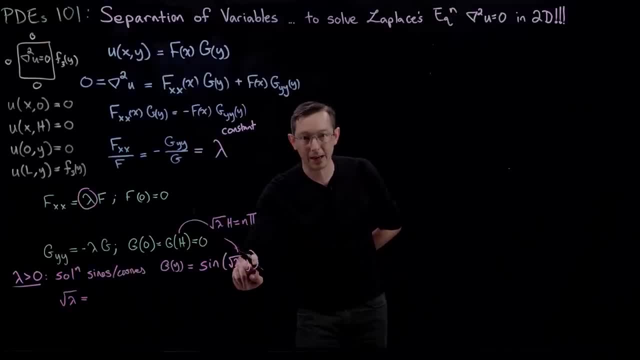 When root lambda times H- because I plug in H here- when that equals an integer multiple of pi, then this satisfies that right boundary, that top boundary condition. So that's my condition- is that root lambda equals N, pi over H. Essentially, for all integers N for N equals 1,, 2,, 3,, 4,, 5,, 6, so on. Okay, So for N equals 1,, 2,, 3, dot, dot, dot, dot dot. 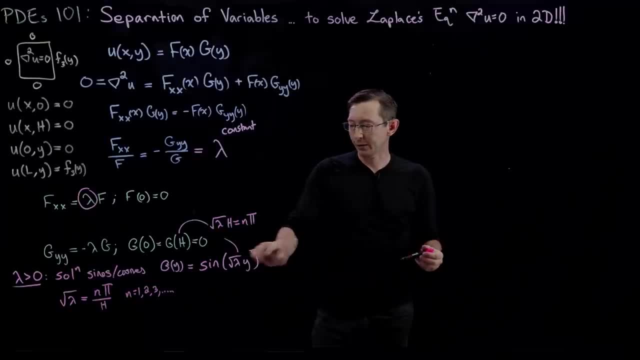 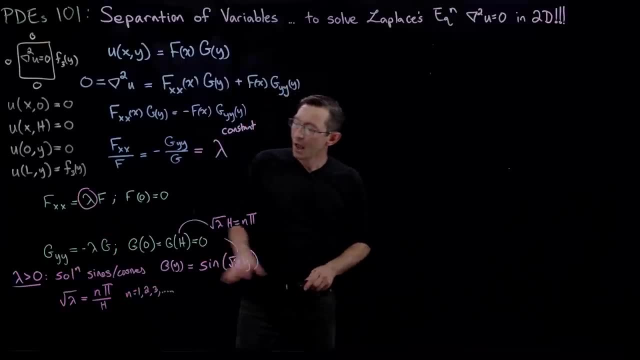 If N equals zero, that's also fine. You can kind of work that out that if N equals zero, then this is just sine of zero, It's just a, it's zero, And so that's also totally fine. So now we have come to a important kind of crux, which is we know that this equation was true. 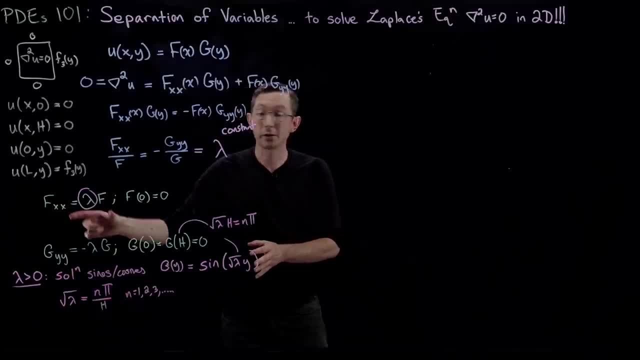 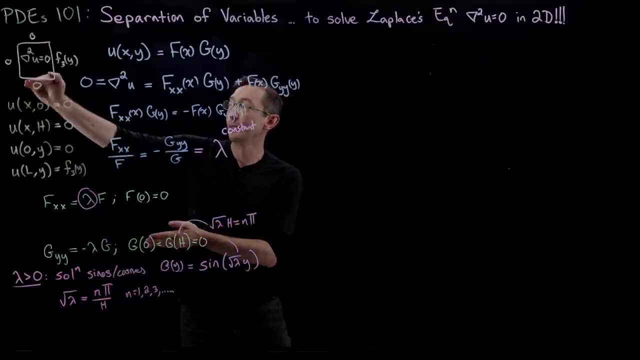 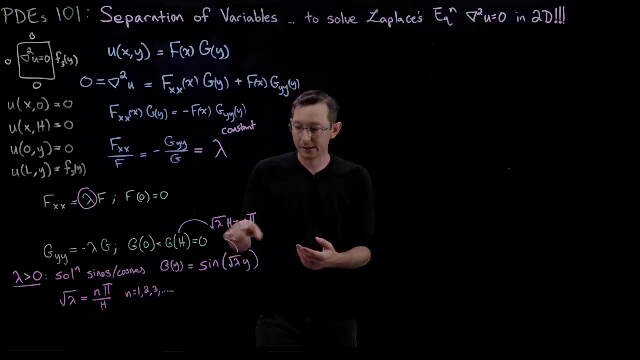 true for all lambda, and so these differential equations are also true for all lambda. But there are only very special lambda that satisfied these boundary conditions, the bottom and top boundary condition of my PDE, and specifically they're the, they're the, the lambda's that satisfy this equation, so that sine of root lambda Y equals 0,. 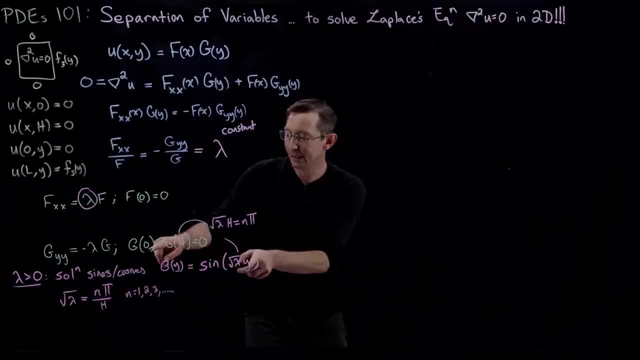 when Y is 0 and when Y is H. Now it's easy: every time Y is 0, this is 0, but when Y equals 0 and every time Y equals H, this is 0. But when Y equals 0 and every time Y is 0, this is 0, but when Y equals 0, this is 0. 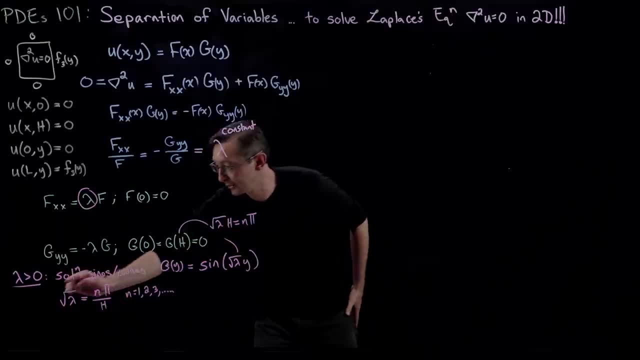 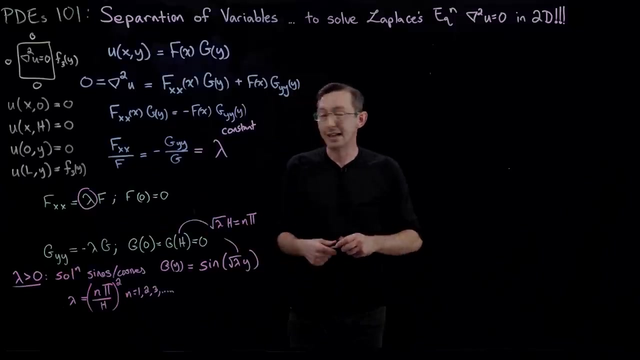 equals h. I need this special relationship for lambda. So lambda has to satisfy this equation And I'm gonna get rid of my root here and I'm gonna square my other side. So lambda equals n pi over h quantity squared. So if lambda equals that for any value of n, 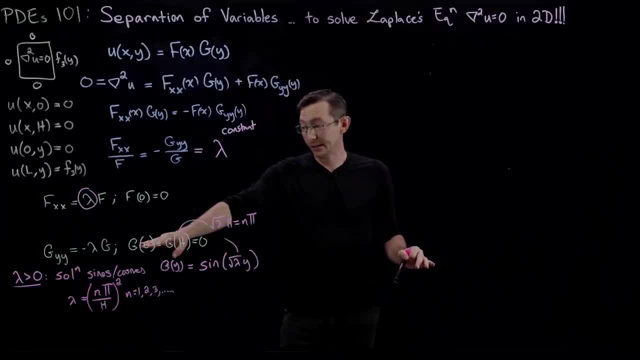 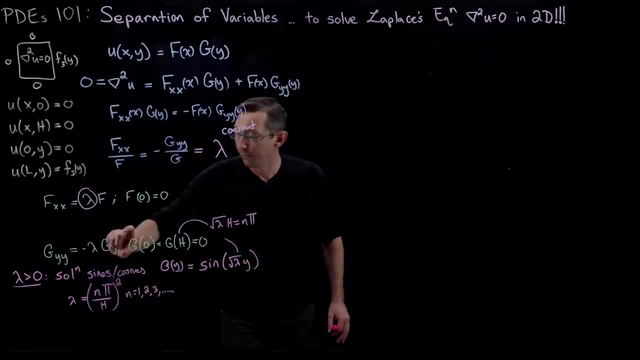 that's an integer. this is a valid lambda that satisfies these boundary conditions. And so now what I have is a countably infinite set of ordinary differential equations for f and for g, A countably infinite set For every n. I get a lambda and I have a corresponding. 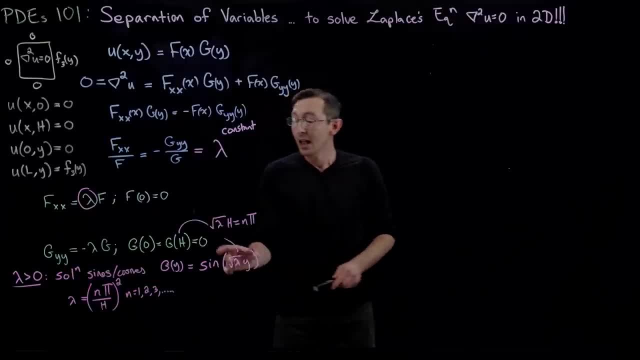 ordinary differential equation that satisfies my boundary conditions And the solution are signs with that fundamental frequency of root lambda in the vertical direction. Good, So I'm gonna write this out just very, very quickly, Very explicitly, so I don't forget. I'm gonna say maybe, probably should have color coded this. 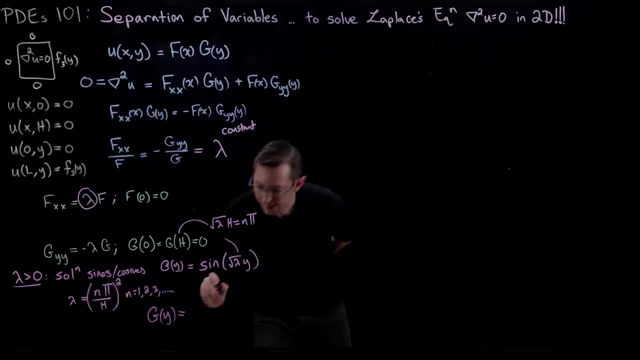 G of y equals sign of n pi over h y. So all of the functions g in this separation of variables that satisfy the top and bottom boundary conditions, all of them are of this form for an integer value of n. That's super cool. 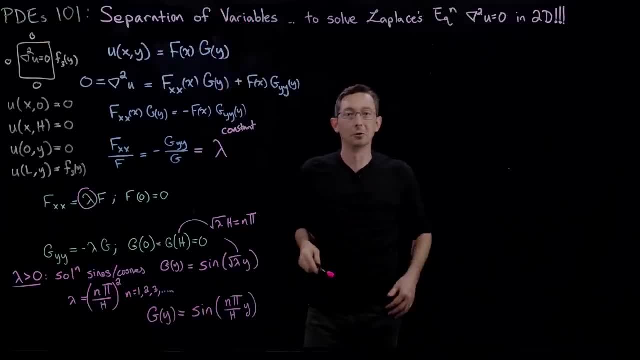 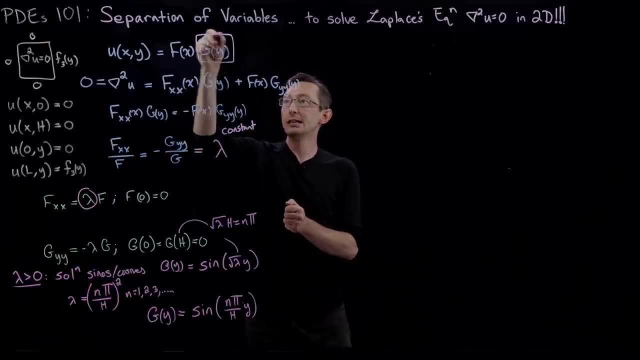 So we've solved half the problem. Check, okay, this video is gonna go long. We're half way through. we've solved half of the problem, Okay. so now we have- we know what these guys are. The g of y's are signs, with these perfect kind of harmonic. 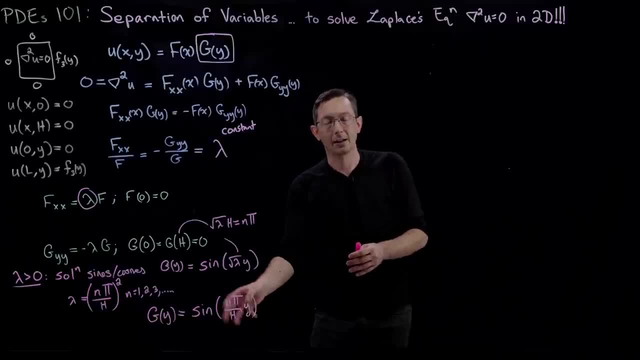 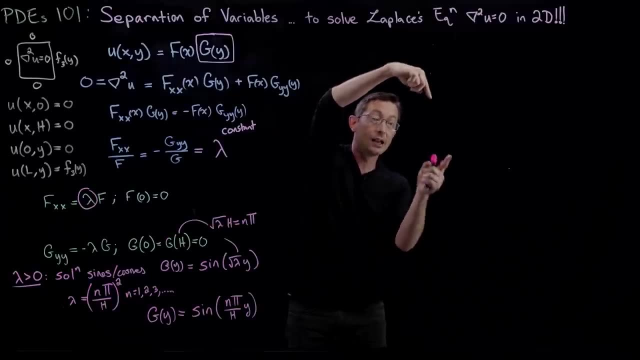 so if you think about a guitar string, these kind of harmonic eigenvalues that satisfy these boundary conditions, Actually very much like a guitar where you pin this in two places. There's only certain signs and cosines that can exist Okay And satisfy the top and bottom boundary conditions. 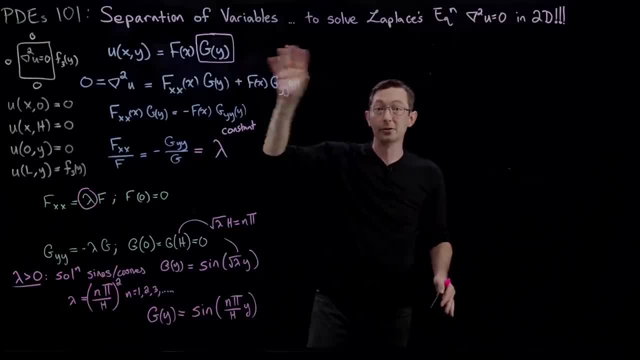 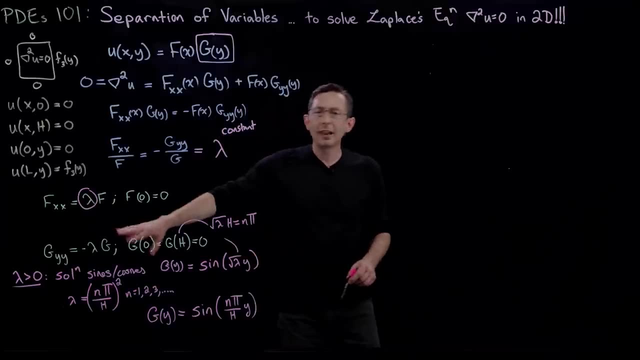 those pin boundary conditions. That's another application of separation of variables. I'll show you in another lecture soon One of my favorites, actually. Good, I'll let you think about what happens. So we already talked about when lambda equals zero. that's the same as when n equals zero. 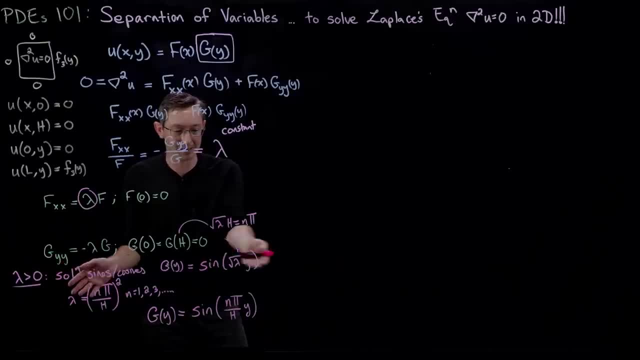 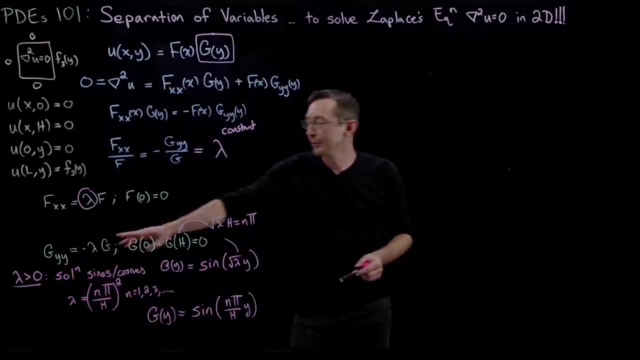 that's a perfectly valid, boring solution where this is the zero function. so that's not interesting. And if lambda is less than zero, this is a good homework problem. If lambda is less than zero, then this equation now will have solutions: e to the plus and minus square root of lambda y. 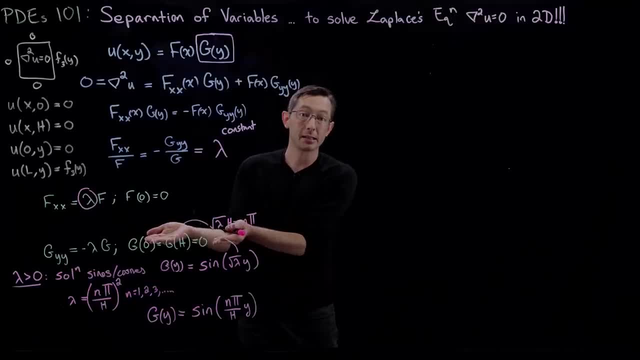 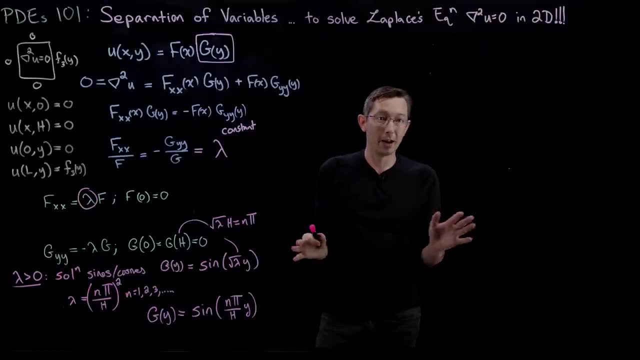 And there is no way of satisfying both of these boundary conditions equaling zero, with e to the root lambda y, plus e to the minus root lambda y. There's no way. with just exponential functions I can satisfy these two boundary conditions. So lambda has to be positive. 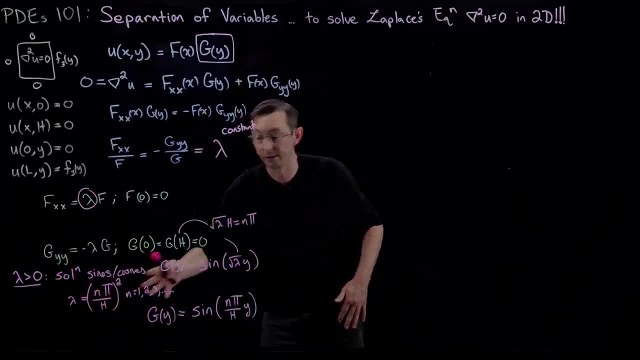 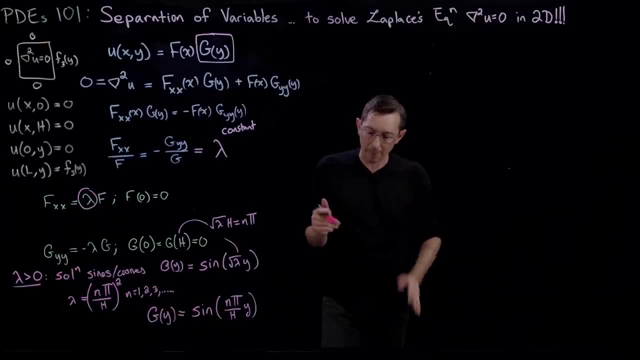 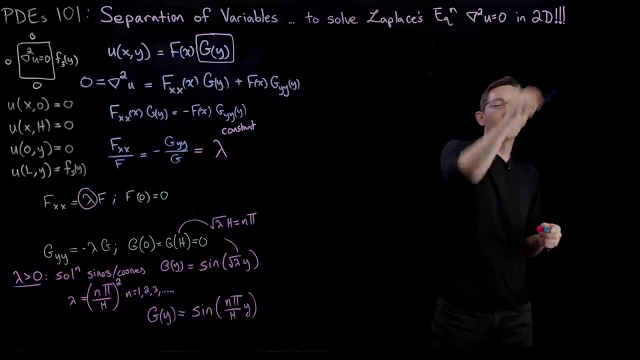 and it has to have this very special set of lambdas to be valid. Okay, so essentially, the big step one was that we- I'm gonna draw this out because I think this is actually really important and I have a little cartoon I draw in my class- 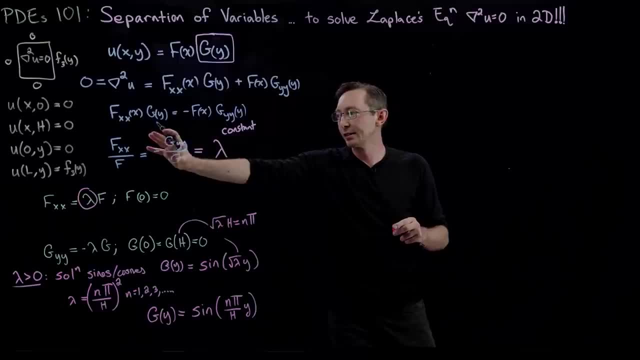 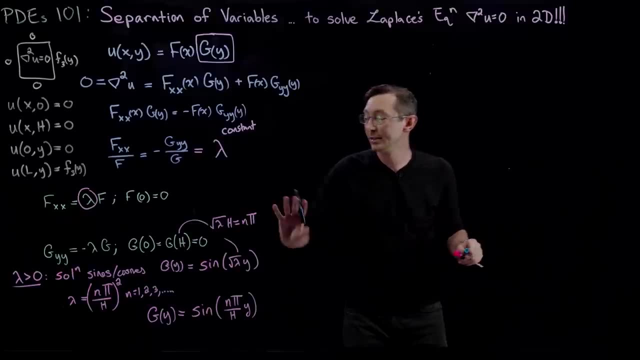 which is the first step after separation of variables and getting this system of ordinary differential equations, was we solved the one with easy boundary conditions? Always make your life easy. solve the easy boundary conditions first, the ones that are zero. okay, so in the y direction in this case. And what we did was we essentially we solved the one with easy boundary conditions first, the ones that are zero. okay, so in the y direction in this case. And what we did was we essentially we solved the one with easy boundary conditions first, the ones that are zero. okay, so in the y direction in this case. And what we did was we essentially 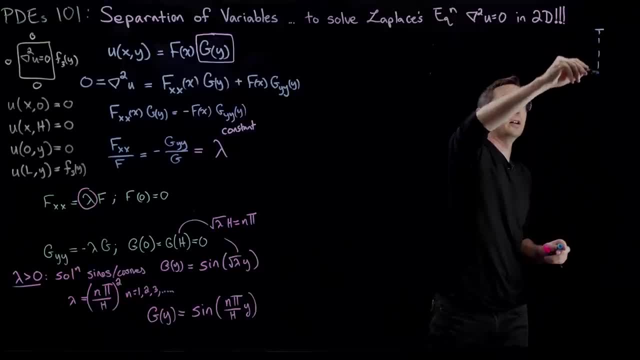 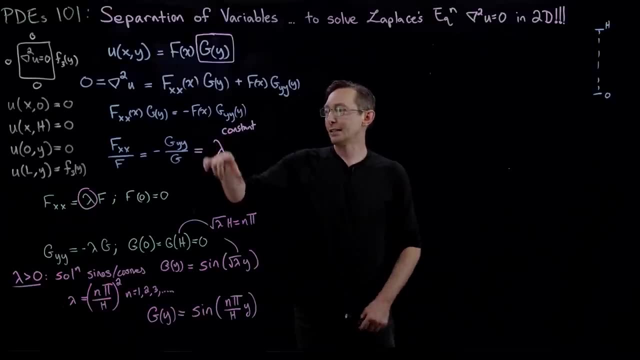 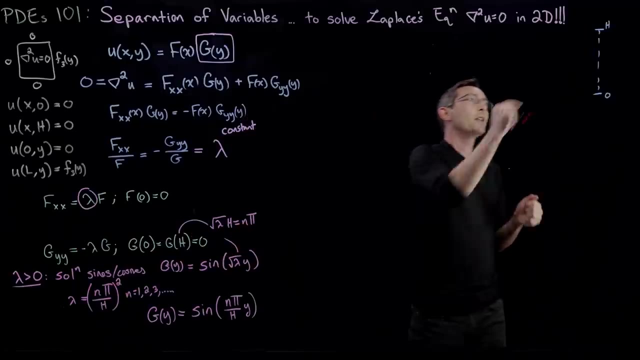 said that, in the y direction, from, let's say, zero to h, the only solutions that can satisfy this differential equation, with these boundary conditions that it has to be zero, at these conditions, are these very, very special sine waves that have the right. I'm not very good at drawing sine waves. 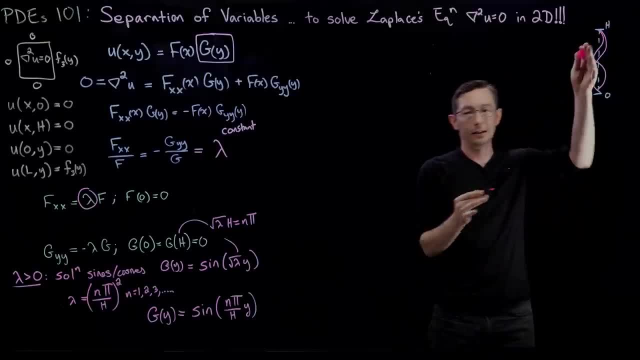 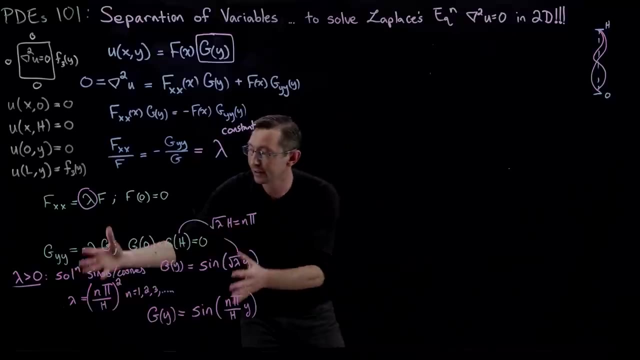 but very, very special sine waves that have the right frequency, so that they exactly are pinned to zero at the bottom and the top of my domain. So that's super cool. okay, And now the next step. the second step is that we're gonna use these lambdas. 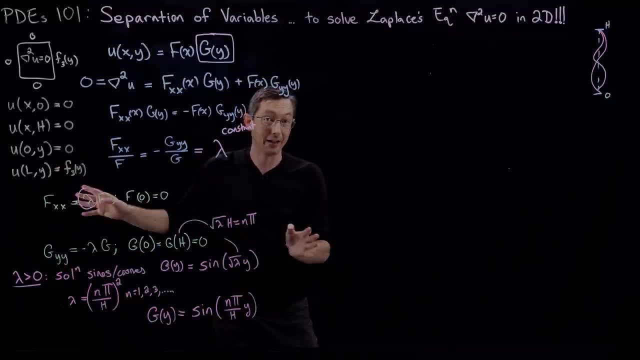 and we're gonna solve our hard ODE in f. okay, So now we're gonna solve our ODE in f and we're going to use the solutions of those. Eventually, we're gonna use our boundary conditions to get the coefficients of this function. 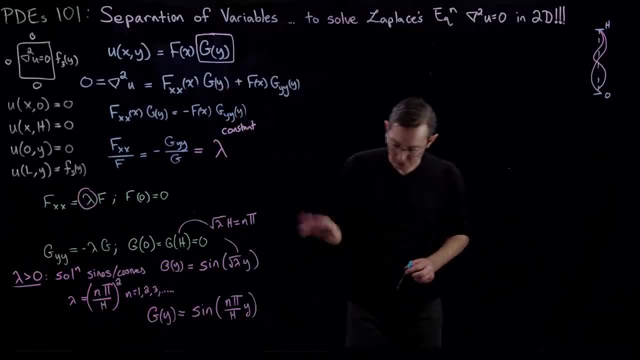 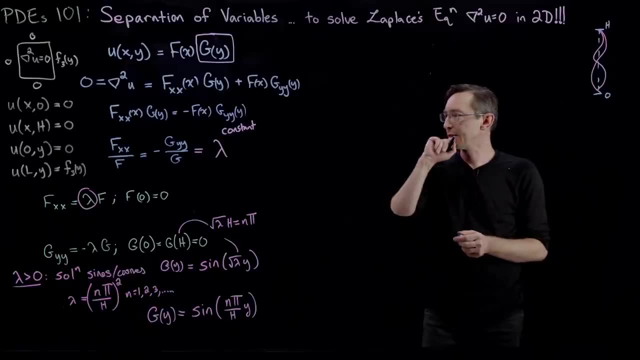 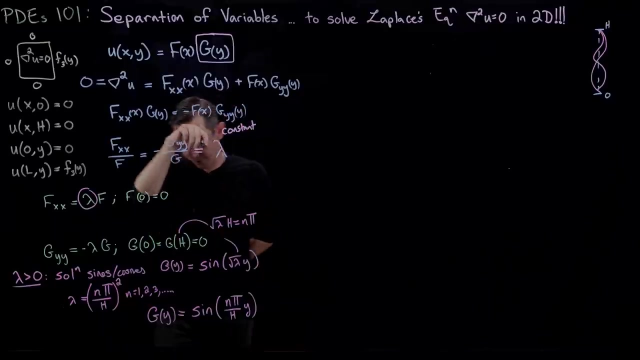 Okay, good, So that is what we're doing now. So we've just solved the y's, now we're going to solve the f's, And I think this actually is not that bad. So where do I wanna do this? Maybe I'll just cheat and use my notes. 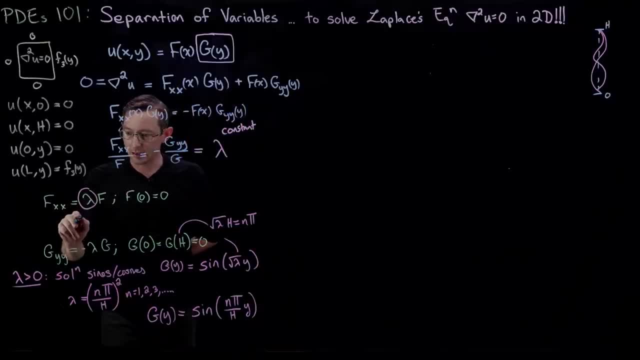 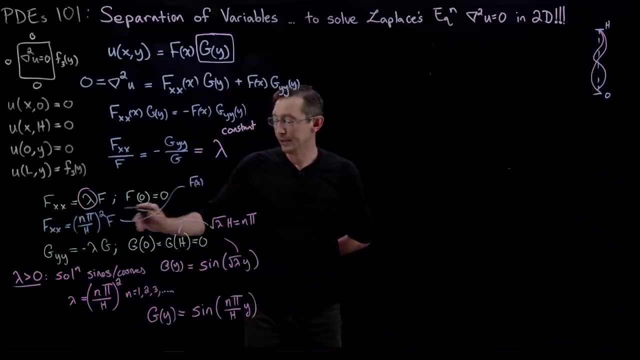 Okay, so we know that f x, x equals lambda, which is n pi over h, quantity squared of f. good, And we know that the solutions of this are going to be f of x. these are positive numbers here, and so we know that the solution of f, prime, prime. 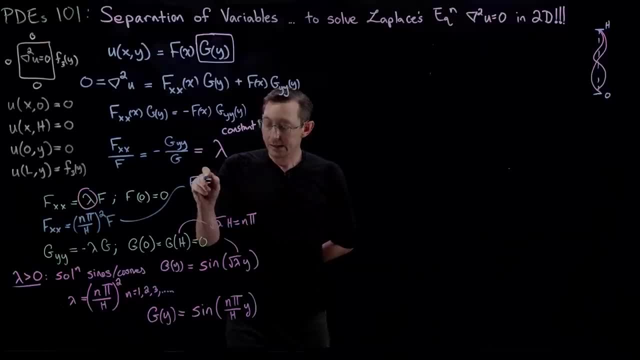 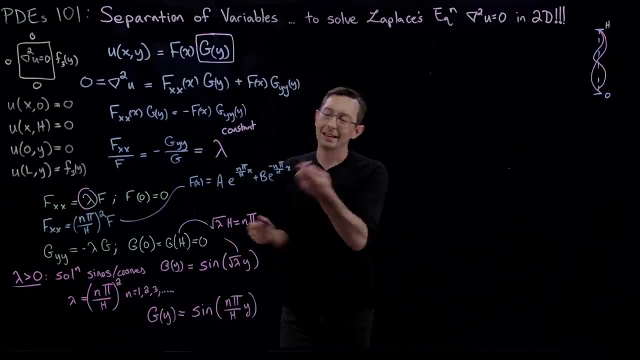 equals a positive number. f is going to be some constant a e to the n pi over h x, plus some other constant b e to the n pi, the minus n pi over h x, And technically for every. this is an ordinary differential equation. 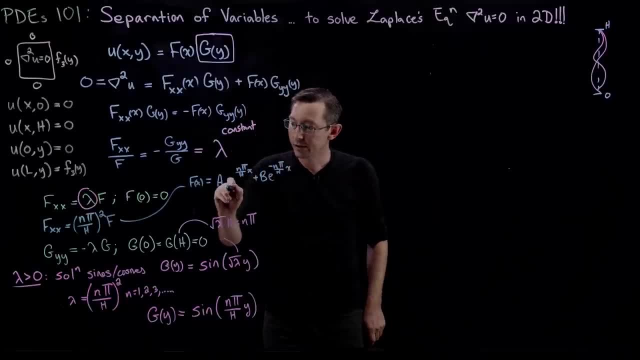 for every integer n. it's a whole separate differential equation. So these are possibly different coefficients: a one, a two, a three, a four for each of those values of n. So this is actually not that bad. I should have boxed this solution here. 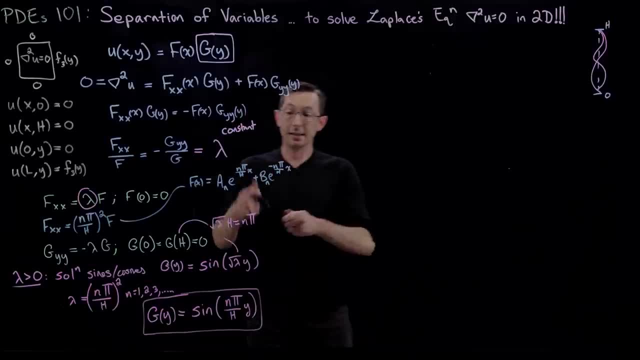 It corresponded to this solution here, And this is the solution of my x equation, now that I know that my eigenvalues have to be root n pi or, sorry, have to be n? pi over h squared. And here's where we get to use our easy x boundary condition. 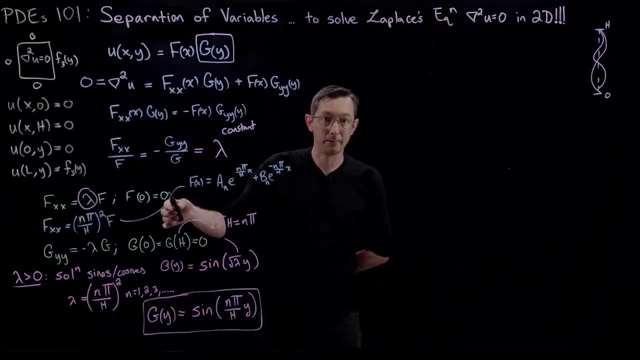 So our easy x boundary condition is that f of zero has to be zero. So I can plug zero into both of these equations and e to the zero is one, And so I get: f of zero equals a n plus b n equals zero. 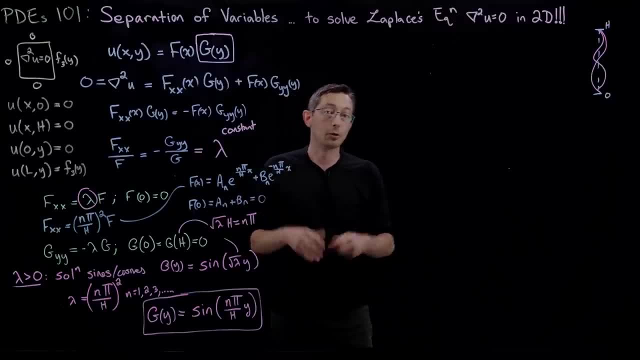 which means b n has to equal minus a n. Okay, so anytime I see a b n, I can just swap this out for a minus a n. I hope you caught what I did. I plugged in: x equals zero. That killed the exponentials, they just became ones. 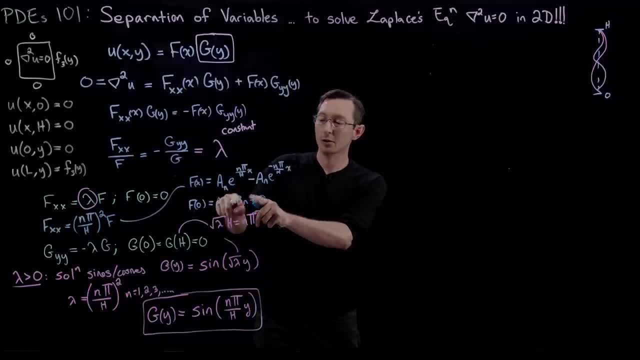 and I got a n plus b n has to equal zero, which means b? n equals minus a n. okay, And I'm getting a little out of space here, but essentially the sum of e to the plus alpha x, minus e to the minus alpha x. 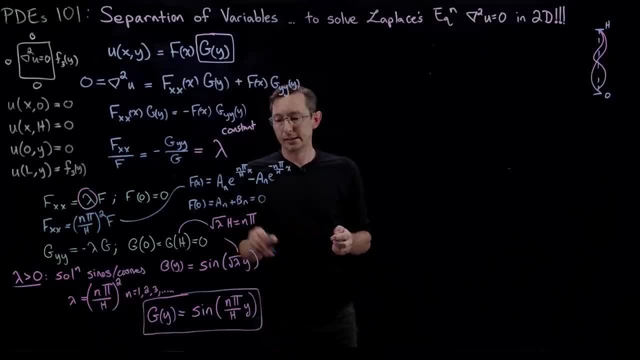 is just a hyperbolic sine function, And so this f of x, maybe I'll just write it down here. So my f of x is equal to a, n. it's actually equal to two, a, n, hyperbolic sine of n, pi over h, x. good, 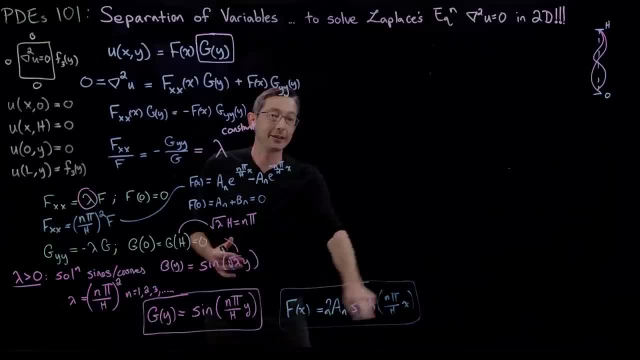 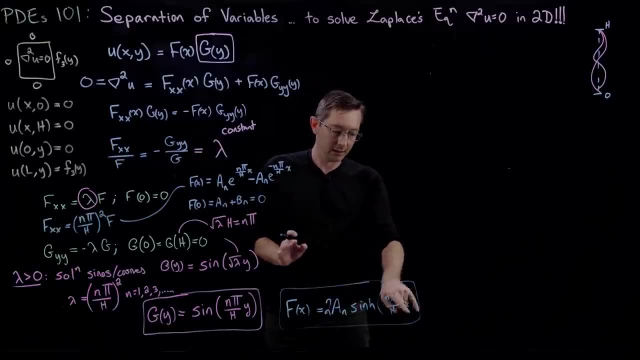 So all of my x solutions have to have this form. This is just a basic basic, like trig identity is that this equals two a n sinh of n pi over h x? You can just verify this yourself. it's pretty easy If you like complex analysis. 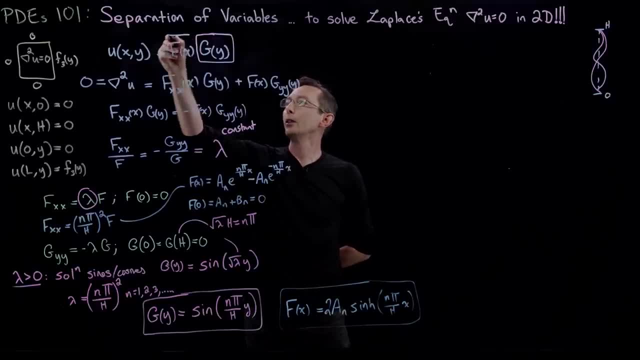 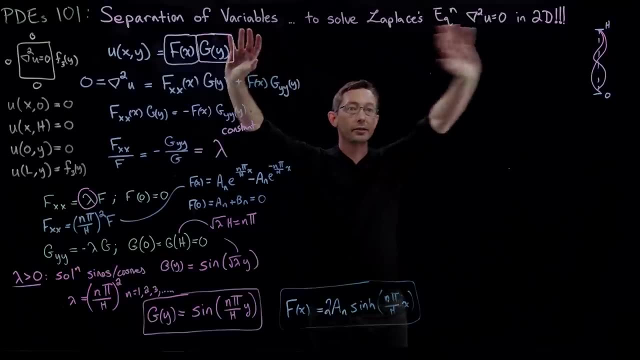 this is like a homework problem in complex, And so now we also have this term. Good, okay, so I'm just gonna barrel through, I'm gonna go all the way to the end and I'm gonna write out the whole solution. 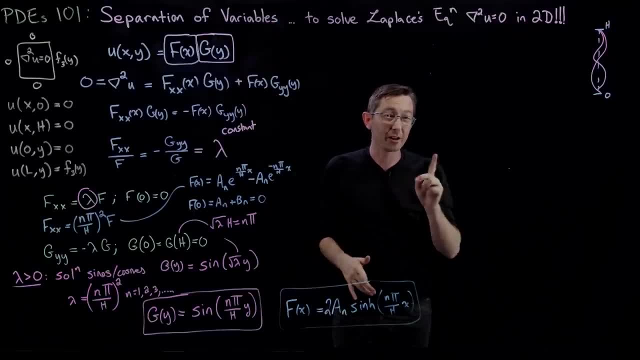 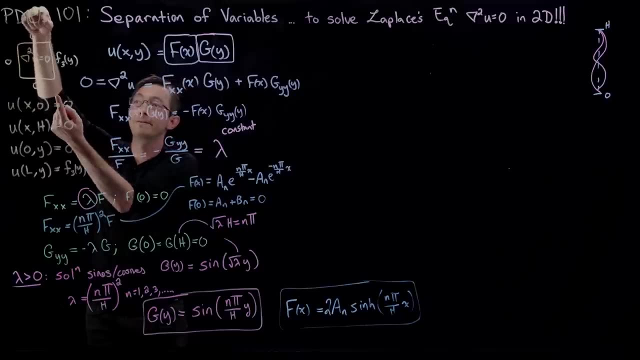 And then we're going to recap what we learned and we're also gonna think about, like, what happened if I had different boundary conditions- Maybe I'll talk about that a little bit- If I had different boundary conditions here these were fixed temperature. 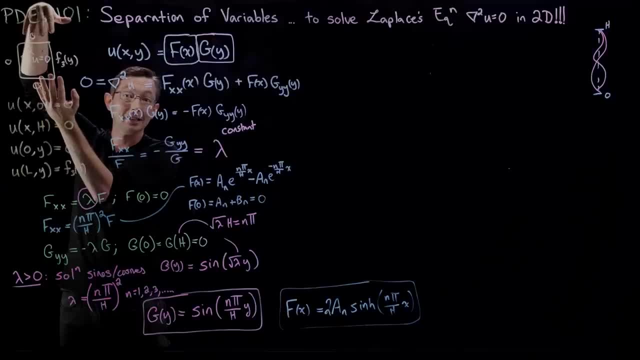 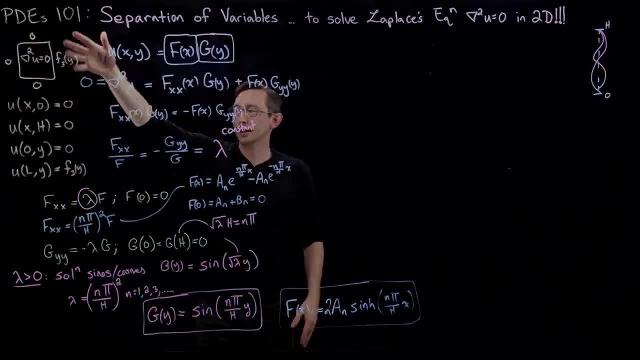 I basically have these sides, let's say, in an ice water bath so that they're fixed to be temperature zero. Same on the left side, And maybe I hit the right hand side with a blow torch to give it some constant thermal profile. 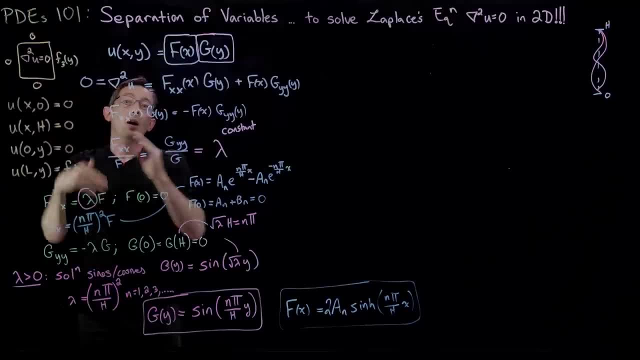 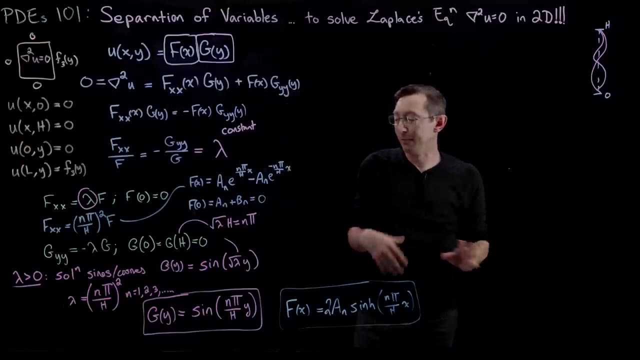 But so these are fixed temperature. u equals zero. What if we had a no flux condition? What if we had an insulating boundary condition? The partial derivative of u sub x equals zero. or the partial derivative of u sub y equals zero. I'll talk you through this in a little bit. 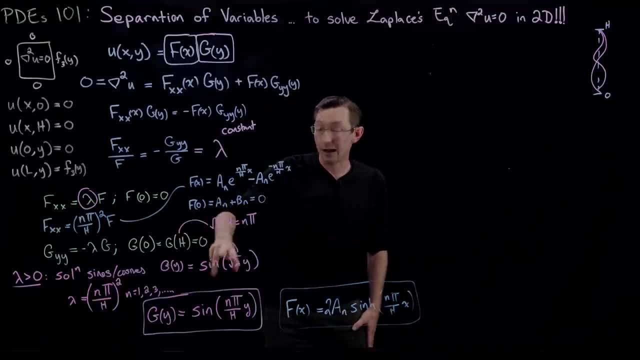 but essentially what would happen is we would get slightly different boundary conditions here. Maybe we would get g sub y of zero equals g sub y of h equals zero, in which case I would get cosine solutions being the only ones that can satisfy that zero flux condition. 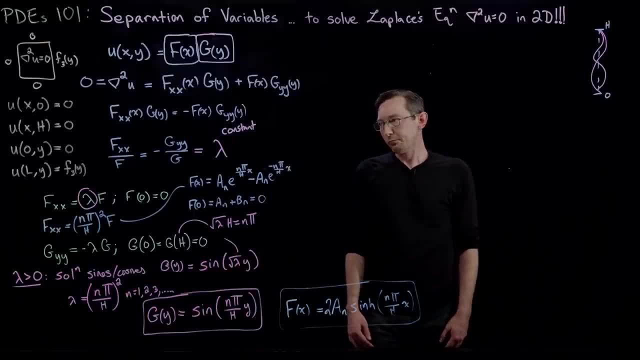 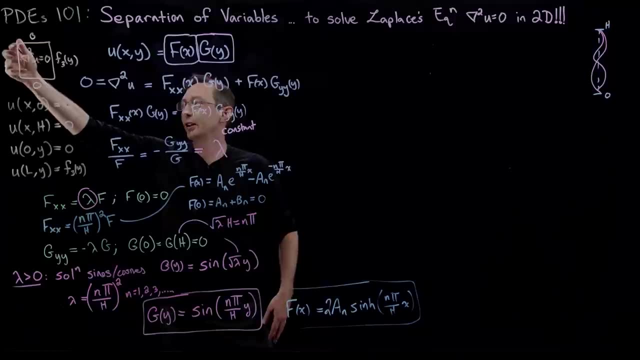 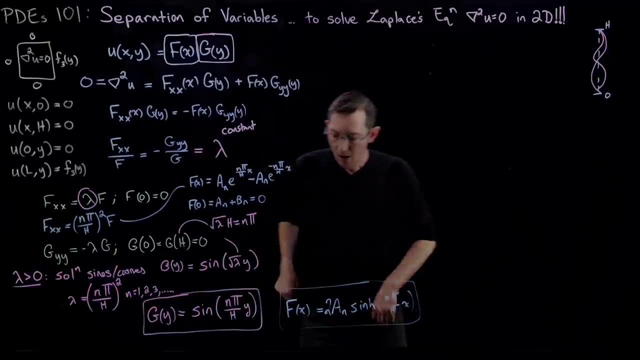 And these would all become cosines. Other things you could do here. I think if I had an insulating boundary condition on the left then I would probably get coshes here, hyperbolic cosines, I don't quite remember. You should work through this yourself, okay. 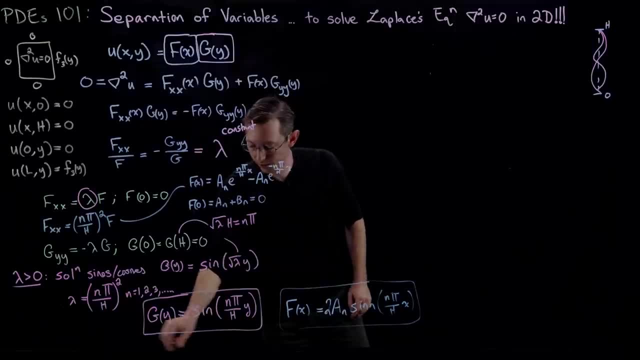 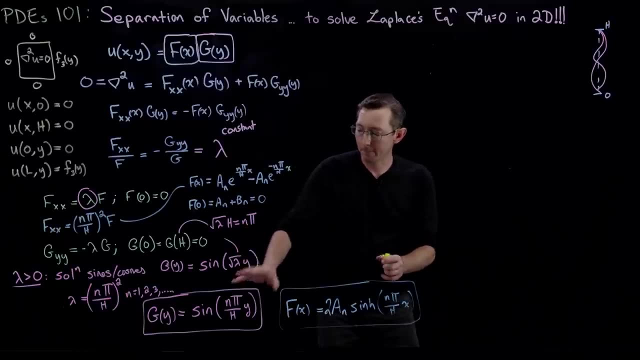 But so now what we have is that the solution of this partial differential equation in u is equal to- and remember this will have. this is true for every single integer: n for n equals zero, one, two, three, four and so on. 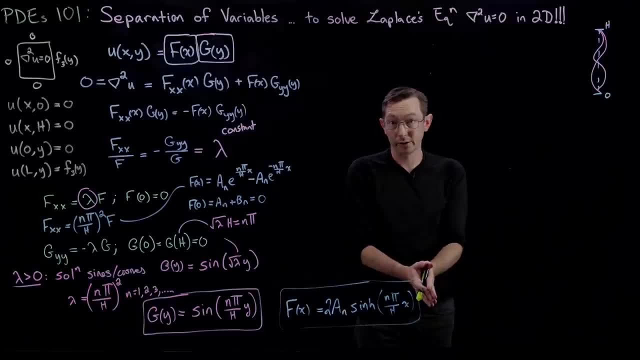 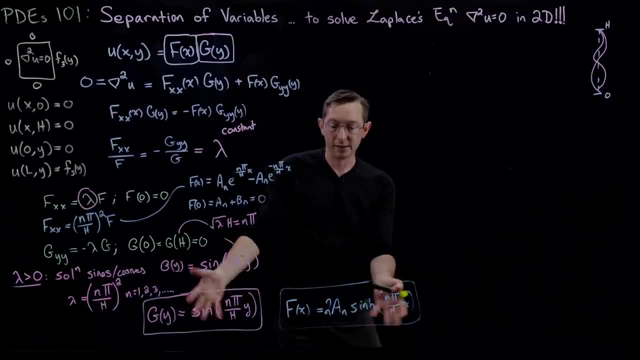 And so, because it's true for all of those, if I add up all of those solutions, that's the solution of u. Every single lambda here, I get one of these solutions, And if I add them all up, that's my global solution to u. 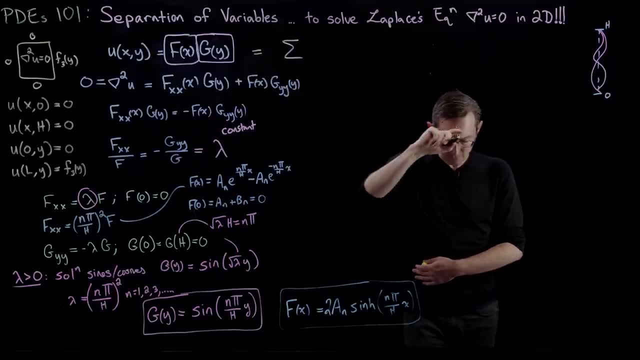 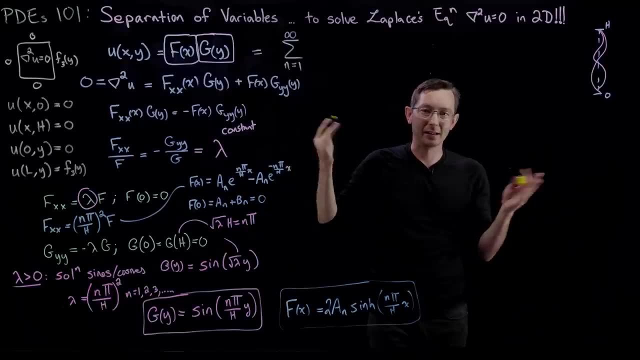 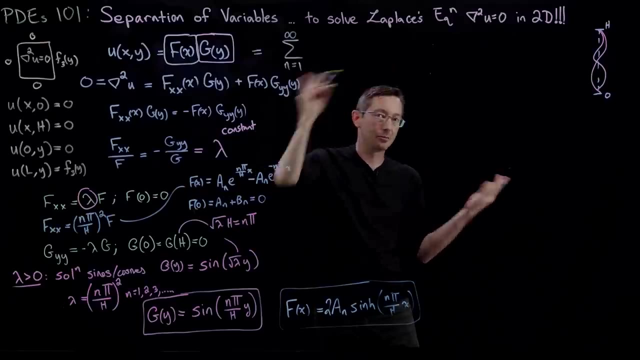 So this is equal to the sum from n equals one to infinity. And the reason I'm not doing n equals zero is because it's boring, because sine of zero is always zero. So you could do n equals zero and write this out, but the first term would be zero. 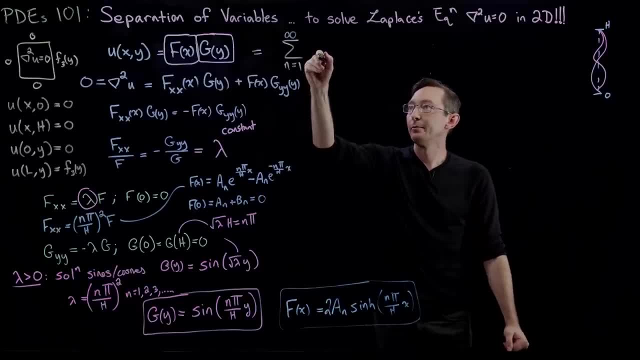 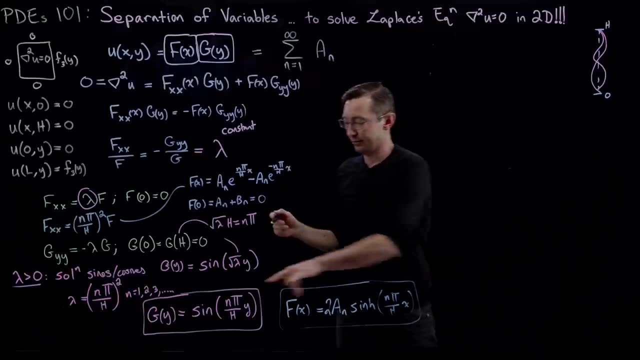 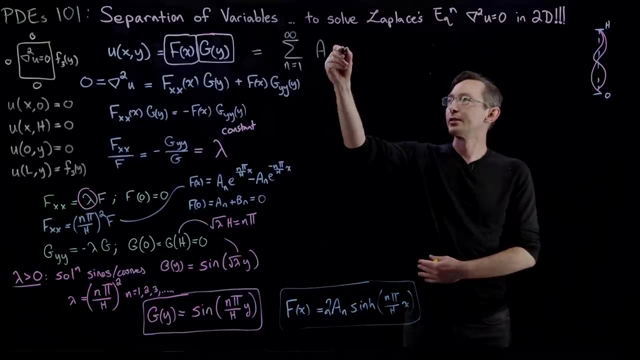 And we have. I'm actually gonna write my f of x's first, So I have my a sub n times, times, what times? let's say, I could do a of n sinh or a of n sine. I'm just gonna do my sine first. 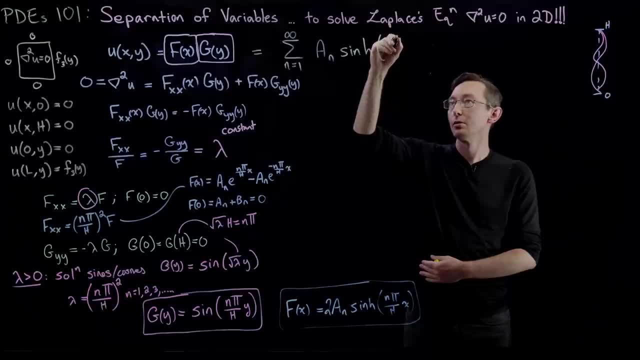 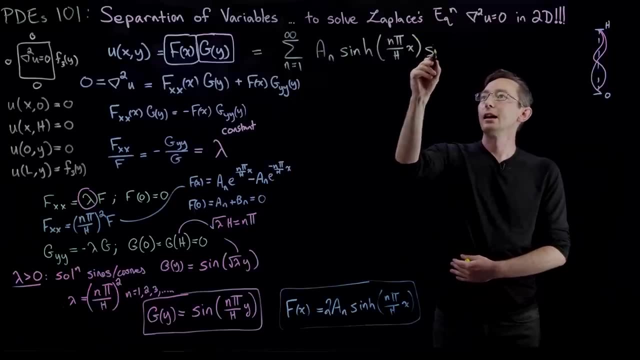 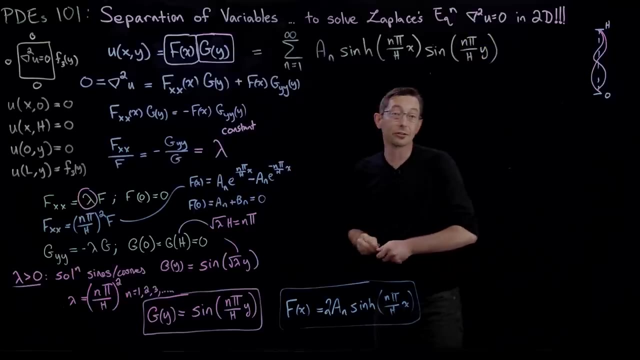 maybe my sinh first of n pi over h. this is in the x direction times. sine of n pi over h in the y direction. So it actually doesn't look that terrible. I get sinhs in the x direction and I get sines in the y direction. 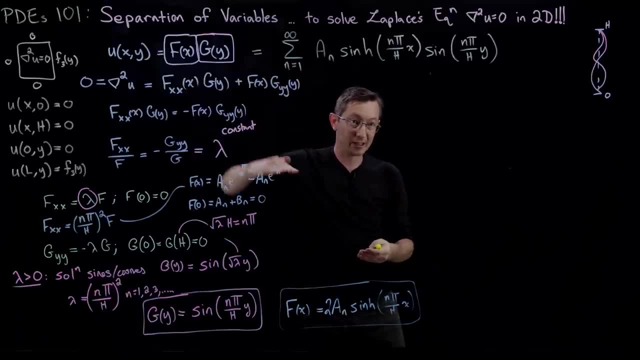 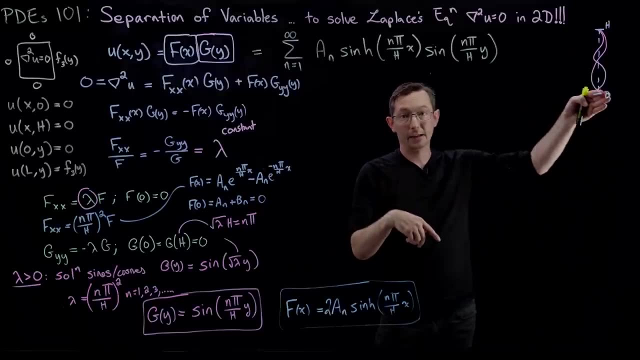 Okay, and sinhs, you know it's gonna look like a decaying exponential plus a growing exponential, so something kind of- you know, almost catenary-ish. And these are harmonic to satisfy those boundary conditions in y. And I've gotten rid of this two here because I am lazy. 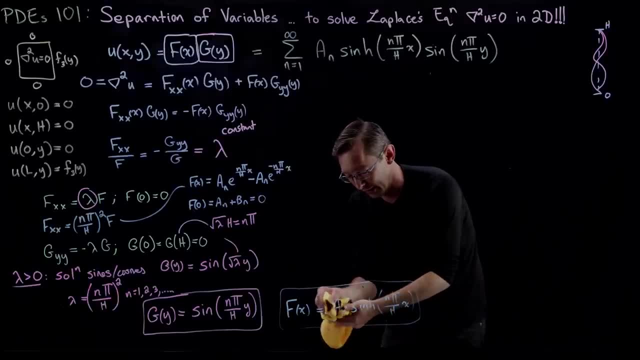 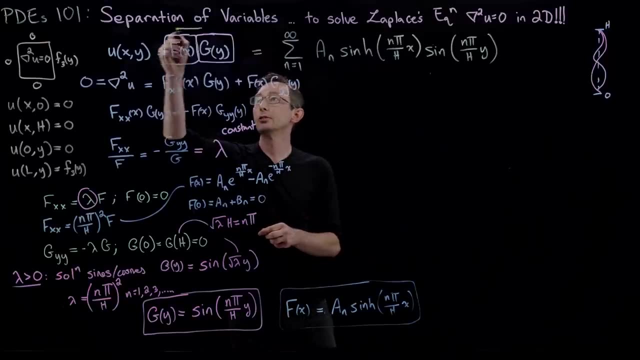 and because this is an undetermined equation, This is an undetermined constant, so I can just say that I am defining a to have that factor of two in there. This is the solution. So this is the actual solution of Laplace's equation. 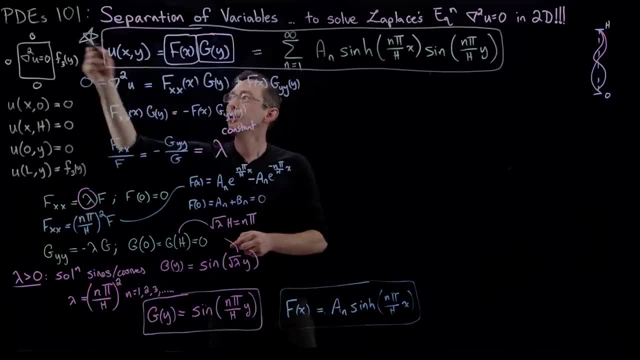 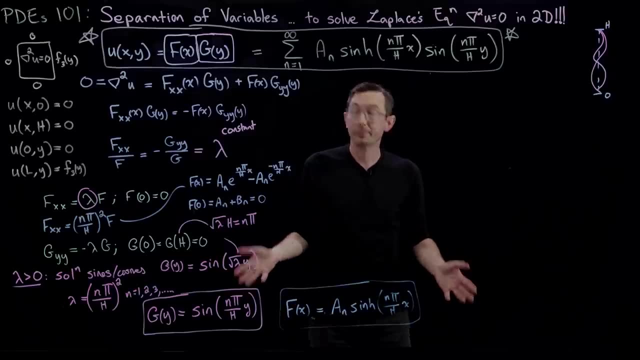 Okay, actual solution of Laplace's equation using separation of variables. Now, separation of variables does not always work. There are problems that are non-separable- Okay. there are problems where you can't separate the solution into a product of functions in x times. 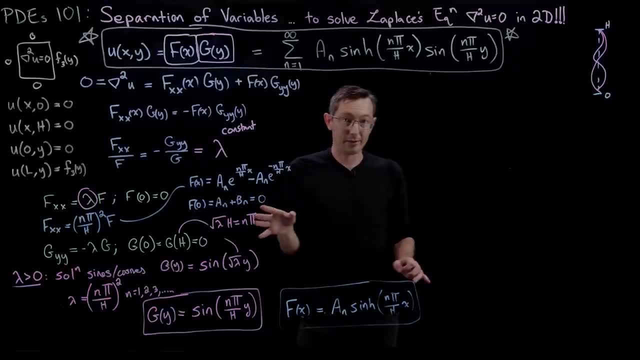 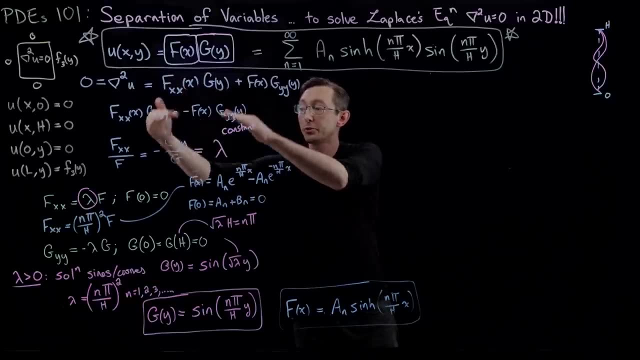 as a product of functions in y Plenty of examples of that. But when you so, what I would recommend is, if you think your problem is separable, you make this assumption, you go through the steps and if, at some point, you box yourself into a corner, 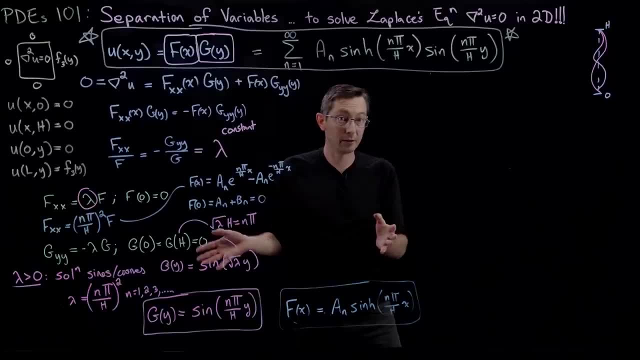 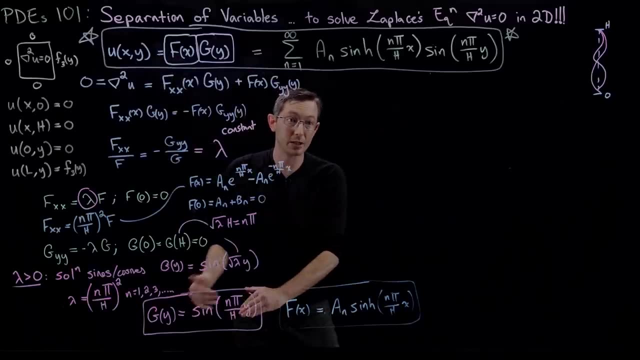 where you can't satisfy your boundary conditions or your initial data or whatever, then you might conclude the separation of variables doesn't work. But in this case we didn't hit any walls through this procedure and we actually were able to derive this full solution piece. 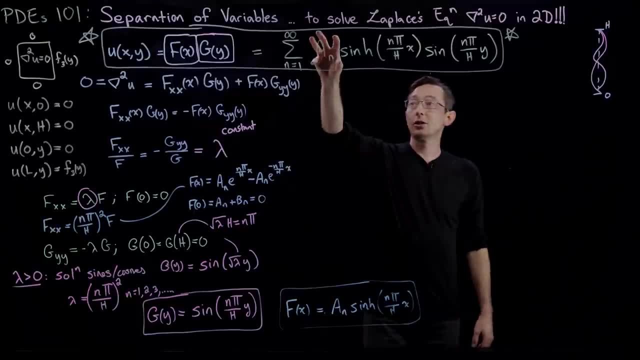 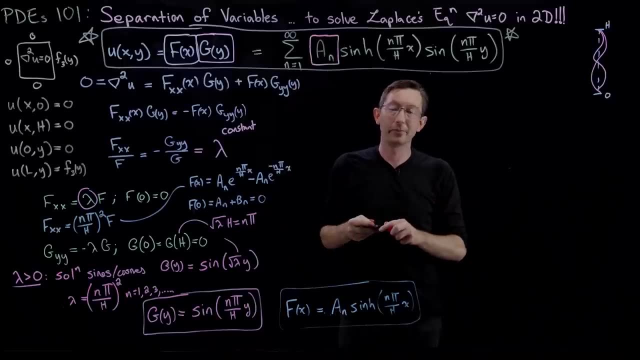 So let's go back to the CDE here. Okay, so I did not determine these coefficients a? n yet. This is kind of a pain in the butt. I will do this in a minute. These a n, these undetermined coefficients a n. 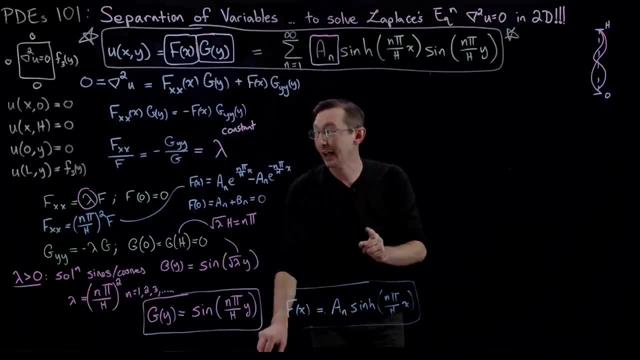 these are super important. There is one boundary condition I haven't used yet, and that is this one. So, if you think about all of the steps we've done up until now, we've used the bottom and top boundary conditions to solve my functions. 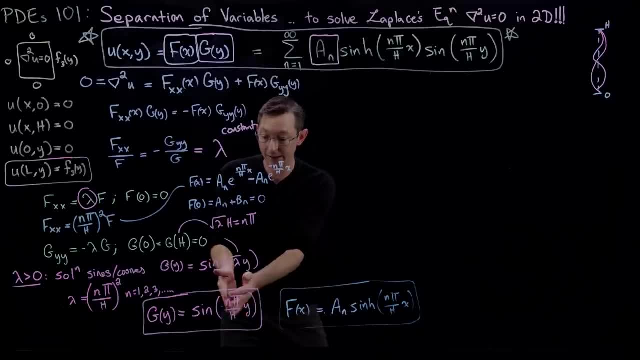 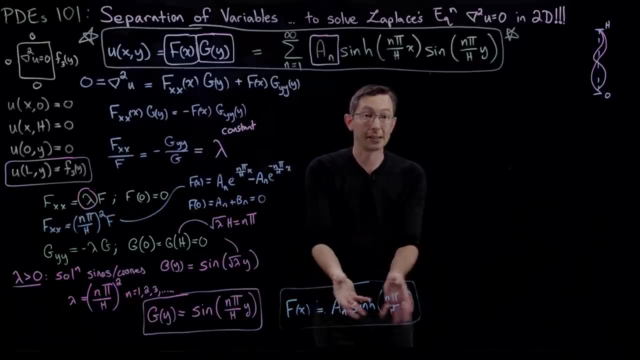 in y to get these perfect eigenvalues and these eigenfunctions in the y direction. We have used the left boundary condition for our f-equations to show that b has to equal minus a, which gave us cinches that gave us the form of this equation. but these coefficients, a, n, 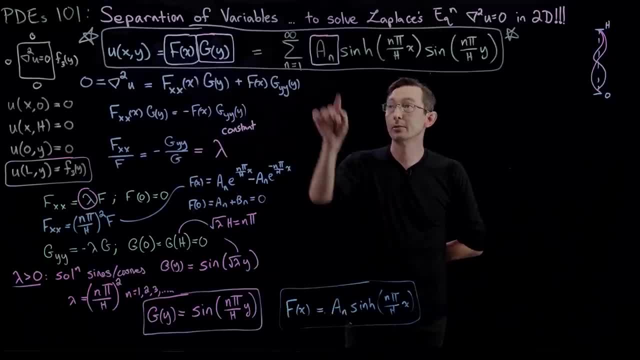 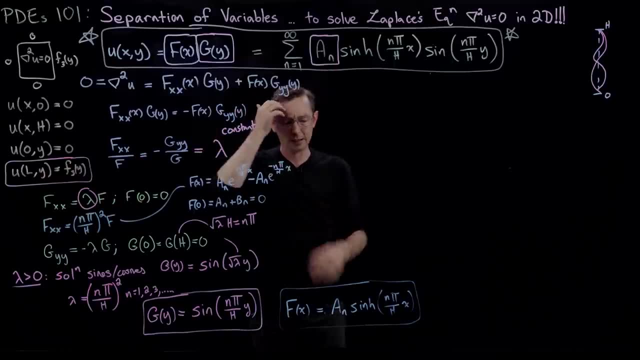 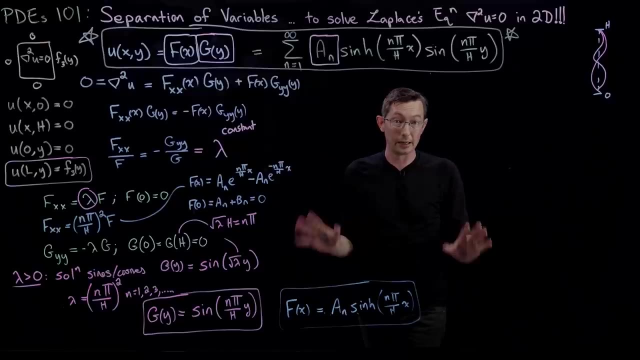 we haven't determined what these are yet, And the only information left to determine these coefficients are these: this kind of nasty boundary condition on the right. Okay, so I'm going to do that in a minute, But what I want to do right now is I just want to do a big recap. 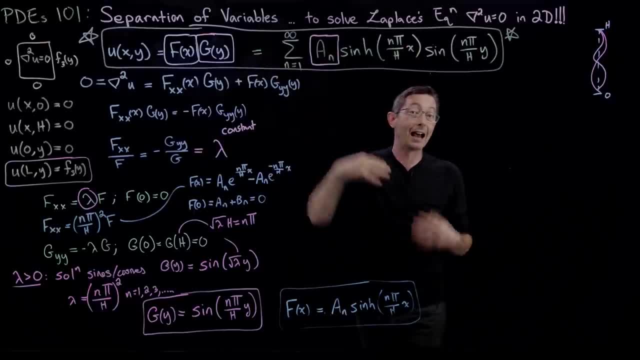 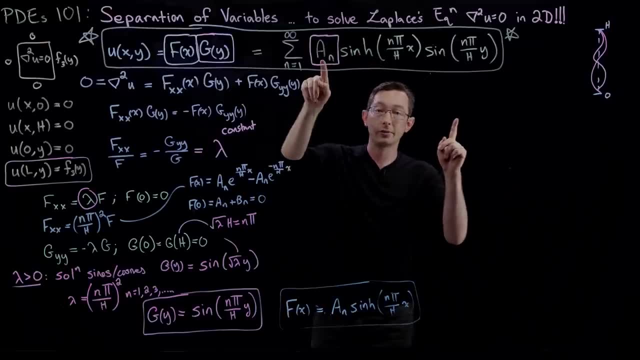 Okay, because some of you might not want to pay attention to this. you know deriving a n. I think it's amazing because this is going to basically use the Fourier transform. If you think about it, these coefficients are going to be the Fourier transform coefficients. 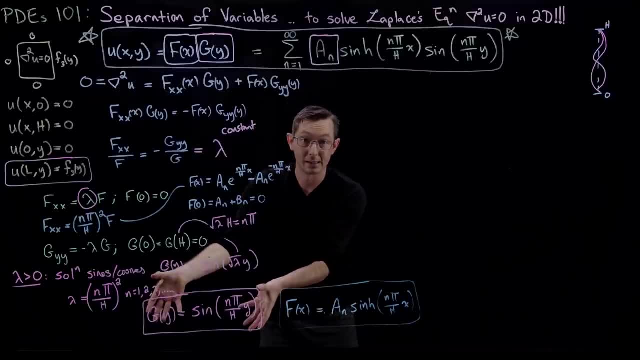 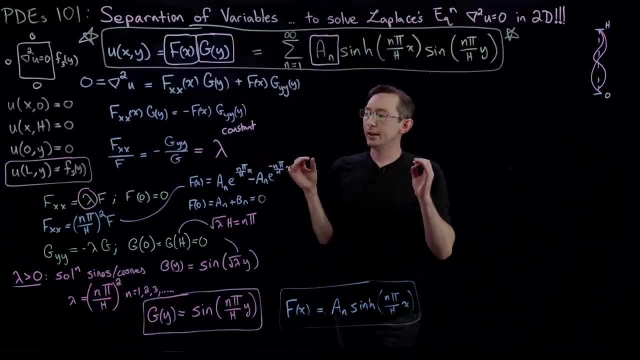 of this function, f3 in this basis of signs. So it's absolutely amazing connection to Fourier analysis. So the recap here for me is the most important part. We have introduced one of the most powerful methods of solving partial differential equations, which is separation of variables. 1690 Bernoulli. 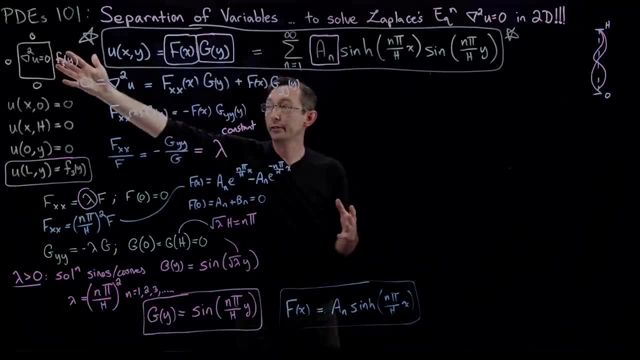 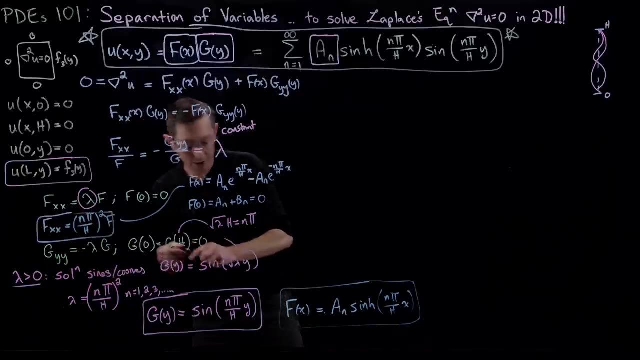 And essentially it allows us to transform our partial differential equation. You make this assumption, You plug it into your partial differential And you get out two systems of ordinary differential equations. You get a set of ordinary differential equations in x And you get a system of ordinary differential equations in y. 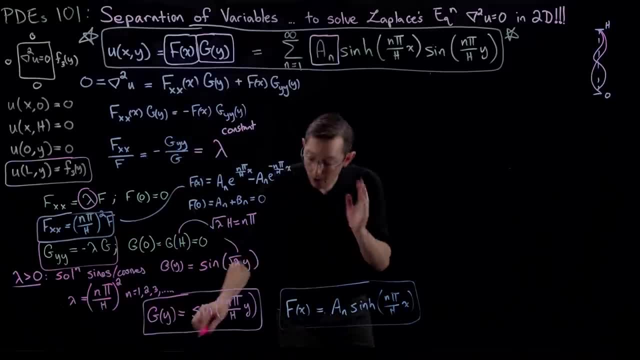 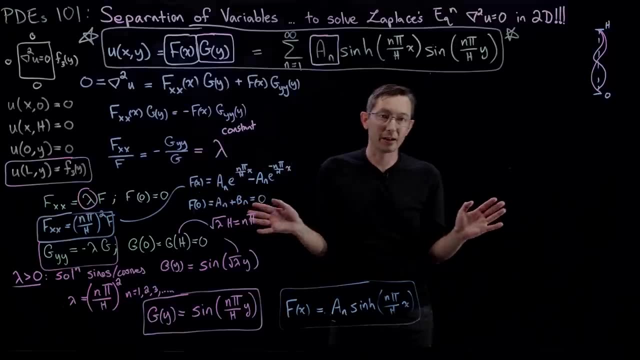 Where are my y's In y? And we know how to solve ordinary differential equations. They're relatively easy, especially linear ODEs that are second order. All of our solutions are going to be exponentials or sines and cosines. 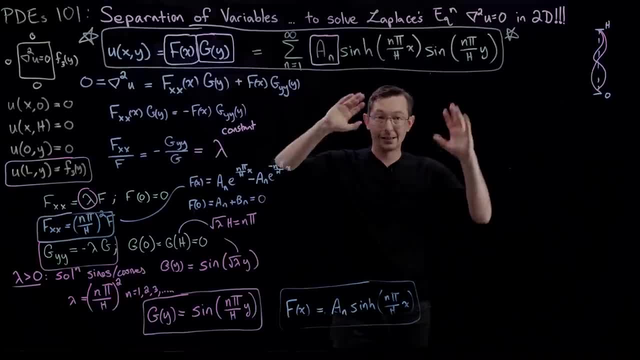 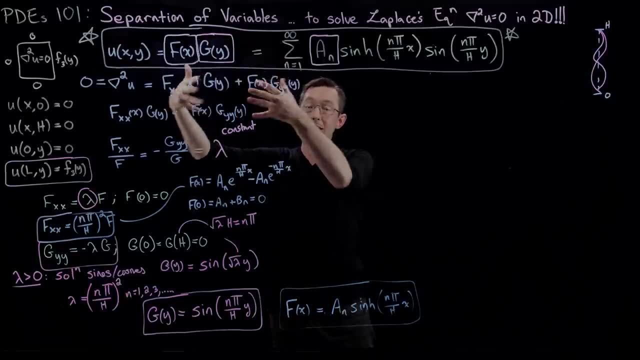 That's it, Okay, And so That's. you know that's big. step one is, you know, step zero is: assume you can split your variables. Step one is: plug it into your PDE and derive a system of ODEs out. 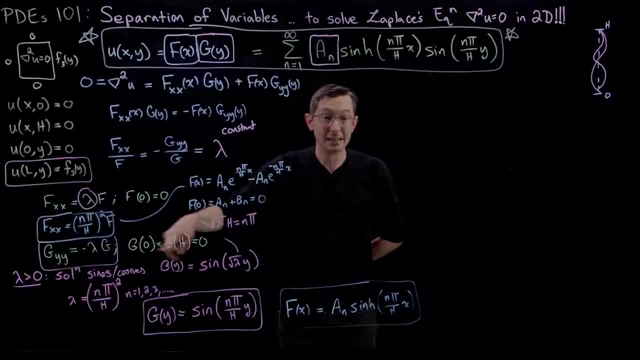 The next step, step two, is pick the one that has easy boundary conditions, not the one that has hard boundary conditions, the easy one- And find the special values of lambda, the special constants lambda that allow you to satisfy those boundary conditions. 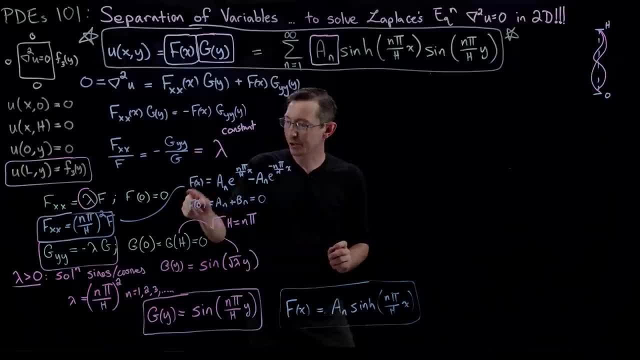 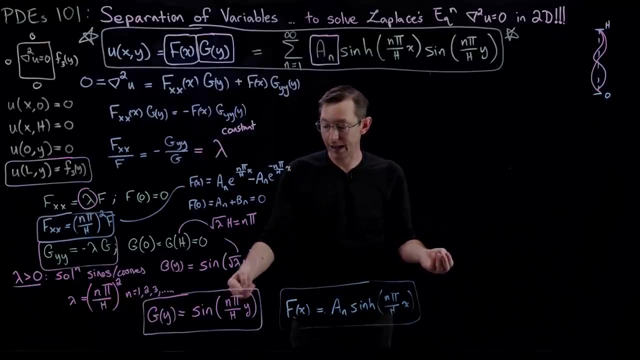 And for me this is one of the most beautiful parts- is that those special lambdas are actually eigenvalues. They are honest-to-goodness eigenvalues of this ordinary differential equation that satisfy these boundary conditions. So we have eigenvalues, lambda, which are these. you know, n pi over h squared for integer n. 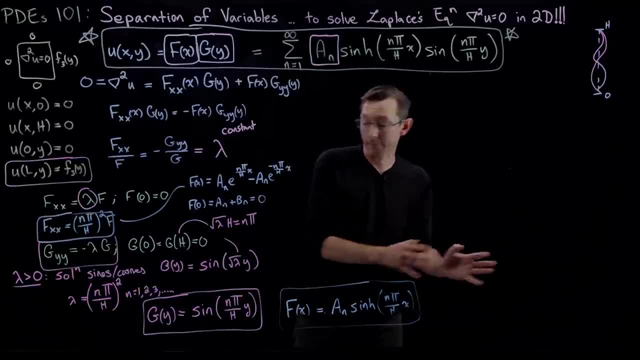 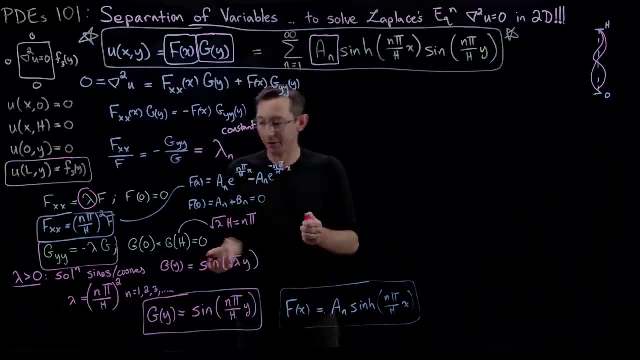 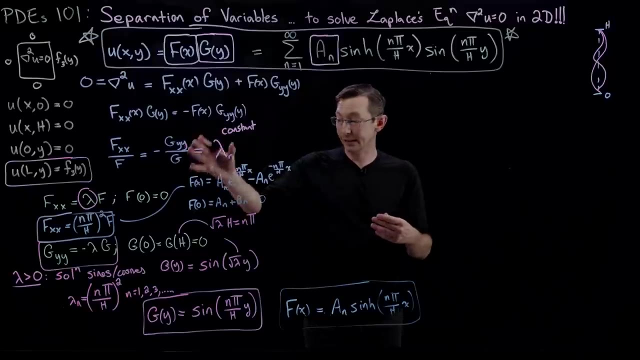 And the corresponding eigenfunction. So these are the eigenfunctions corresponding to those eigenvalues lambda. I'm actually going to write down Lambda n. Okay, these are all. these are my lambda n's. I have countably many eigenvalues lambda that satisfy these boundary conditions. 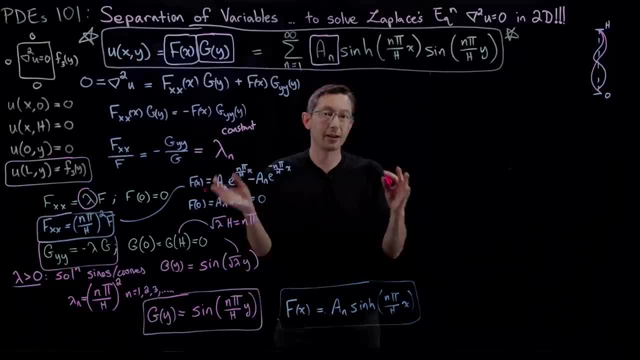 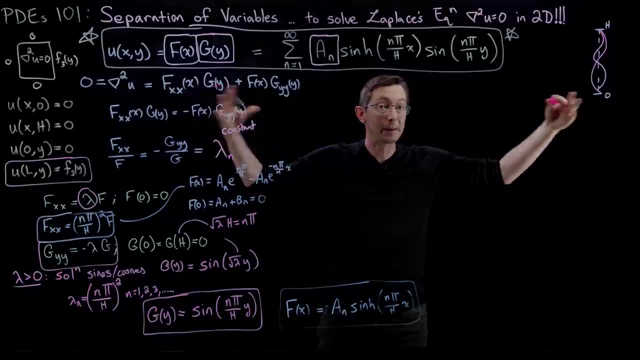 And corresponding, I have eigenfunctions. Okay, so I used to have eigenvalues and eigenvectors, But now we have eigenfunctions because the solutions are functions. We live in a function space, a Hilbert space. If you want to learn more about that, check out my Fourier analysis series. 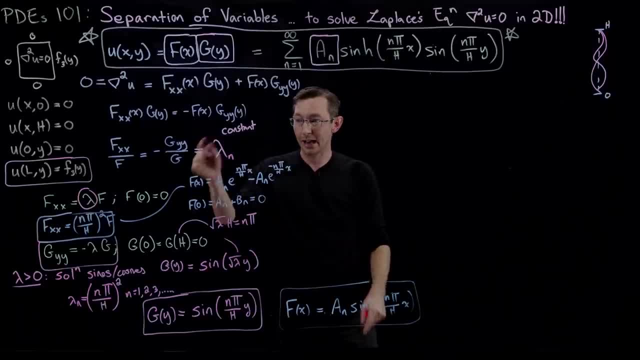 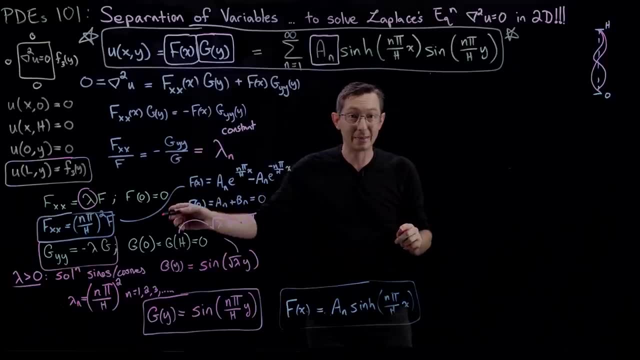 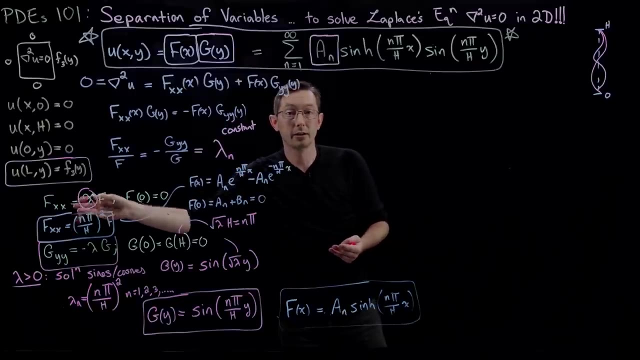 We talk all about, you know, Fourier, transforms and these eigenvalues and eigenfunctions. Okay, that was step two. I'm losing track here. I think that was step two. solve the one with the easy boundary conditions. Step three is now that we have determined those special lambdas, plug those into our hard, our differential equation with hard boundary conditions. 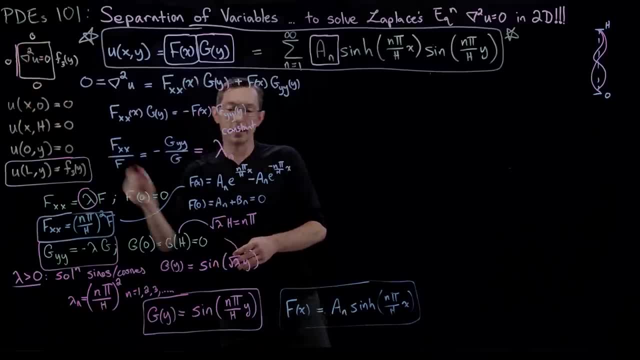 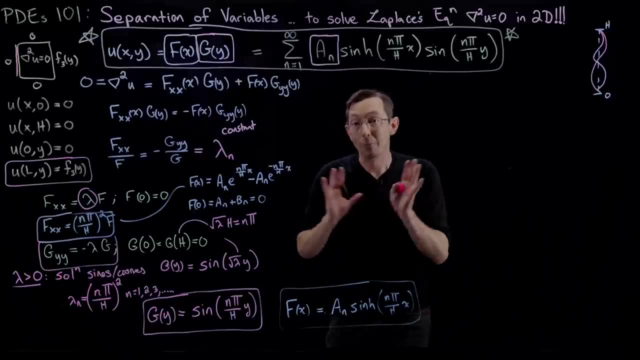 And one of the boundary conditions was easy- this one here. So I use that to figure out that Bn has to equal minus An. That tells me that I get cinches out And I am almost done. That's like three steps within a second. 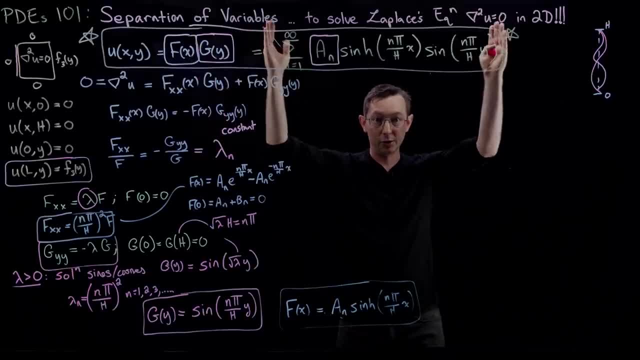 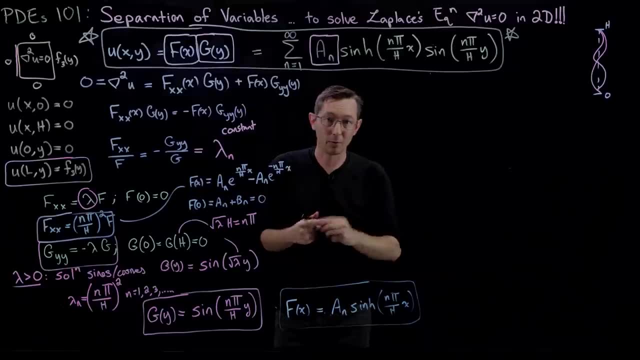 Okay, With a zeroth step and we get this solution here And the only thing we haven't done is solve for this An, And I'll just remind you, you know this is a homework problem. I hope you all do it. 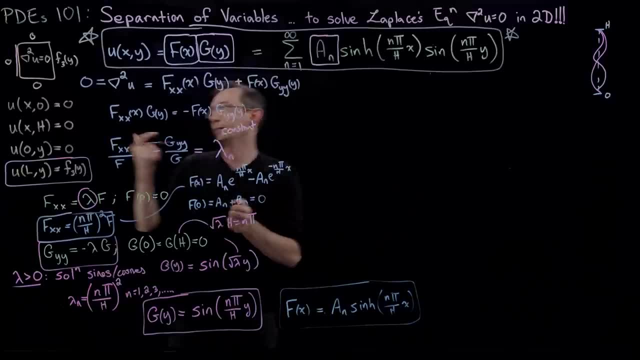 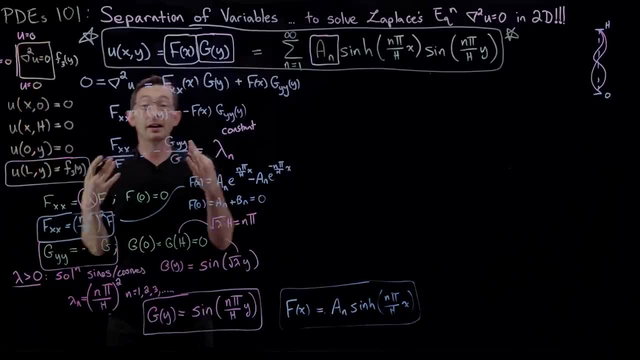 Maybe I'll do a little follow-up video of some of the other ways we can perturb the system. But this was for u equals zero and u equals zero and u equals zero. It's very interesting to try out what happens if the- you know partial derivative in y equals zero. 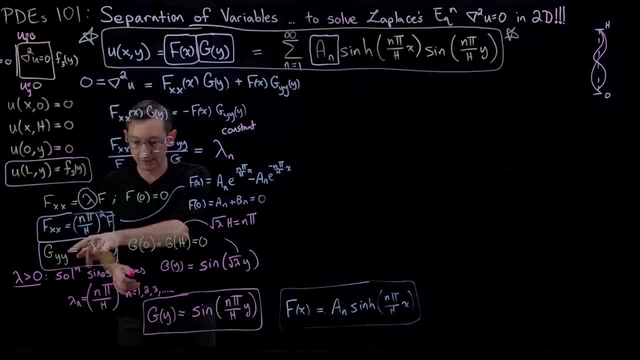 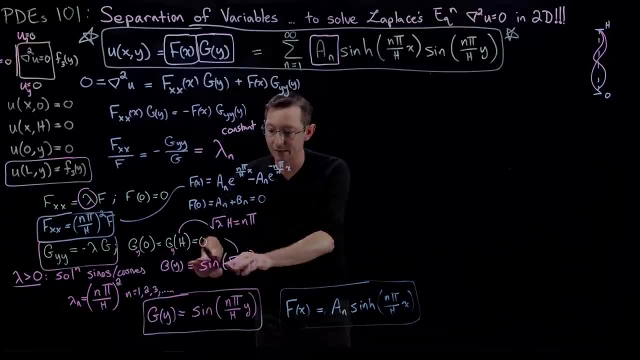 What if I have insulating boundary conditions? That changes these to gy, you know, sub y of zero and h equals zero, And that would change this to being so that only the cosine solutions can have their first derivative be zero on these. 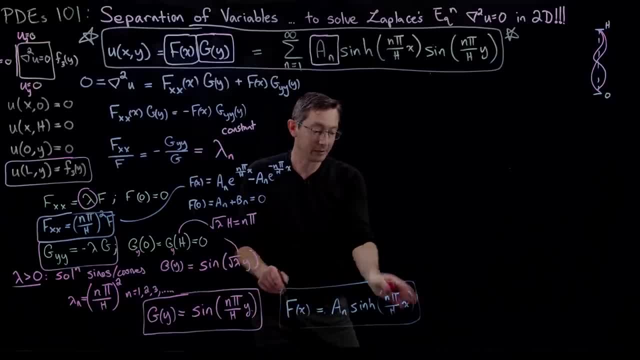 And so I would get cosine solutions here. same fundamental eigenvalues, same cinches here, But my gy's would now be cosine functions. if I had insulating top and bottom, if I put styrofoam on the top and bottom of this. 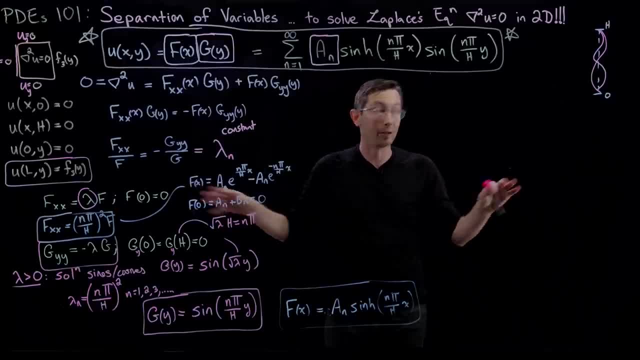 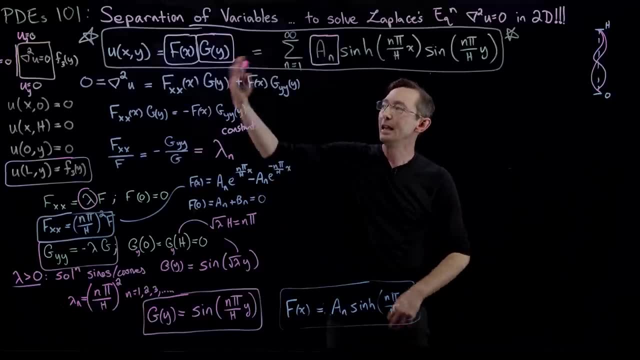 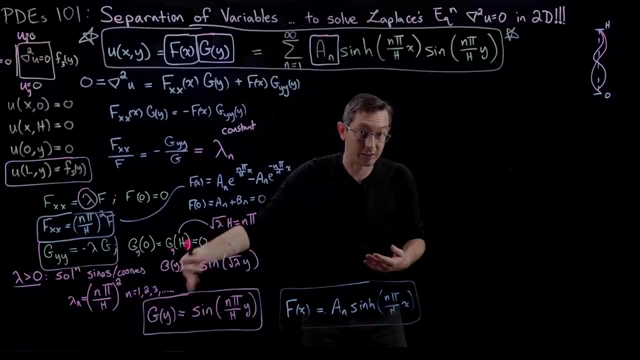 So really cool things. Once you know how this works, you can pretty much solve All of these problems. You could solve this on a circle on a disk. You could solve this on you know a ring. You could solve this on lots of different geometries. if you know this kind of basic procedure of you know split, plug it in. solve your differential equations. solve the easy one first, find your eigenvalues. plug it into the blue equation. 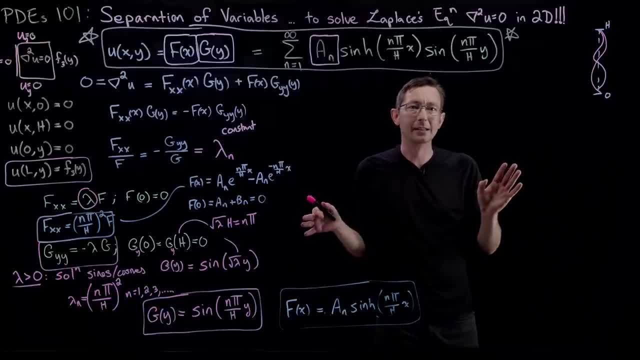 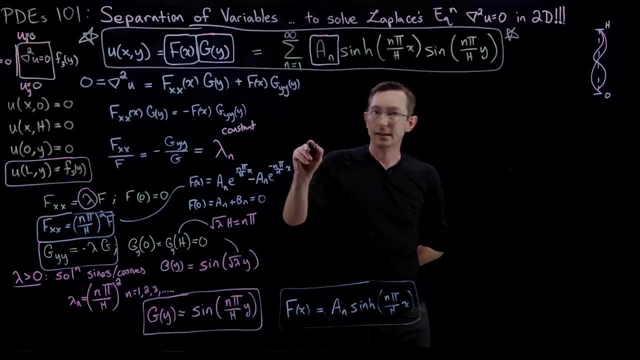 Last thing I'm going to do now. So this is kind of where the video ends, except we don't have these a n's. So the last thing I'm going to do is actually derive these a n's And we're going to use our boundary condition, which is- and I hope I have room, this is kind of a mess- is that u at my right boundary condition, u at x, equals l of y, equals this f of y boundary condition. 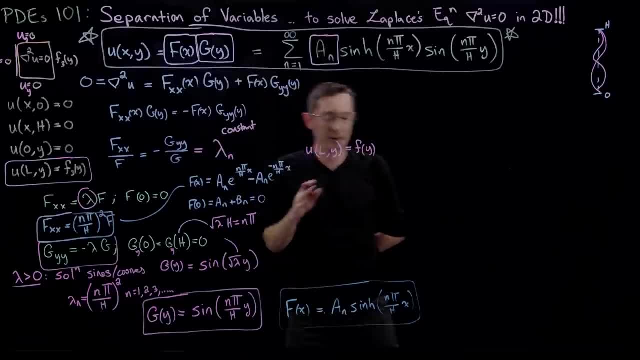 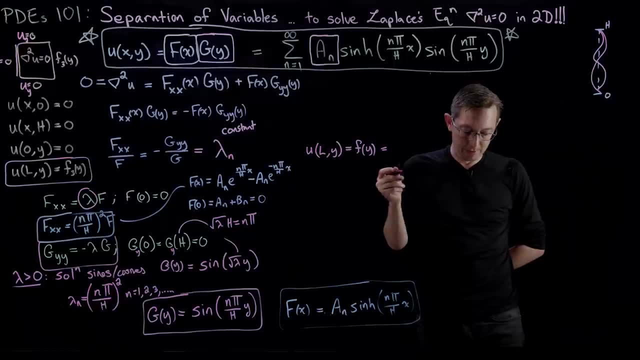 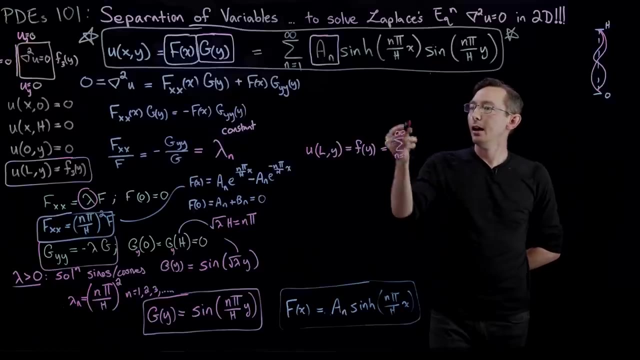 I'm going to drop the subscript 3, because I can't bear to write down subscript 3 every time I have a y here And that equals this summation up here. So it equals my sum From n. I know everyone hates it when it squeaks, I'm sorry. n equals 0 to 1 of an goodness gracious, an sinh of, and now all I'm going to do is, anytime I see an x, I'm going to replace it with an l. 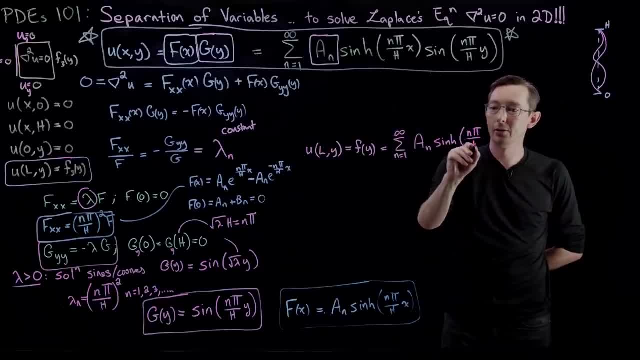 It's that simple. So I have n pi over h times l. This is a number That's actually easier. Plugging in x, x equals l, made this easier. This is just a number Times sin of n pi over hy. 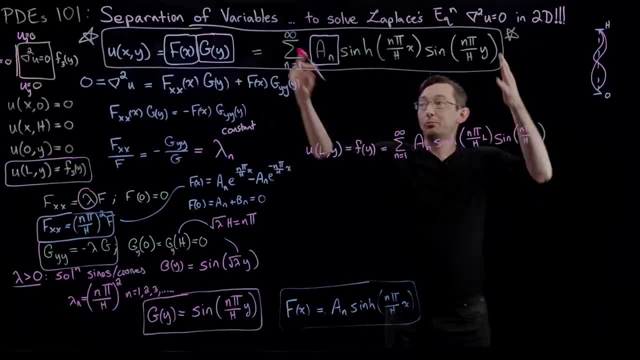 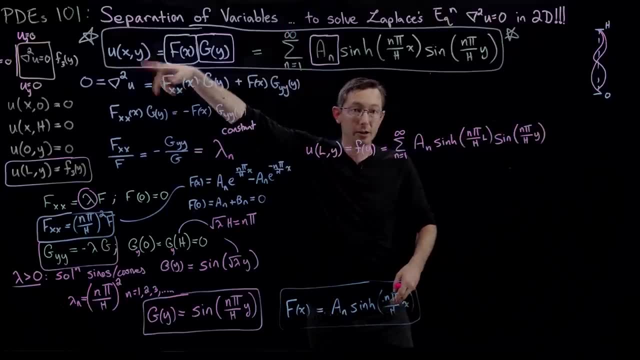 Okay, good, This is just all I've done is I've just recapitulated my solution and I've plugged in x equals l And I've said: all of this stuff in my solution has to equal my right boundary condition at x equals l. 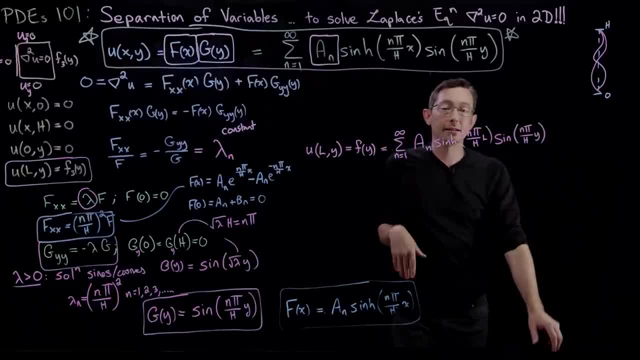 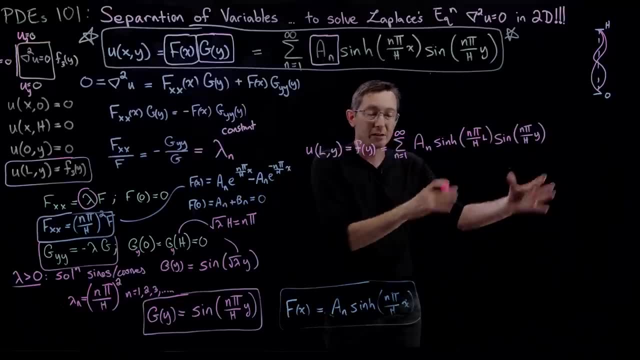 It's that simple. And now this is where the Fourier analysis comes in. And it drives me crazy that you know, when I was going to school, Fourier analysis Was its own semester class And everyone thought it would be really cool to learn Fourier analysis because it sounded, you know, neat. 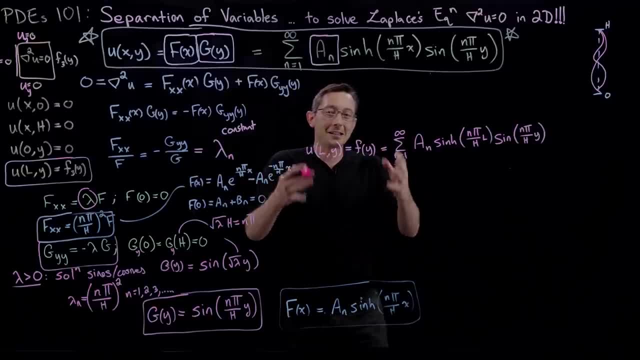 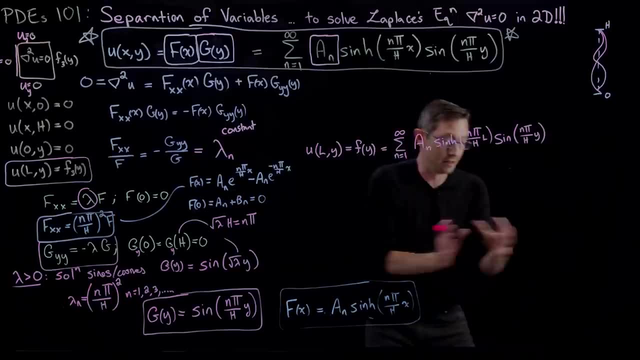 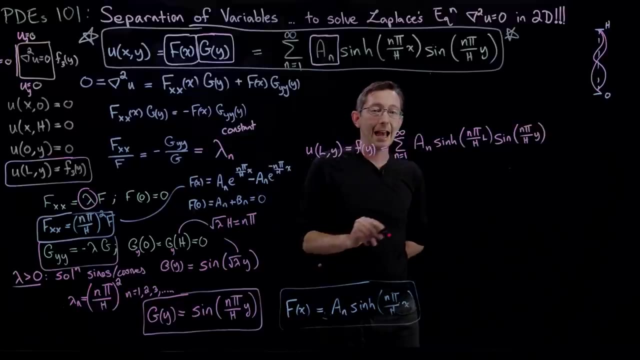 Fourier analysis in isolation is boring. Fourier analysis is a tool to solve partial differential equations and physics equations And I think it's a crime to you know separate it and quarantine it off from differential equations. But the way we're going to figure out these a n's is what we're now going to do, is we are going to. 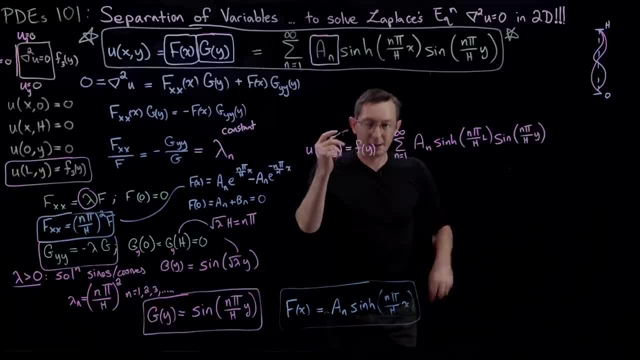 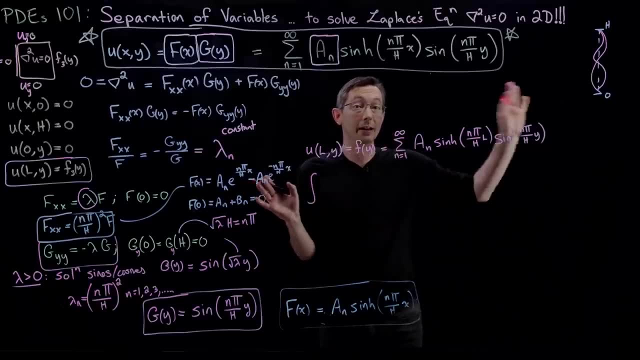 I'm just going to write this out. So I'm going to write out the essentially the inner product of this function y. So the inner product. And if you don't remember what an inner product is in a Hilbert space, a function space, 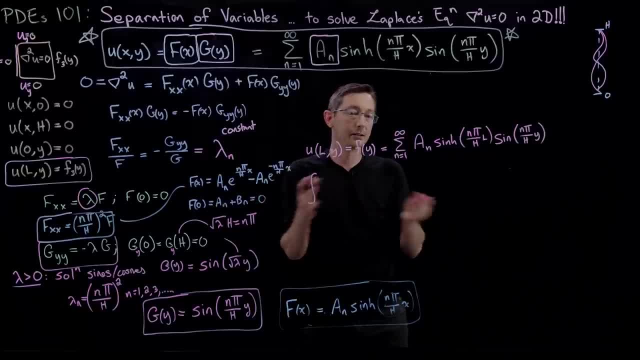 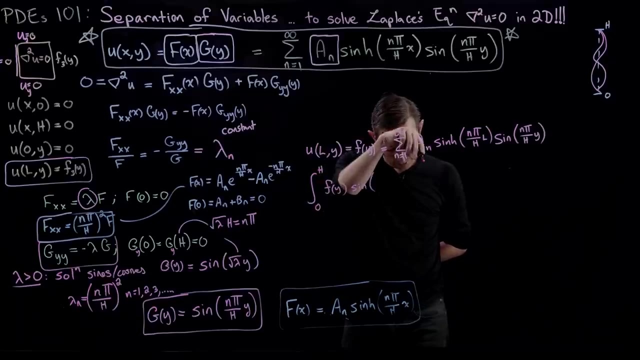 I'll put a link to the video in my Fourier analysis series where I talk all about this. It's actually really easy. It's the integral from zero to h of f of y times. my sin n. Goodness, gracious, N or m. 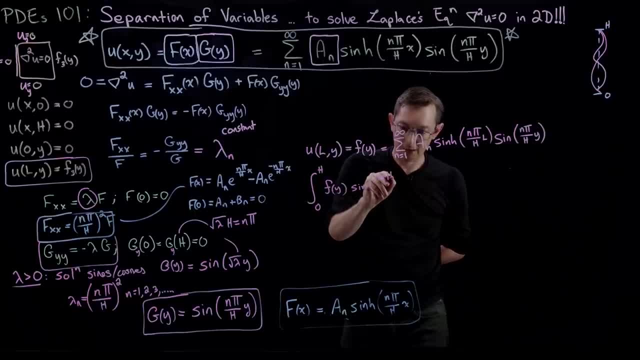 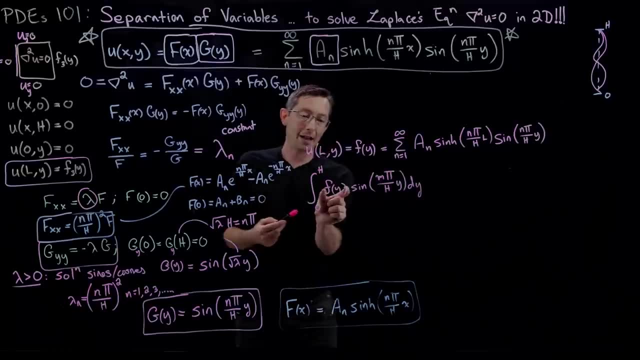 I'm going to use another variable: m, h, n, pi over h y, dy. This is literally just breaking f of y into Fourier coefficients. Okay, This is like the projection of f onto the mth Fourier coefficient. So this is the mth Fourier coefficient of this data: f y. 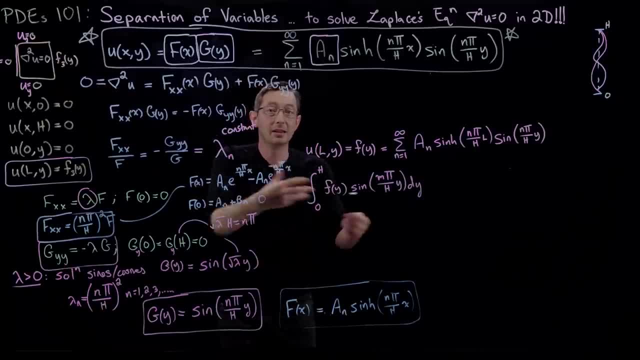 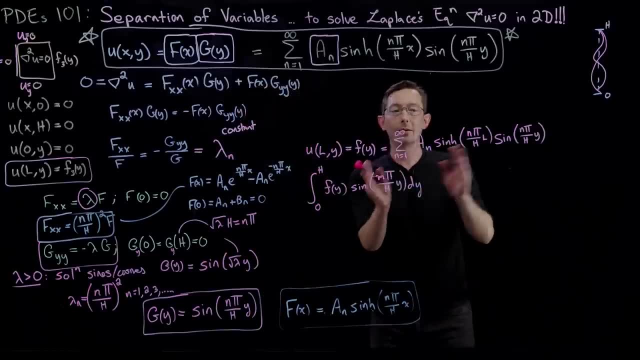 I think of this as data, because this is just a function that someone gives me, Someone specifies, And I get to use it, And so I'm going to. I'm going to compute its Fourier transform and get its Fourier transform coefficients, But now I'm going to plug in all of this nonsense into that f of y. 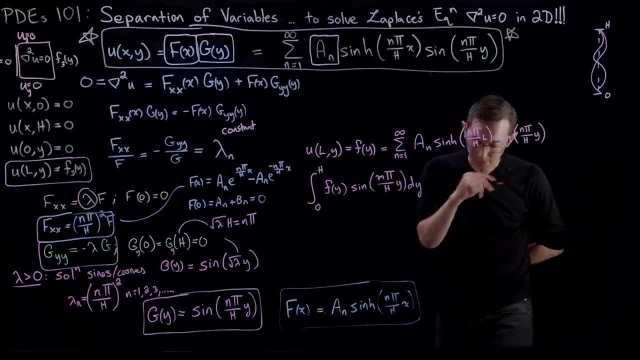 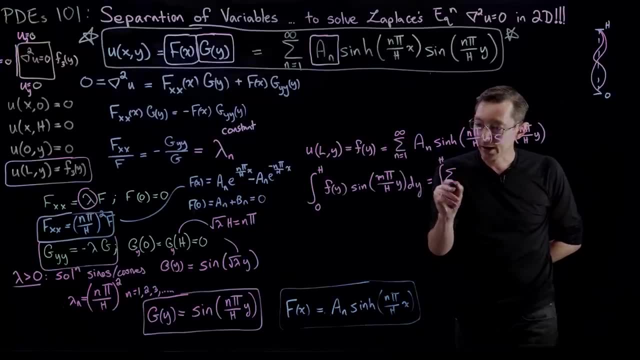 And I'm going to get something nasty, But things are going to cancel out. Okay, So this equals integral. I'm trying to make this not squeak Zero to h of my god awful sum of a n sinch, Which is just a number. 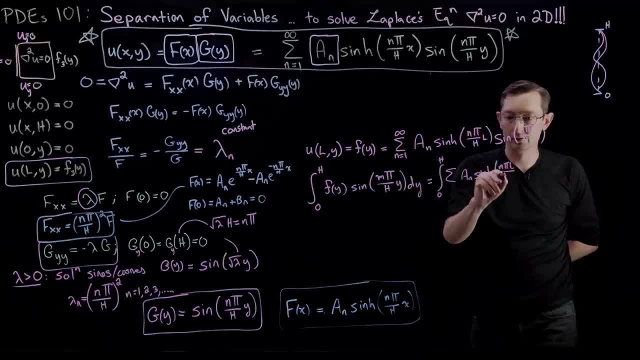 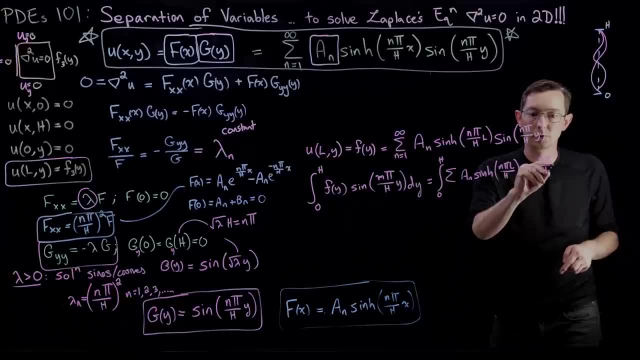 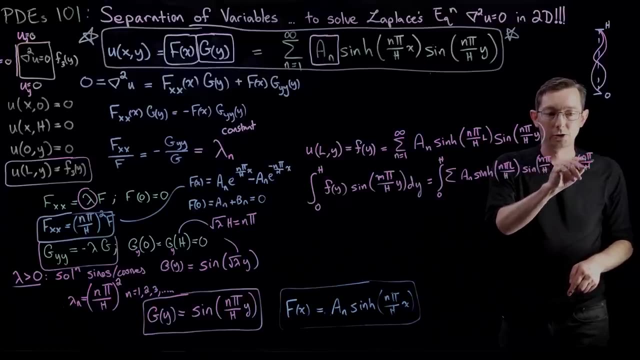 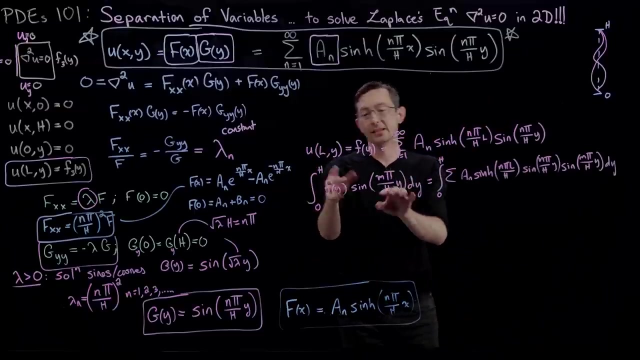 Sinch n? pi l over h? Just a number Times this sin Sin n? pi over h? y Times this sin Sin m? pi over h? y dy. Now, literally, I just took. This is the Fourier transform of f? y. This is one of the terms of the Fourier transform of f? y. 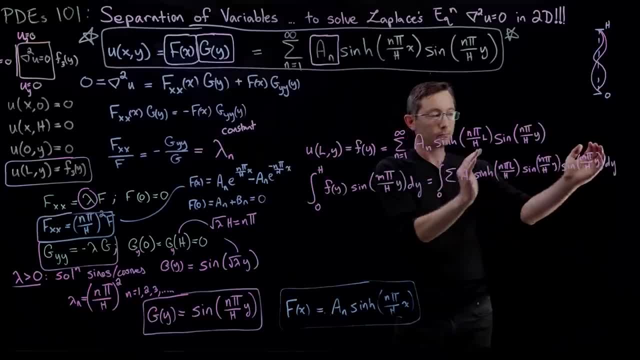 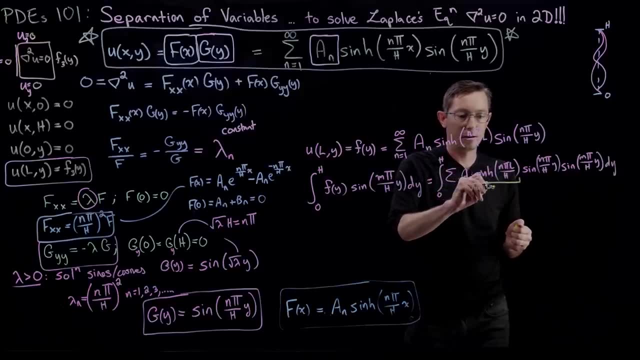 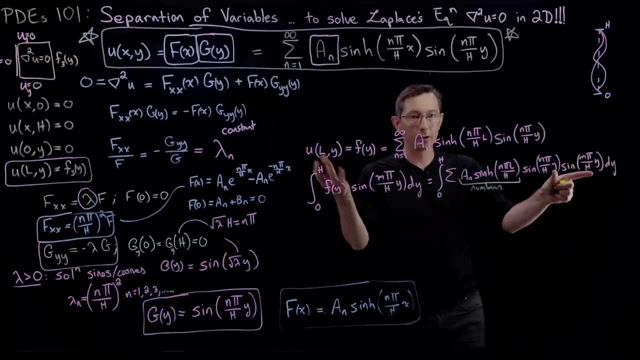 And I plugged in this expression of f? y, My solution And what you'll notice now. You know these are just numbers, These are numbers And this inner product Can, only This integral from zero to h. This is something you'll learn in Fourier analysis. 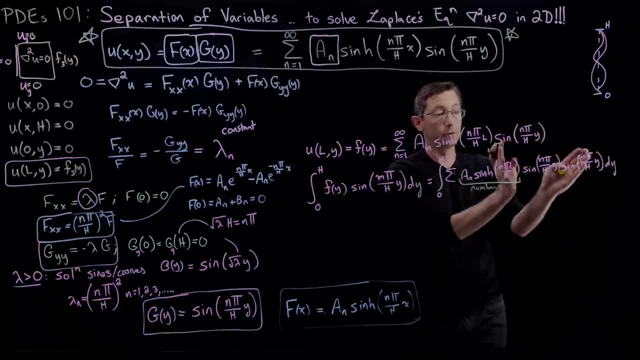 I call this an inner product between these two functions. These are orthogonal functions. If n is not equal to m For any non-integer n and m For any integer n and m that don't equal each other, This integral is zero. 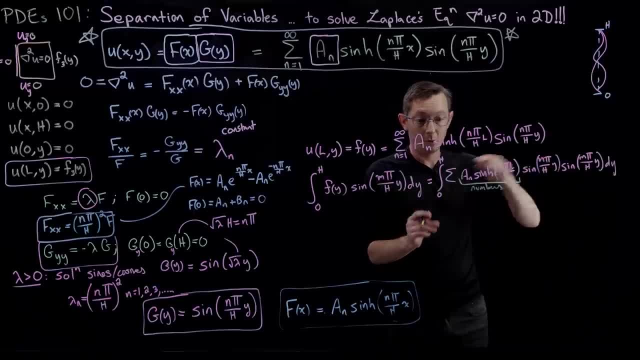 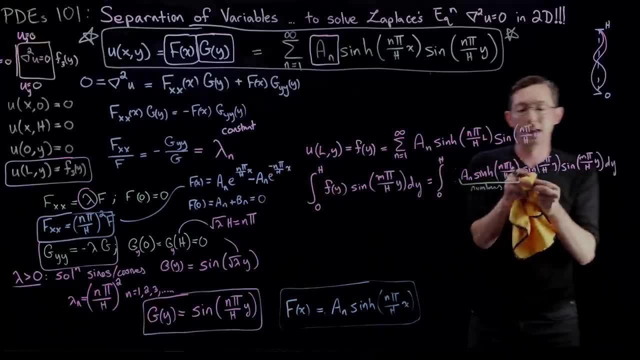 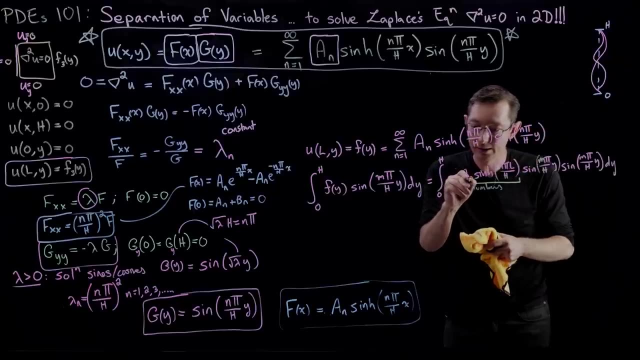 So this is only non-zero when n equals m, Which means we can drop this, We can drop this summation here, And this n has to equal m, Okay, And this n has to equal m, And all of these n's have to equal m's. 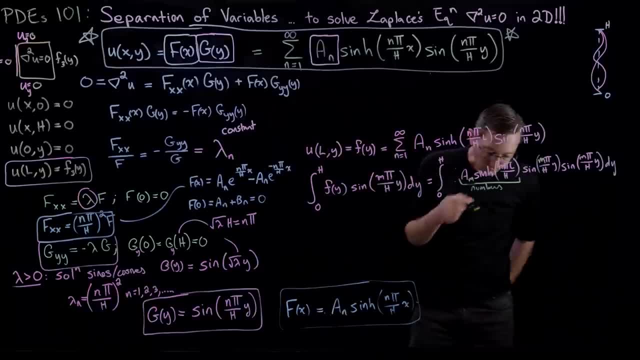 And I can probably just make my n's m's without erasing them, And so essentially what we get Is that this equals a, m a m. This integral From zero to h Will have A length scale h. Again, this is just details over two. 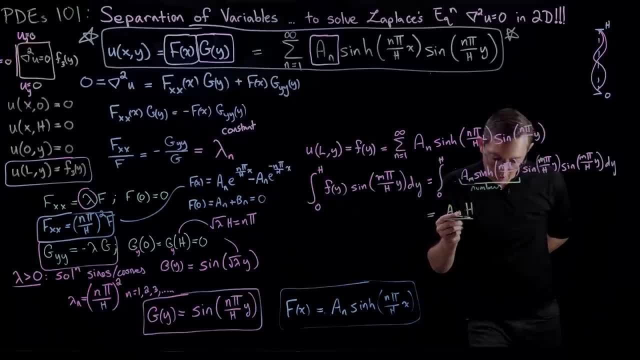 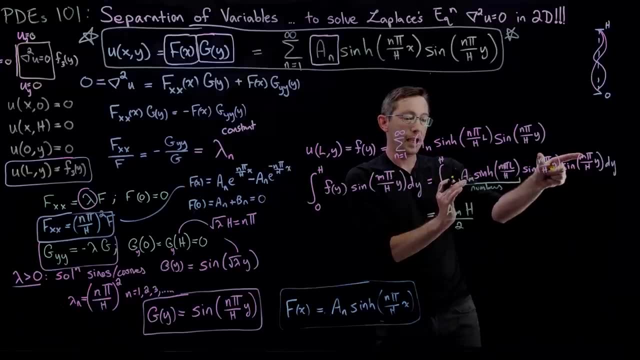 This is just from this integral. I'm just showing you what the integral is. So the integral- Forget all this junk, This is a constant. This pops out. The integral of these two things, When n equals m, Is just one half. 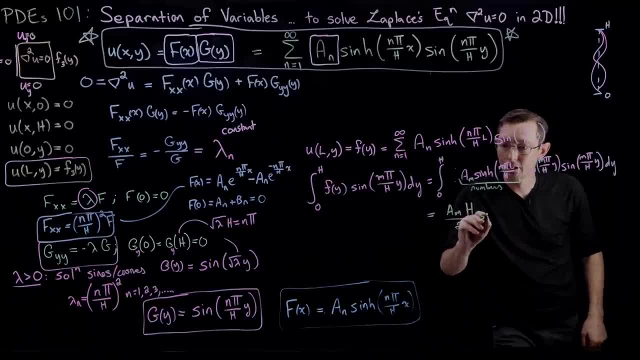 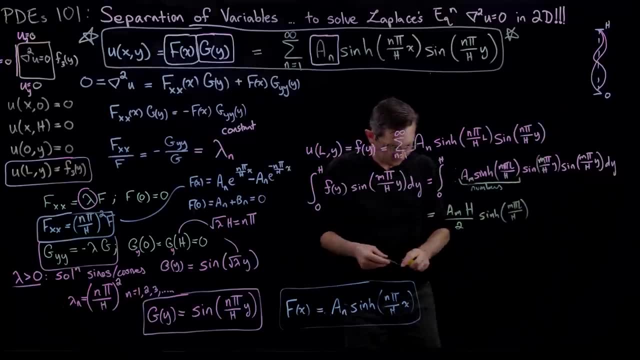 Times h. It's h over two, So I get h over two a m Cinch m pi l over h. Good, And so This is What this integral equals: Okay, Ha, Which means I can solve for a m. 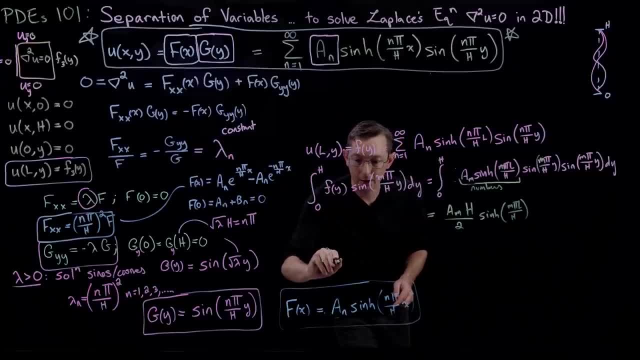 So now a m- And I'll just call it a m Equals This thing here Equals Two Over H. Cinch M pi l over h Moved all this over here. Times the integral From zero to h. 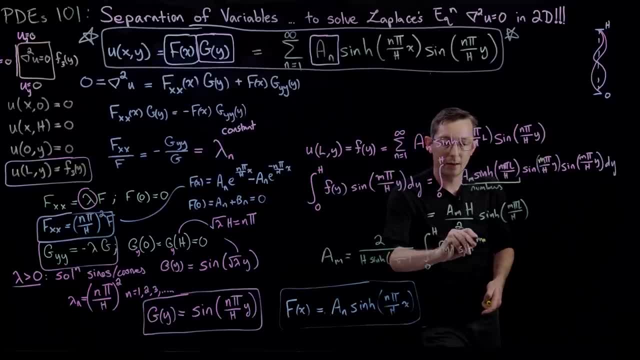 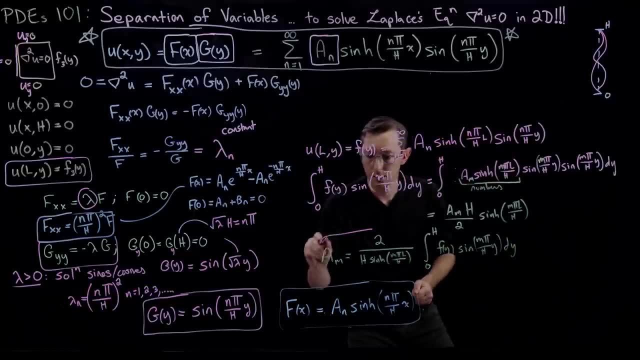 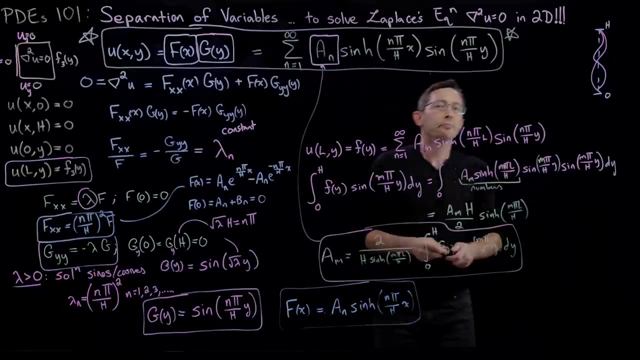 Of f, of y, Sine, M, pi, over h, Y, D, y. This here, And let's just confirm This here, Is this coefficient. So This is a number, Number Number. This is a function Of specified numbers. 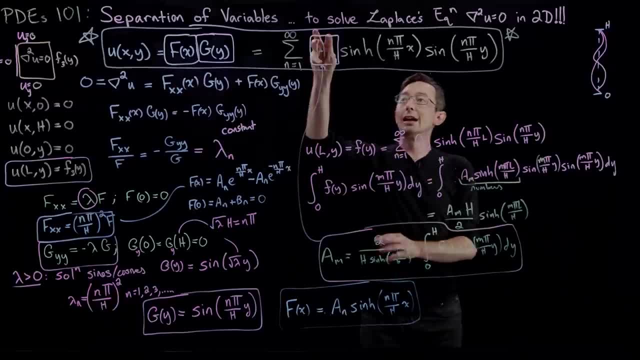 And this is data. This is my boundary condition F of y, So I can determine these A coefficients Purely From taking the Fourier transform. It's essentially just some constant times, The Fourier transform coefficients Of my data On my right boundary condition. 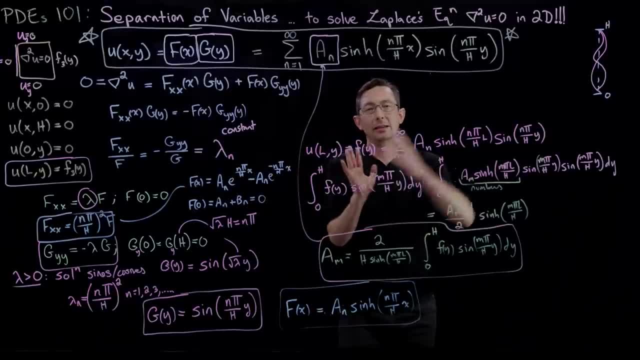 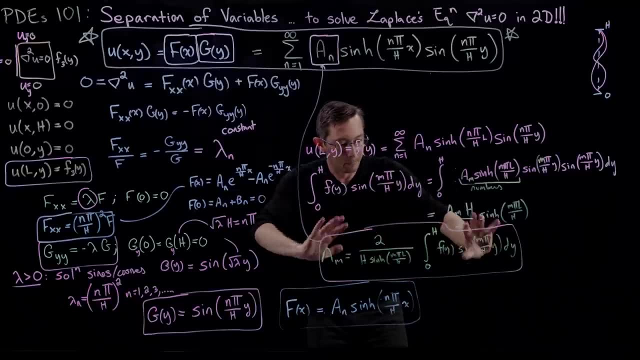 So that's how you get these a? n, Which I think is kind of cool. I know this made the video about 10 minutes extra long And some of you have fallen asleep, So you're welcome if it's late at night, But I think it's really cool.